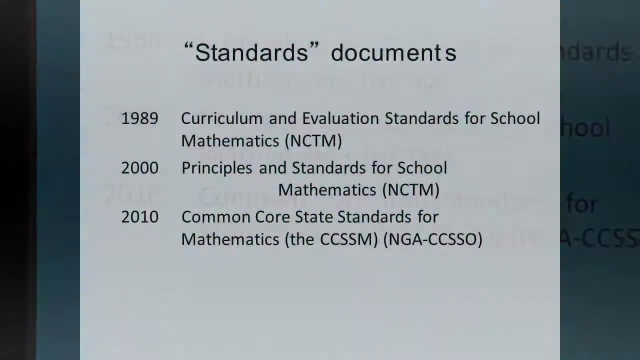 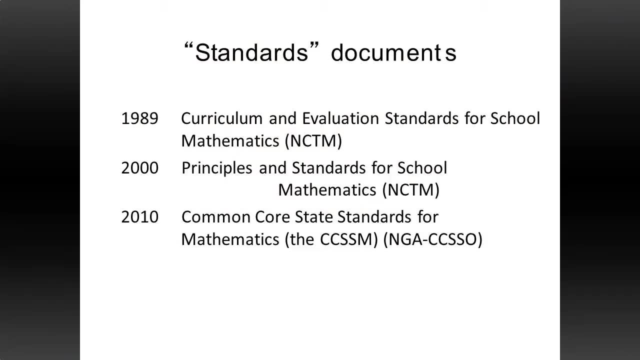 State School Officers. The mathematics standards, the CCSSM Common Core State Standards for Mathematics, are different from the NCTM standards of 1989 and the Principles and Standards for School Mathematics of 2000.. Those documents indicated directions To which mathematics educators wanted schools to move, and the directions were given in. 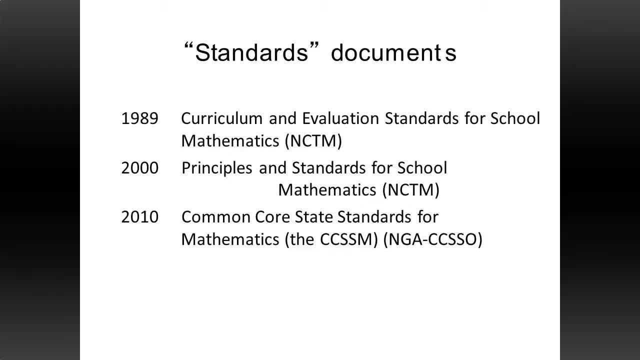 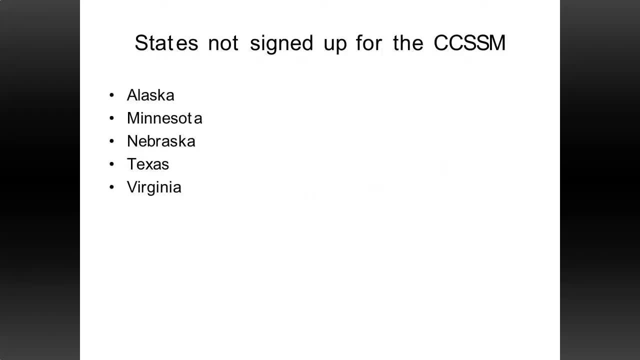 grade level: bands K-2,, 3,, 5,, 6,, 8,, 9, 12.. Two carrots were dangled by the federal government to get states to sign up to follow the Common Core standards. The first carrot was the race. 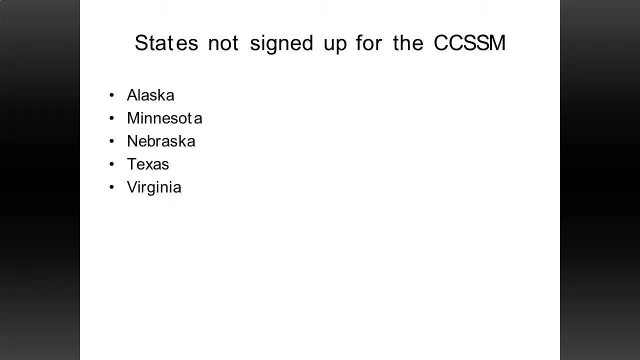 to the top. federal funds were only available to states that signed up. The second carrot was the federal money was given to fund through testing agencies, So a state would not have to create its own assessments for language arts and mathematics. So ostensibly the Common. 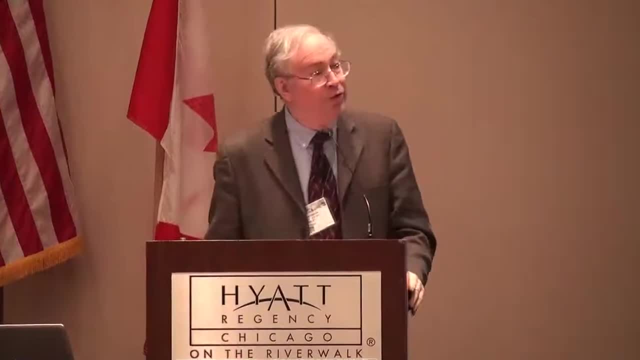 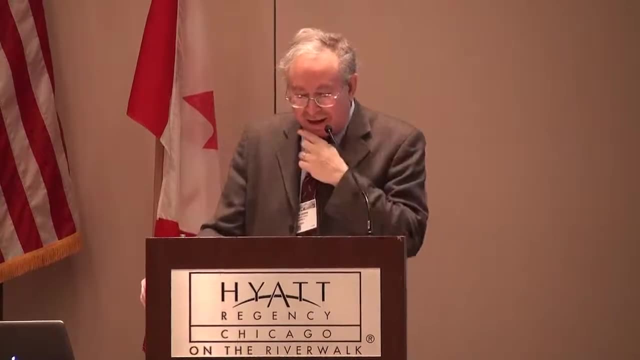 Core process would save states money. As a result, 45 states and the District of Columbia have signed up to follow the Common Core standards. Only five states- the ones here- have decided not to align their standards with one of these two agencies. The Common Core standards could. 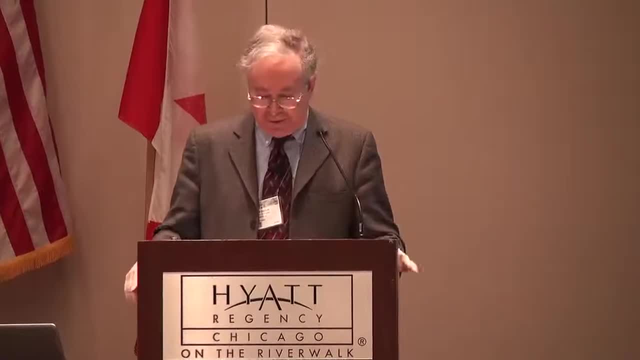 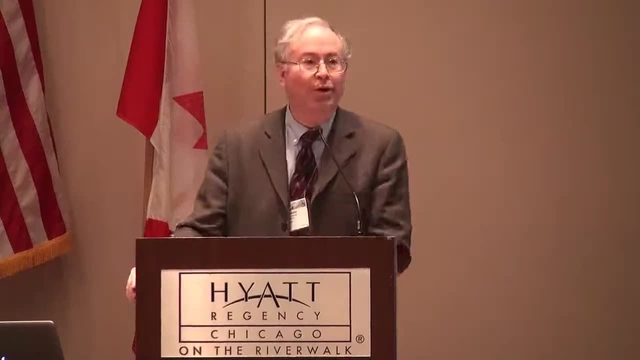 be relatively ignored by schools and teachers, were it not for their purpose, which is to provide a framework for the testing of all students in grades 3 through 8, and in high school, each year beginning in the school year 2014-15. And in a growing number of. 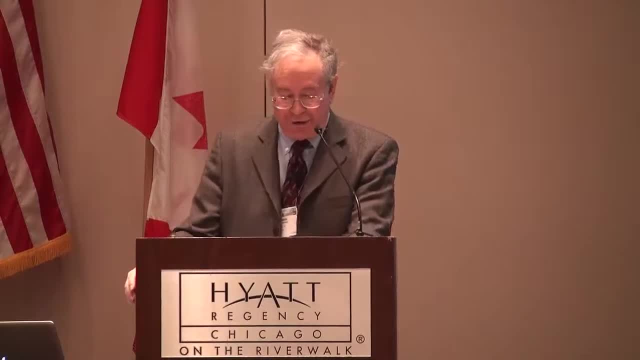 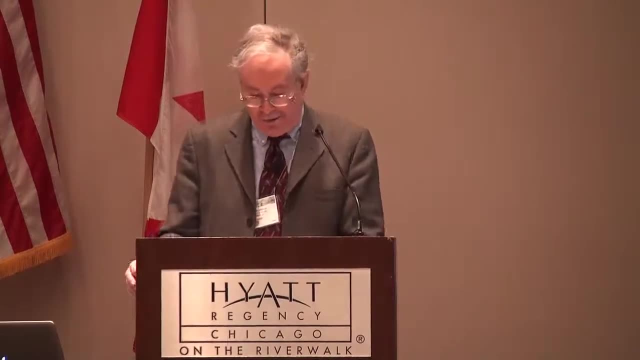 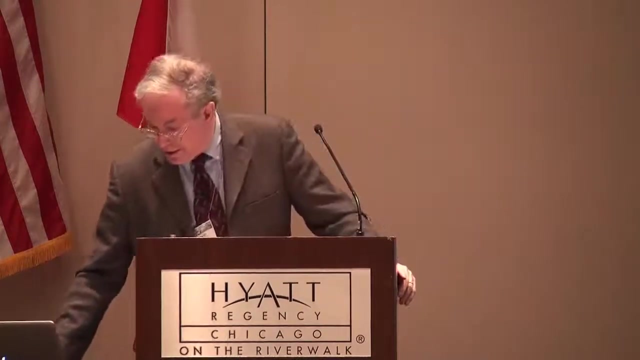 states. teachers are going to be judged by how their students perform on these tests. So the Common Core standards are big stuff, important for everyone to know, And so everyone should know what is in them. In the Common Core state standards there are 385 content. 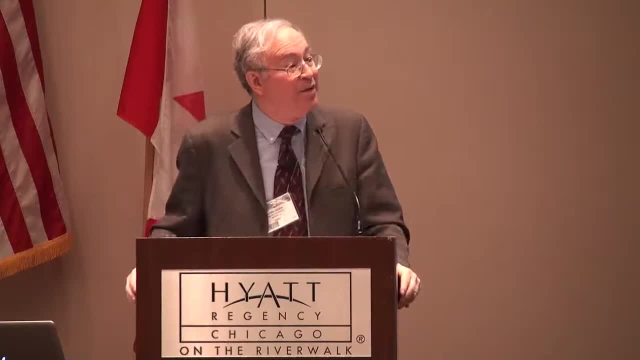 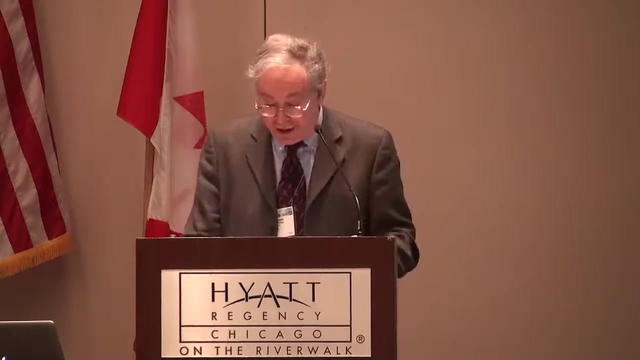 standards. They occupy 76 of the 93 pages of the original document. They are indicated by individual grade for grades K-8, and by subject areas for high school. In addition, there are eight standards for mathematical practice, Though they occupy only three pages, the standards- 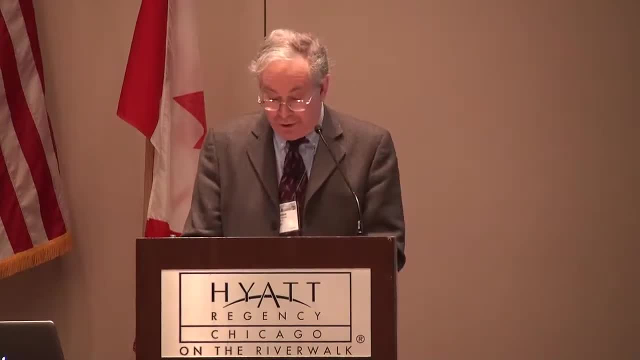 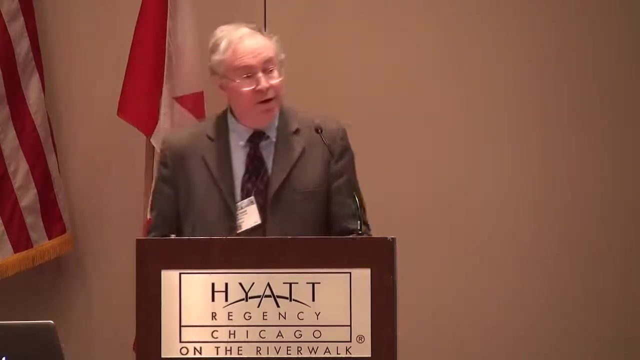 for mathematical practice are meant to be infused throughout the content standards, And many people think they are the most important standards, but also the ones most likely to be given short shrift In classrooms and in assessments. Here are the headings for the eight standards for mathematical practice. Many of you are 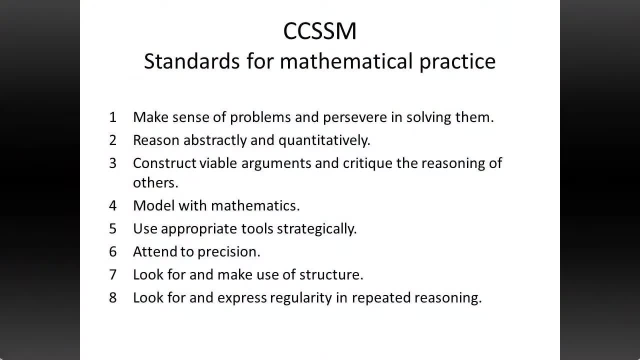 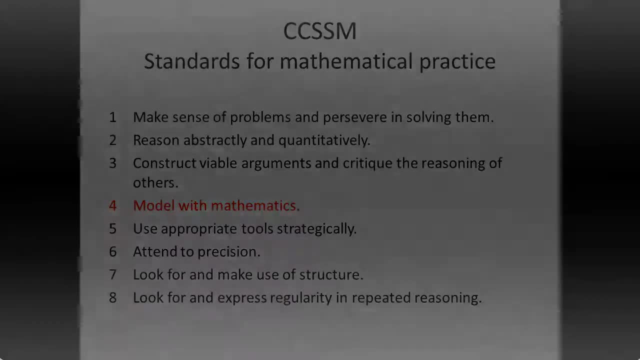 familiar with these headings. My talk today is about the fourth of these standards, The standard that deals with mathematical modeling. What does model with mathematics mean? Here's the script of the fourth standard: 4.310: All-Positive Practical Practice standards. 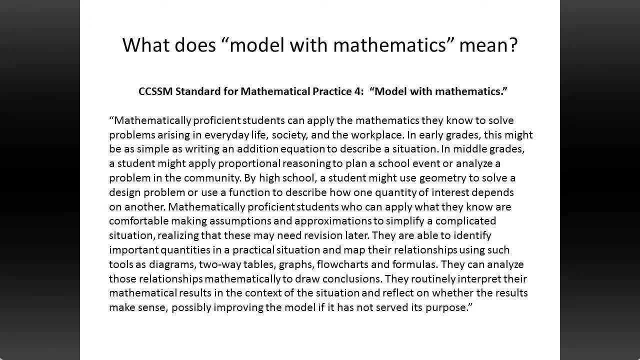 4.310: All-Positive Practical Practice standards. This is it. You'll be tested on it at the end of this session. Well, I don't know the intent of the writers of the Common Core when they wrote the standard, but I feel that it has two parts. 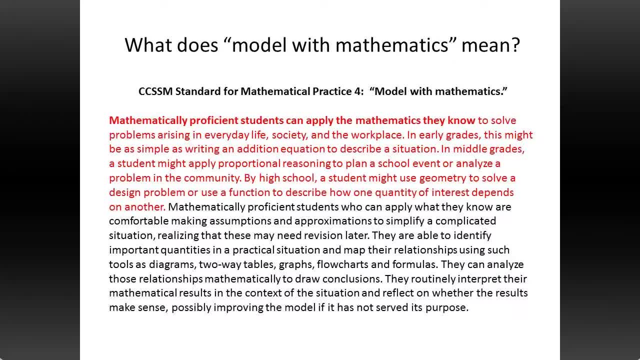 This part is described in the first sentence. Mathematically proficient students can apply the mathematics they know, And then they give three examples: One from arithmetic, one from- well, they call it- early grades, and one from the middle grades, and one in high school. 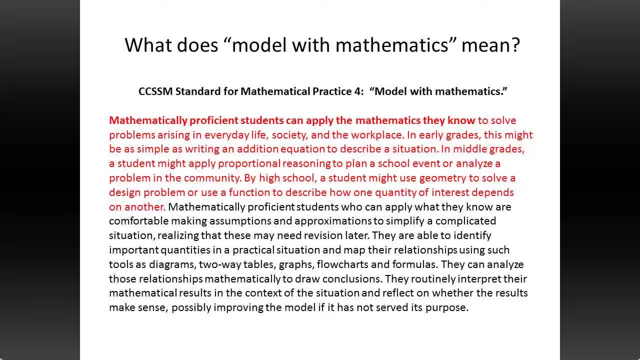 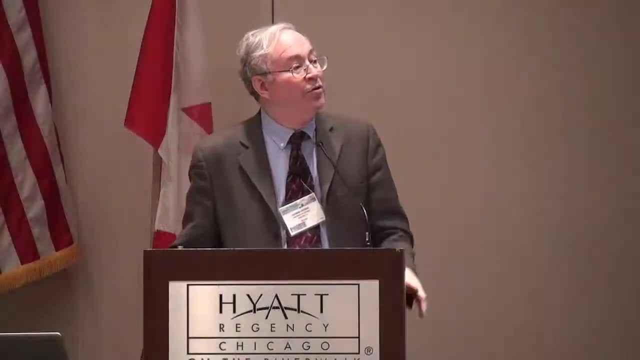 Okay, so that's the first half of it. The second half of the standard for mathematical practice is about mathematical modeling, But before discussing it, I would like to give one of my favorite examples of mathematical modeling. I've used this example before in order to describe 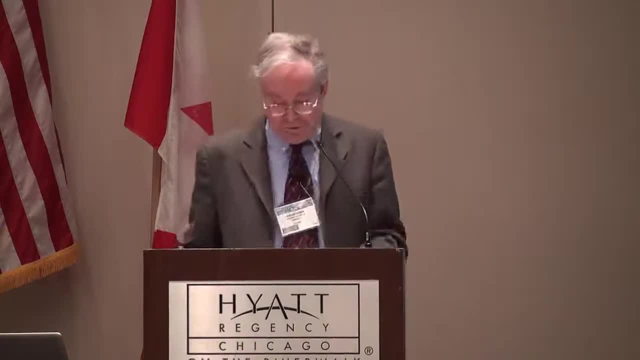 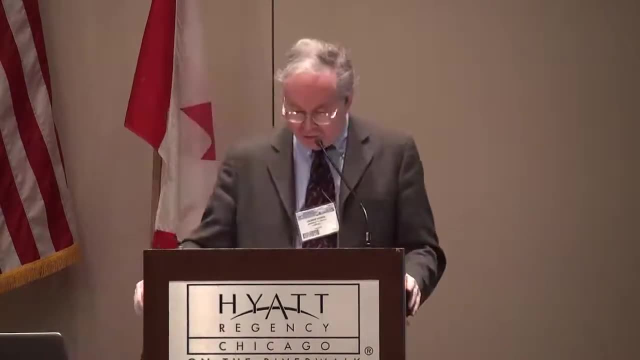 some things in some talks, so I apologize to those of you who've heard this story before, but it's so good I want to repeat it. It's called Mitchell's Golf Problem. It's a true story named after my first cousin, Mitchell. 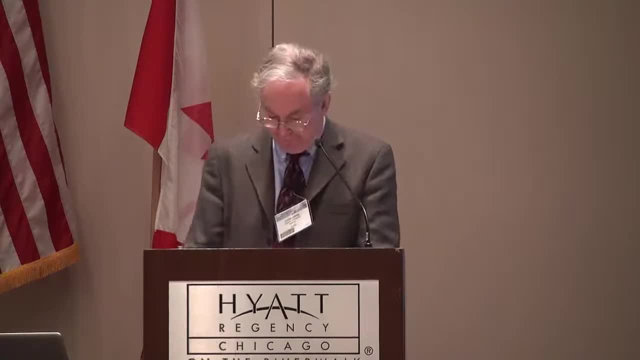 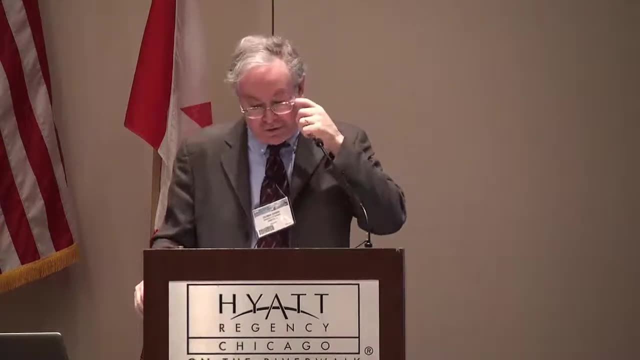 who posed it to me on May 15, 1970.. In the afternoon of that day I'd learned that my mother died. At the time I was in my first year in the faculty at the University of Chicago and living on the far south side of Chicago. 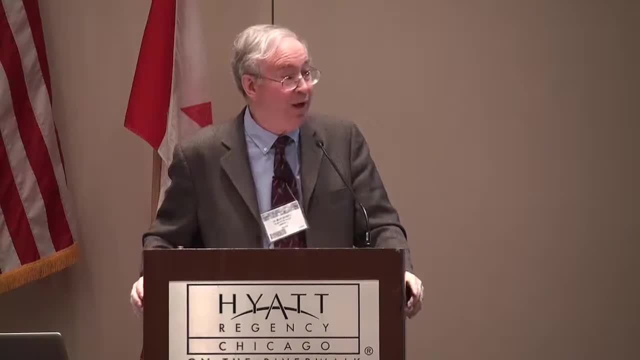 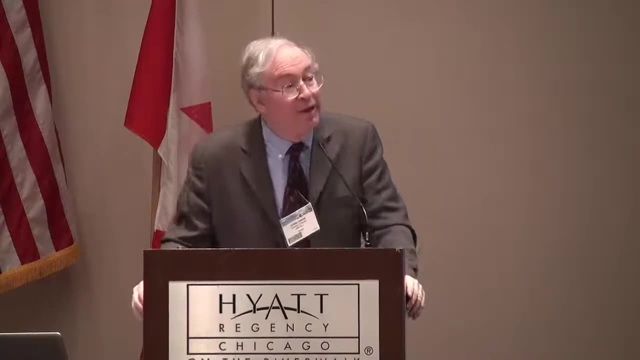 My parents lived on the north side, about 45 minutes away. We're native Chicagoans. As soon as I learned of her sudden death, I informed my colleagues I wouldn't be around for a week. They said they would cover my classes. 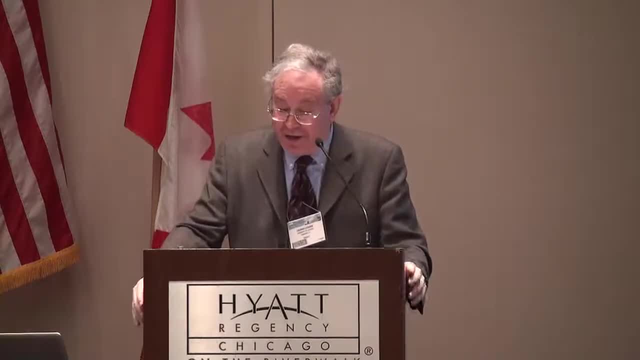 and I went to my apartment to get some changes of clothing because I knew I'd be staying the entire next week with my father and it wasn't clear what I was going to do. but I was going to be there for the next week. 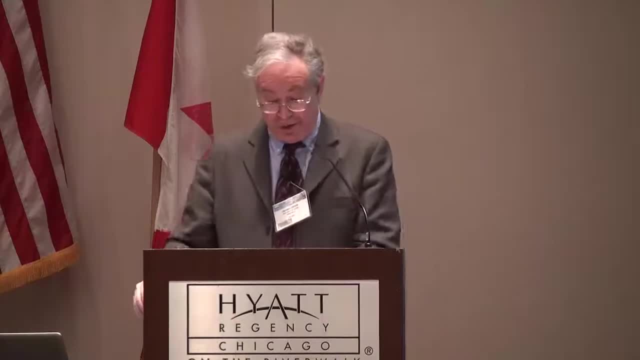 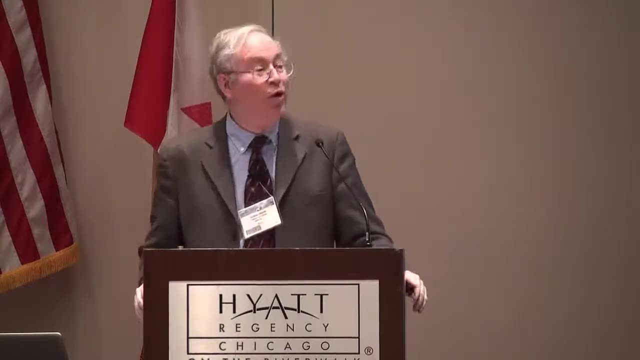 And that evening Mitchell came over with other close relatives to console us. He knew that I would not have that much to do for the week and it would be good to take my mind off the loss, and so he told me his problem. 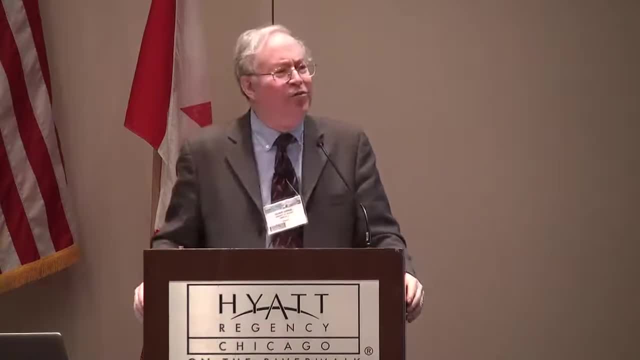 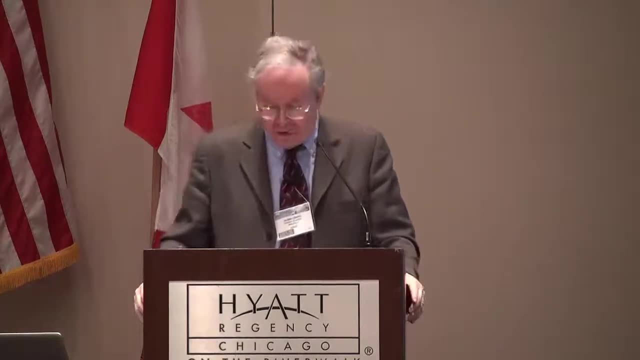 He said I golf with a group of 40 men every Saturday. We go off in foursomes. The first four guys show up, go out first, Then the next four, and so on. The problem is that the same guys tend to come early every week. 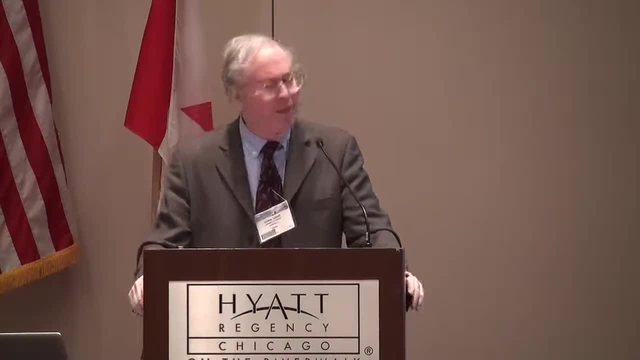 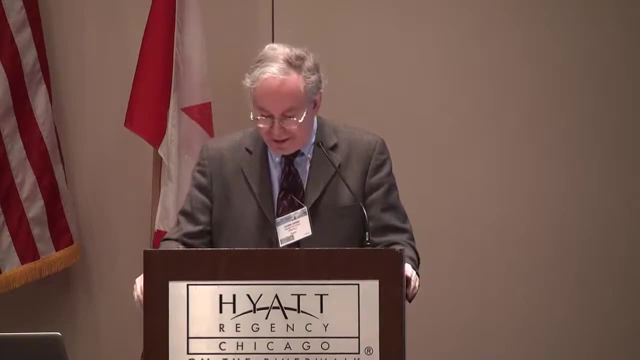 and the same guys tend to come late. People are complaining that they're always golfing with the same people and never get to golf with most of the others. I'm secretary of the group and they asked me to form a schedule whereby every man would be in a foursome. 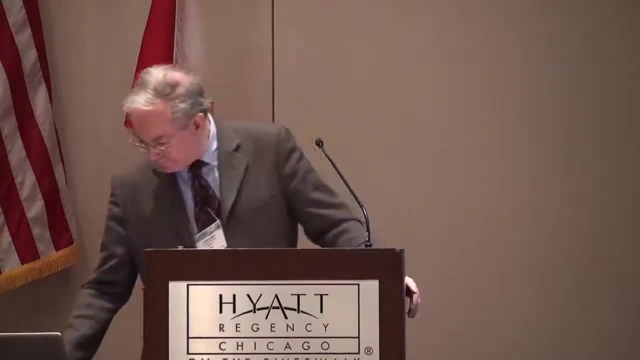 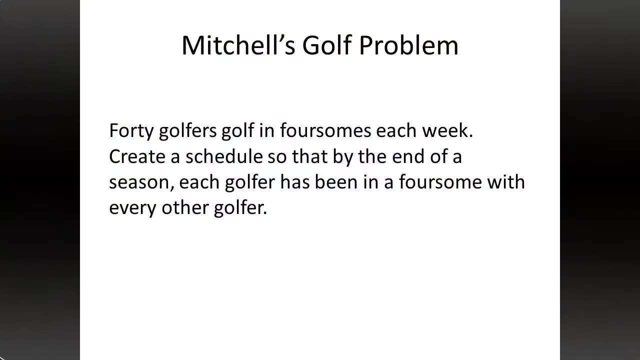 with every other person by the end of the summer. So here's the problem. Mitchell is no dummy. He went on. I tried to figure this out, but every process I tried wound up collapsing after a few weeks, well before guys had played with everyone. 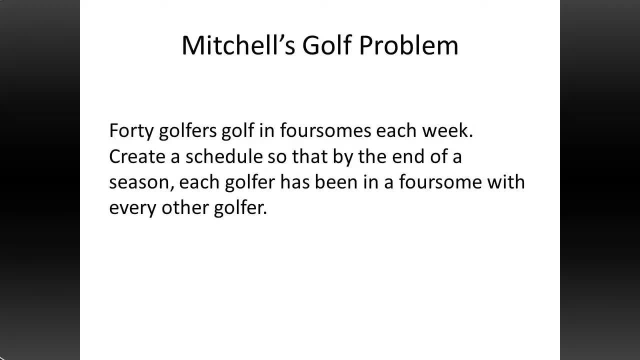 I immediately. I immediately responded that this problem was right up my alley and I would try for a solution in 13 weeks, the minimum. Mitchell said he didn't need such an optimal solution because there were many more weeks than 13 in the summer. 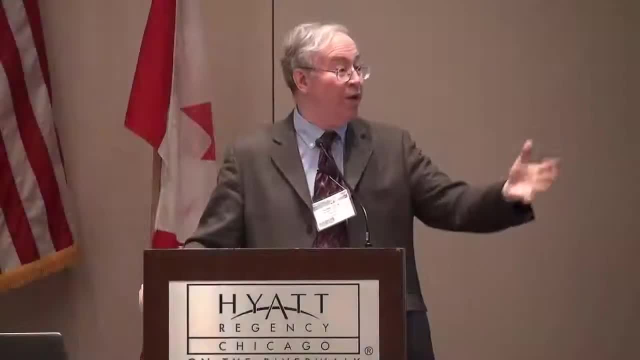 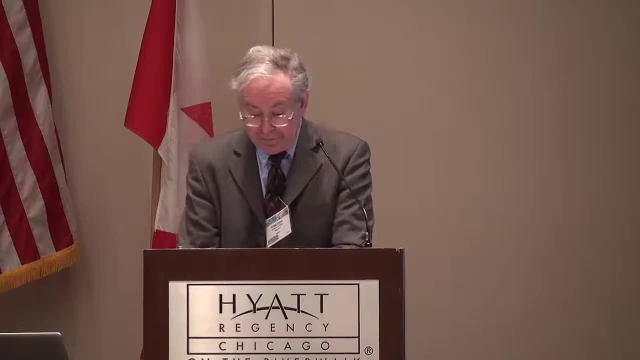 and if I just had a solution that could be done in 19 weeks or 20 weeks, where everybody could play with everybody else, that'd be good enough- Not for me. And so as soon as I had some free time, I went at the problem. 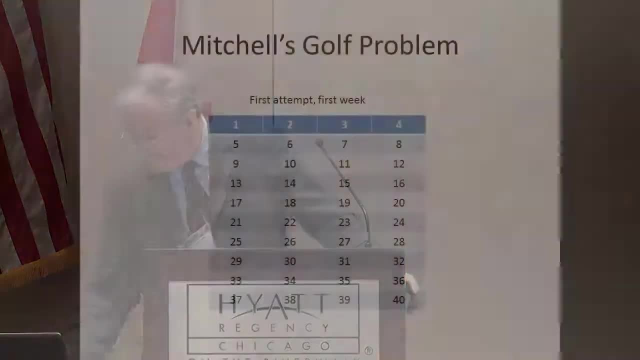 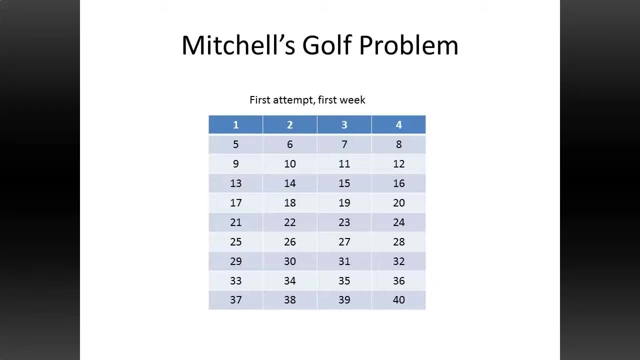 I put down the numbers from 1 to 40 in four columns. Here were my foursomes for the first week: 1 to 4,, 5 to 8,, 9 to 12, and so on. They're my foursomes. 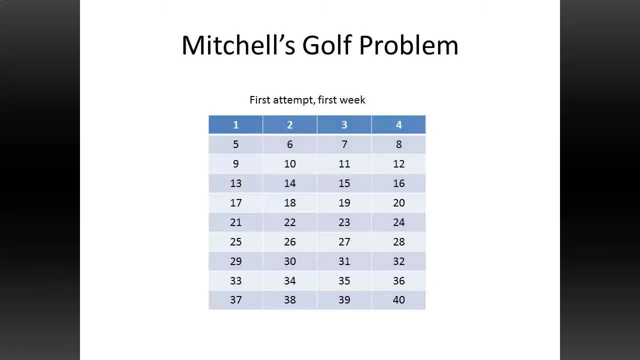 Now, what should I do for the second week? Well, perhaps go down the columns. So foursomes for the second week became 1,, 5,, 9,, 13.. That was the first foursome. 17,, 21,, 25,, 29 became the second foursome. 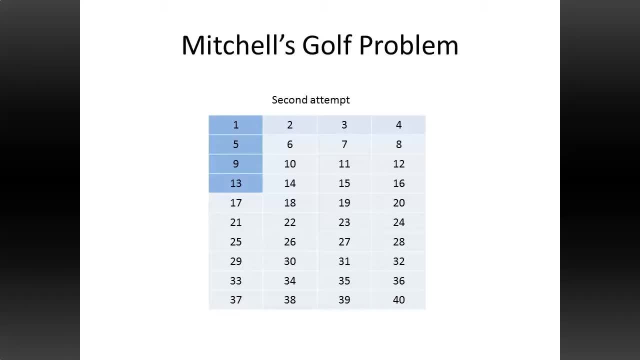 33,, 37, I went up to the column 2, 6 became the third one. This worked for a few weeks. I kept getting different foursomes. Then it started giving me people playing with each other twice even in just a few weeks. 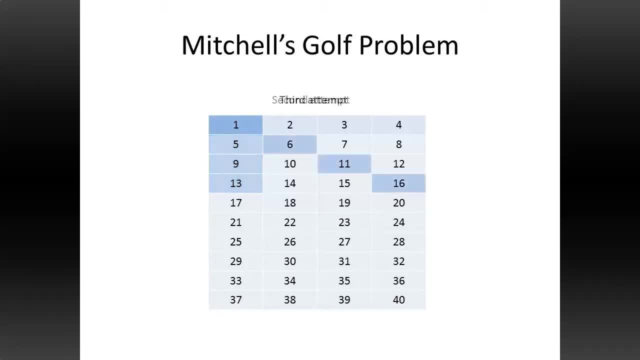 Maybe go diagonal: 1,, 6,, 11,, 16.. 5,, 10,, 15,, 20.. I wound up in the same place as Mitchell, a little frustrated. This was not as simple a problem as I thought. 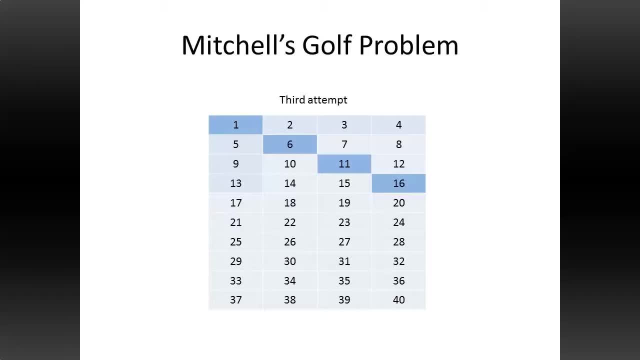 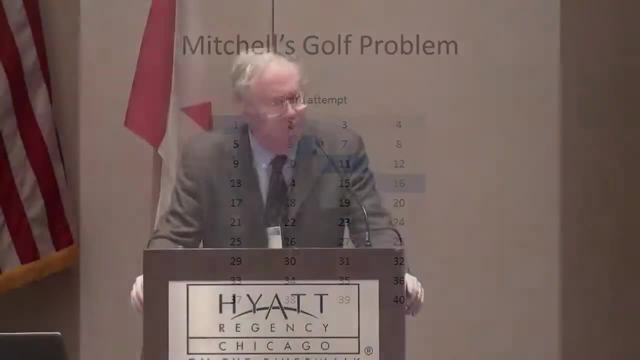 To make a long story short- and it is a long story, so I am making it short. I was unable to find a solution whereby, in 13 weeks of golf, each golfer would be in a foursome with every other one. I wasn't able to do it in 13 weeks. There are 39 other golfers, you understand. There are 40 golfers, so you're playing with three each week. so it takes 13 weeks at a minimum, But I did find a solution in 15 weeks. There's still a seat here. 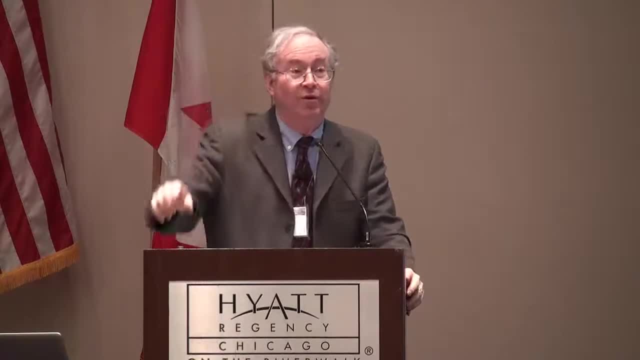 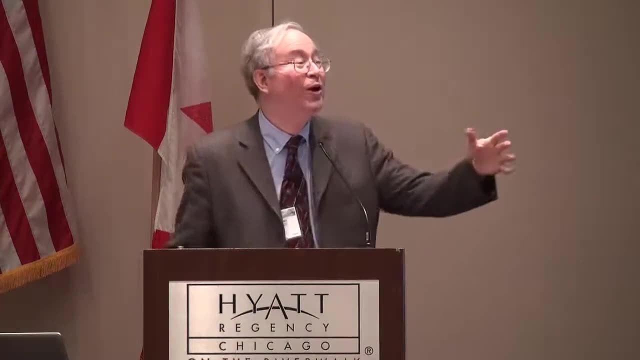 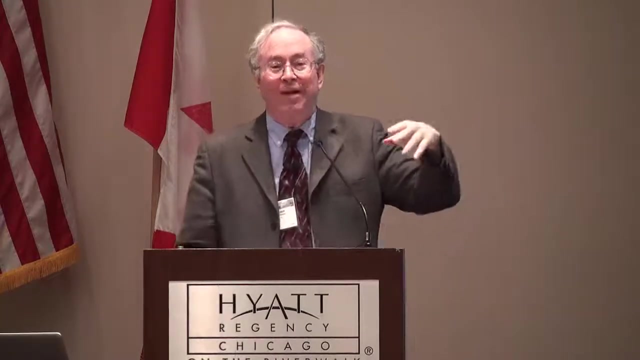 There's a special seat, Marty. it's for you. They've been saving it for you. We work together. I found a solution in 15 weeks and I mailed it to Mitchell. A short time later, I received a call from Mitchell. 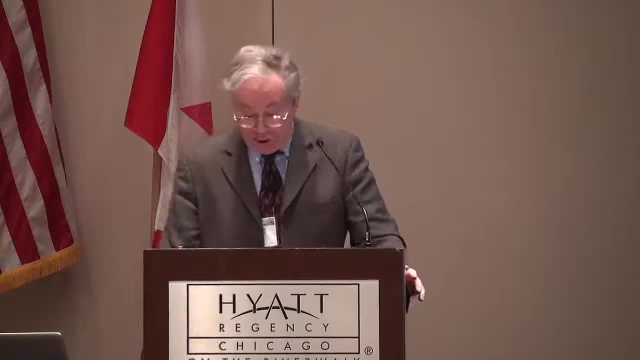 He was very happy. He had taken my solution and worked up a schedule and sent it to all the members of the golfing group and they were happy too. But he said he had to modify my solution in two ways. First, there were 41 golfers in the group, not 40.. 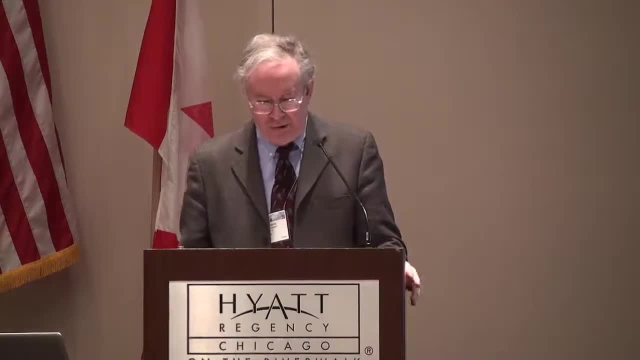 Second, there were these two men who hated each other and they would not play with each other. Mitchell said I modified the first problem by making myself the 41st player. Every week there's someone who's on vacation, who can't show up. 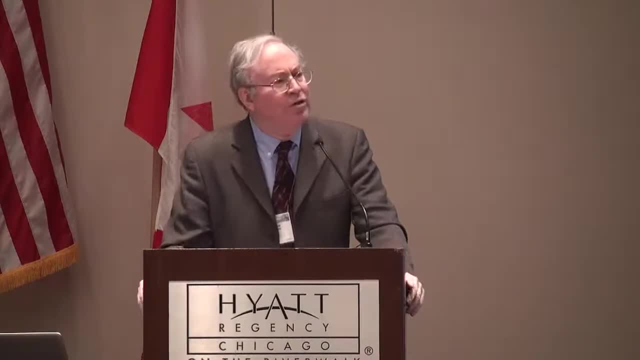 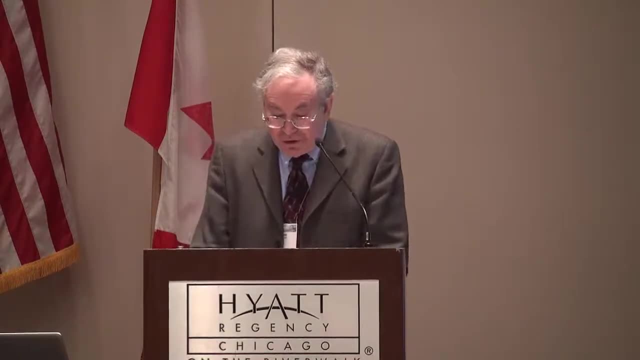 and so I'm taking their place And I switched some people so that the two guys who hate each other would never be in the same foursome. Mitchell's golf problem exemplifies the modeling process. Modeling starts with a real problem. The first step in the process is simplifying the problem. 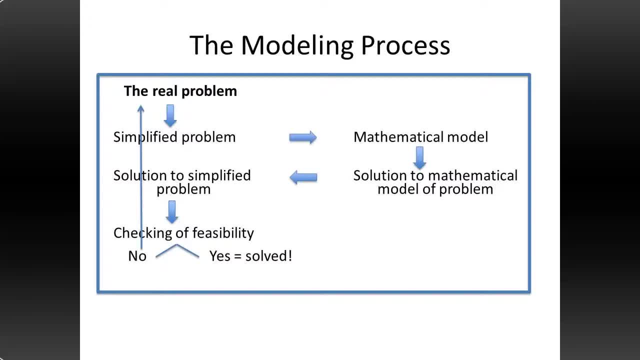 Which Mitchell did by converting 41 to 40. And ignoring the fact that two men would not play together. Now I've indicated the steps by arrows. The next step is translating the simplified problem into mathematics, That is, finding a mathematical model. 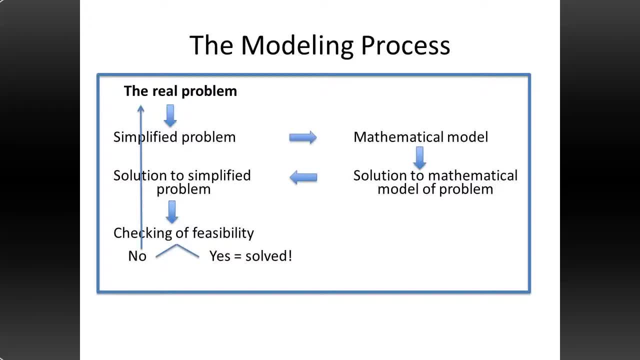 The third step is to work with the mathematics. In this case the mathematics it turns out of block design, These arrays in blocks. Then, once a solution has been found to the mathematical problem, there's the step of translating the solution back to the original situation. 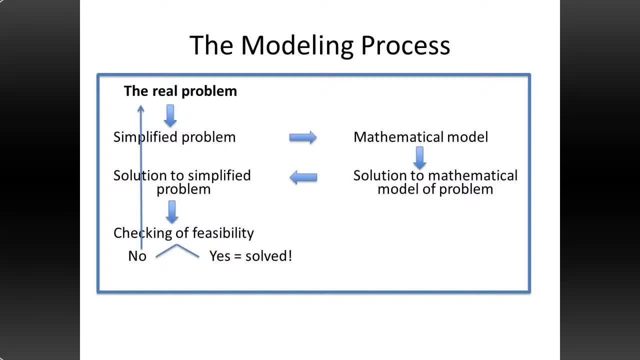 And then asking whether the solution is feasible. In advance, Mitchell knew that my solution would not be feasible, So there was no way to get everyone playing with each other in 19 and 20 weeks. that didn't have these people, You know. he knew. he didn't tell me about it, so he knew it wouldn't be feasible. 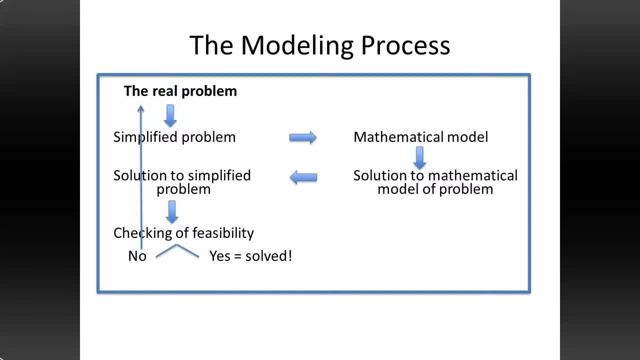 If there had been no feasible solution, there would have been no way to get everyone playing with each other. even in 19 or 20 weeks We might have to go back to the beginning of the problem and say it's not solvable. 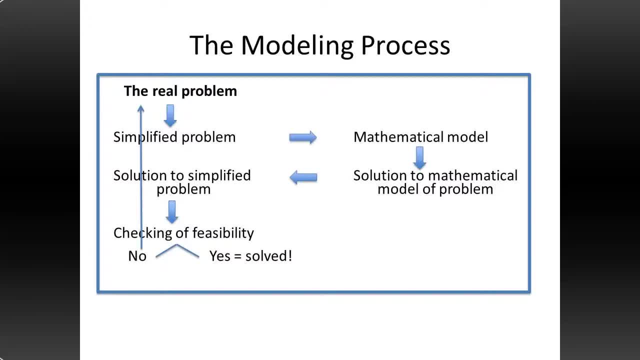 Maybe we'll have to do it in two summers rather than one summer To change the problem. Some people would say that my diagram focuses not on the process but on the results of the process. Would prefer an emphasis on the actions, So this next slide emphasizes the actions. 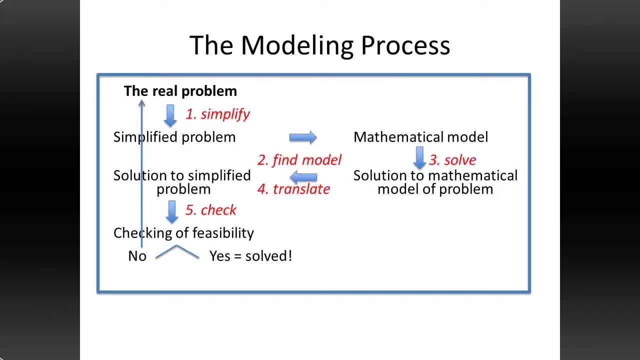 Simplify, find a model, solve, translate, check. The mathematical modeling of Mitchell's problem began as soon as I denoted the golfers by the numbers 1 through 40. This enabled me to apply mathematical operations to obtain the needed foursomes. 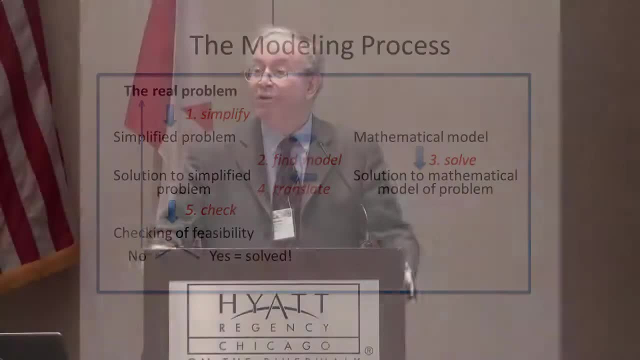 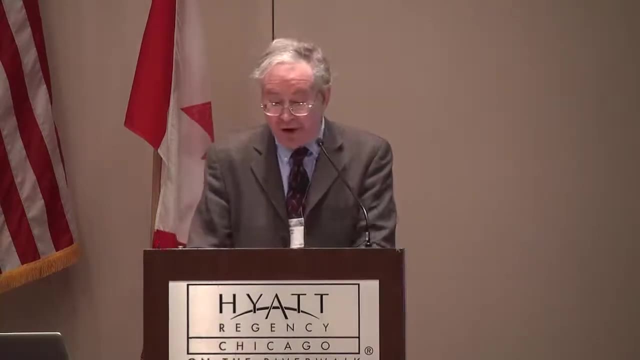 Even this step, which was so obvious to me- it was the first thing that I did- is not obvious to some people who are not into mathematics. A well-educated friend of mine was surprised I didn't keep people's names in the mix. 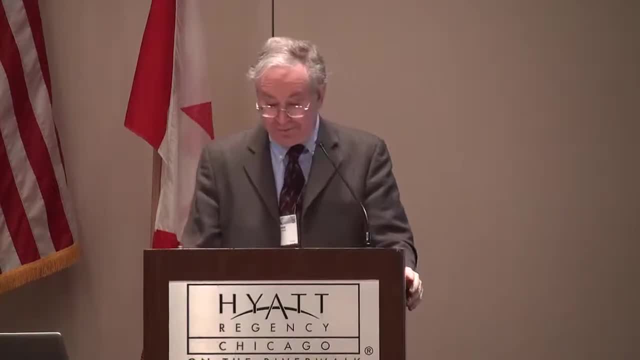 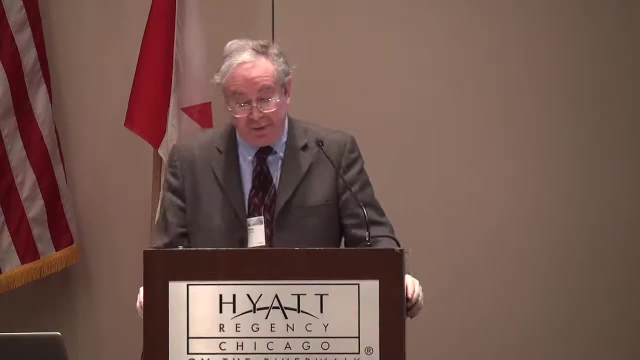 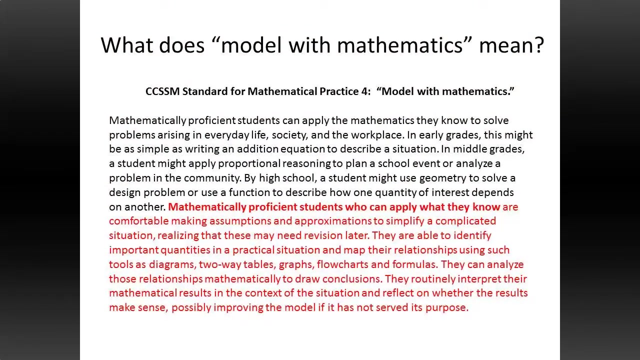 This would have made a difficult problem Even more difficult. Now let's compare this modeling diagram with the second half of the CCSM-SSM Standard for Mathematical Practice. Mathematically proficient students who can apply what they know are comfortable making assumptions and approximations. 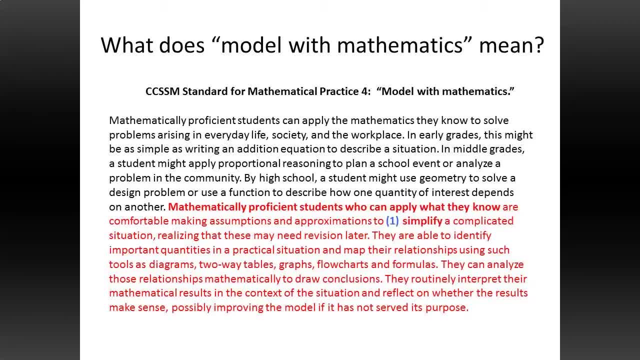 to simplify the first thing, To simplify a complicated situation, realizing that these may need revision later. They're able to identify important quantities in a practical situation and map their relationships using such tools as diagrams, two-way tables, graphs, flow charts and formulas. 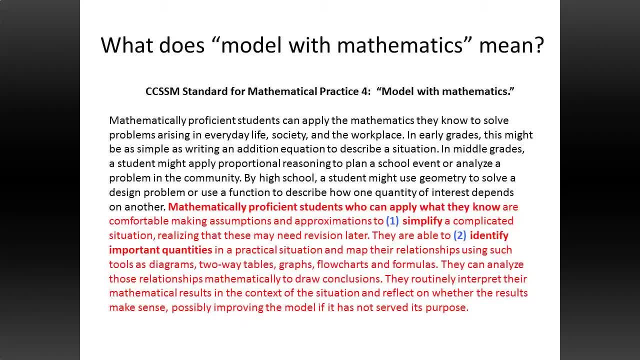 I used two-way tables. They can analyze their relationships mathematically to draw conclusions. They routinely interpret their mathematical results. They interpret them, which I did in the context of the situation, and then they reflect on whether the results make sense. 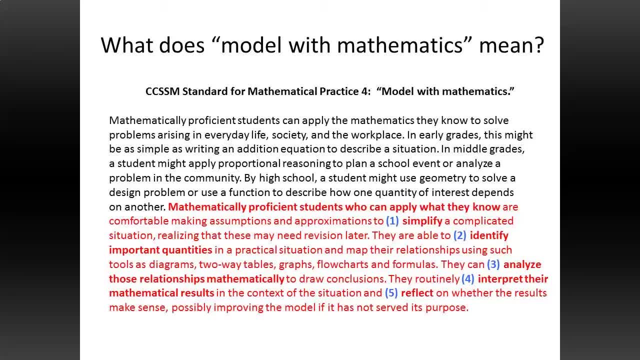 possibly improving the model if it has not served its purpose. Do you see that this modeling standard has two parts, One to apply, the other to model? It's very interesting. I don't even know if the writers realized when they were writing it. 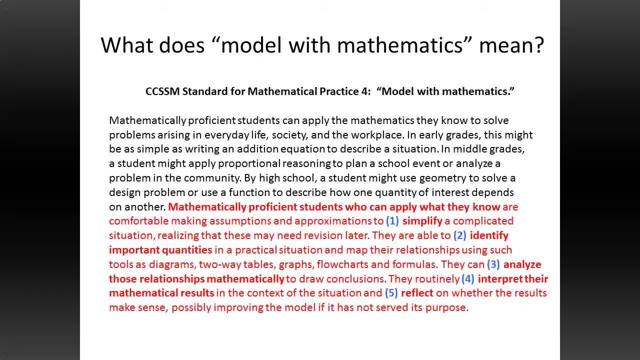 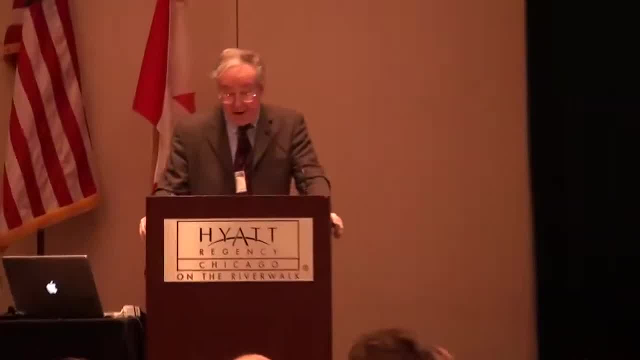 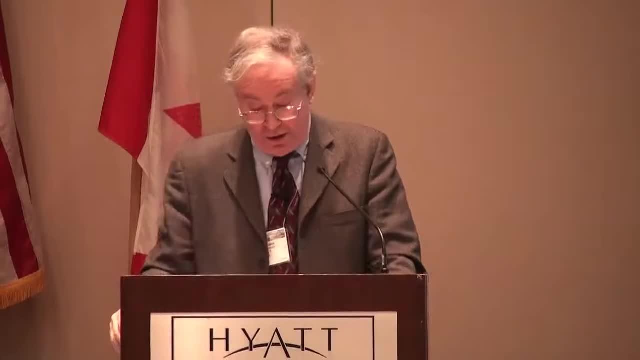 that they were doing this. We model all the time. University courses in mathematical modeling are often at advanced levels and they may lead people to believe that the mathematical modeling process is very difficult, But mathematical modeling is not an arcane activity or one that just professionals do. 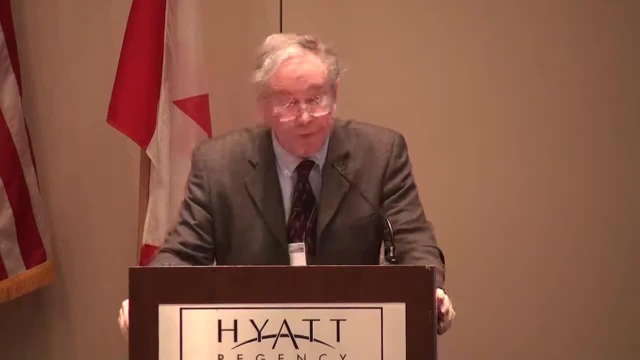 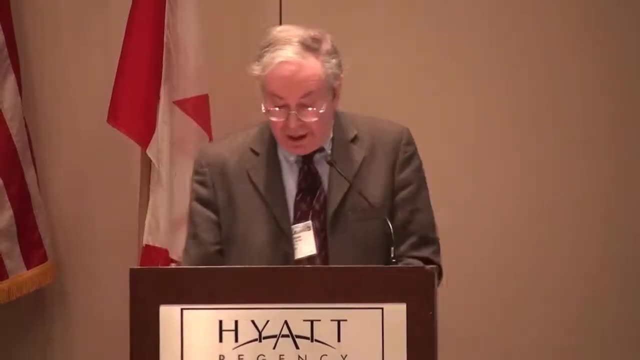 It's so common that it's incumbent on us to understand what modeling can do and what pitfalls we should try to avoid. Teachers, in particular, come into contact with modeling in a variety of ways. In terms of the modeling process, the problem to model is that we want to know. 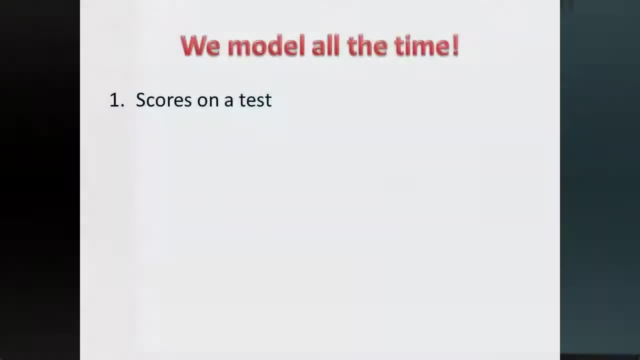 how much a student knows about a certain topic or area. This is an impossible test, so we simplify the problem by selecting a few things we think are important, asking what the student knows about these things. We call these things test items. We assign weights of importance. 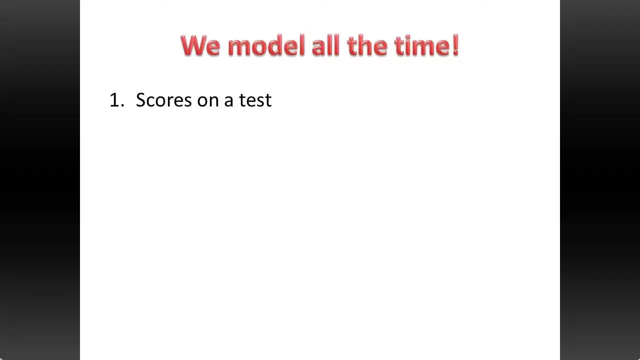 to each test item we've selected. We usually call the weights points And we decide to add the weights to get a single number representing what the student knows of the area. These weights are the mathematical model of what we think is important and the sum of the weights 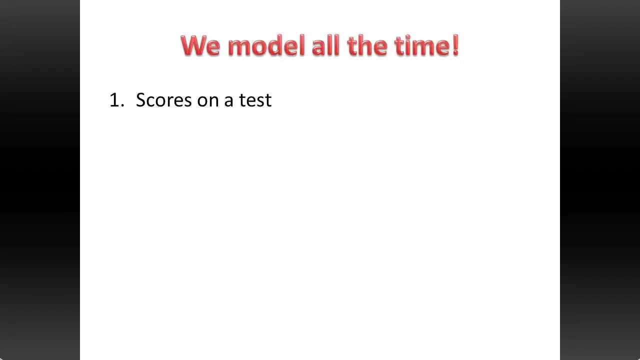 is the mathematical solution to our problem. Now we have to translate that solution into the real world, often to give a letter grade. Let's look at the theory of this grade. Did too many students fail based upon the model we used? If so, we may deem the model as unsuitable. 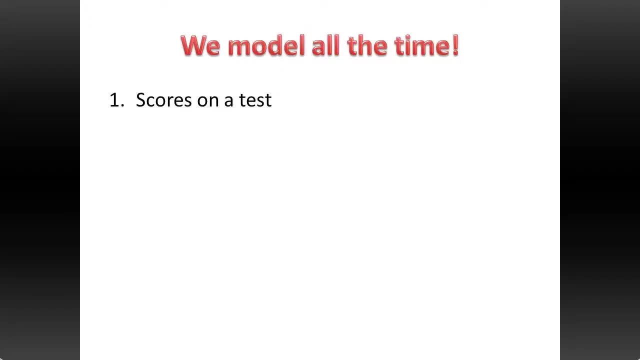 We may wish to curve the test, That is, to change the model. We may even change some weights if an item does not act as we expected. That is, we create a model that we hope accurately indicates performance. We work with that model. 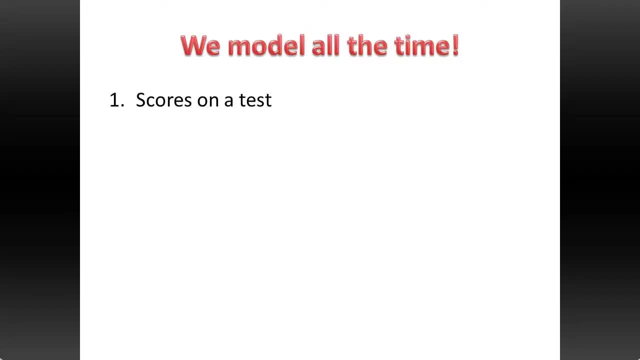 and, unless we're quite rigid, we look at the grades that the model gives us and test those grades for feasibility and accuracy. Are the students we think know the most about getting the highest grades is a question we will ask ourselves. You get the idea. 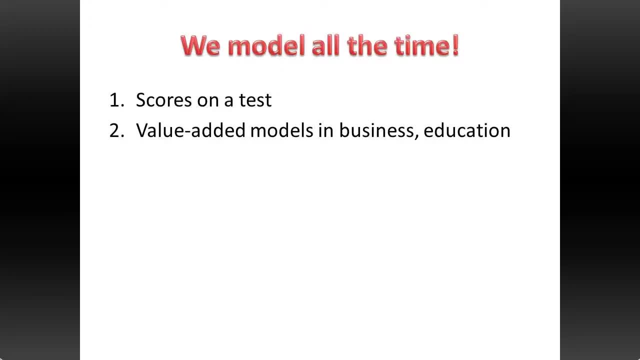 In business and economics, value-added models have become common. This is an attempt to measure the worth of something by mathematically comparing a scenario before a treatment is undertaken and then, after the treatment is undertaken, to ask: how much has the treatment influenced the change. 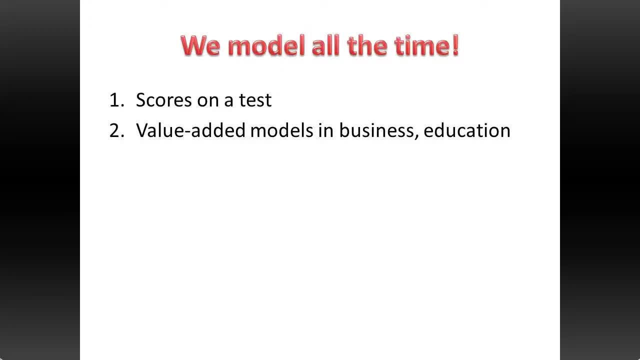 Some people want to evaluate teachers based on a value-added model. These models are very controversial because the translation from the school world into the mathematical model requires an extraordinary simplification of the real situation, namely a simplification that ignores the effects of student attitudes and abilities. 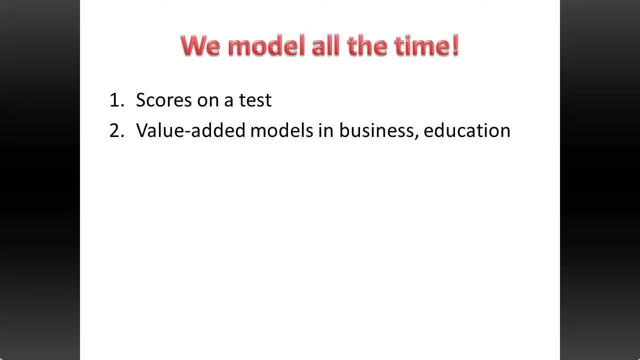 and the overall culture of a particular school, Not to mention the randomness that just occurs when third period doesn't act the same way as fifth period. The third type of model is commonly treated in school mathematics but not viewed as modeling. We have lots of mathematical ways. 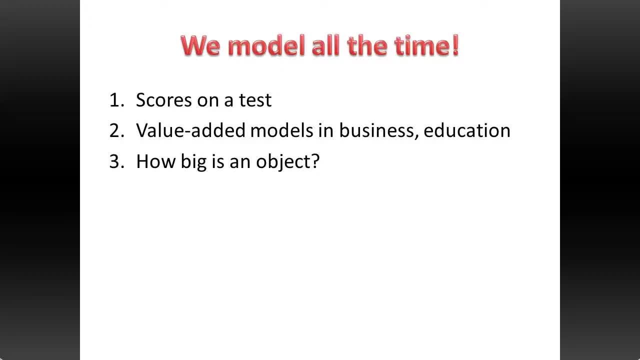 to answer that question, Consider an object like an airplane. We might describe its size by its length, its wingspan, its height off the ground, its weight- the maximum weight it can handle and the maximum number of passengers it can handle. 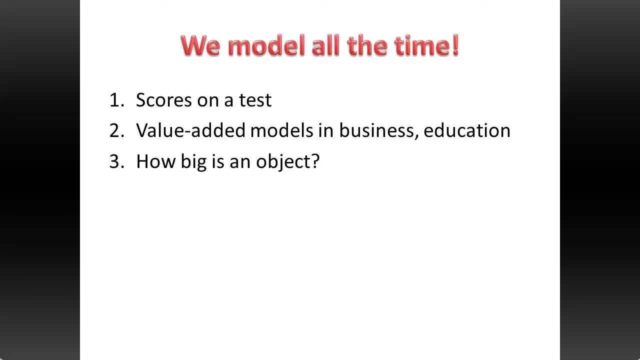 And maybe you can think of a few other variables that we could use to describe the size of an airplane. We recognize that you cannot describe an airplane's size by a single number. You need a few numbers. And yet some people believe you can describe. 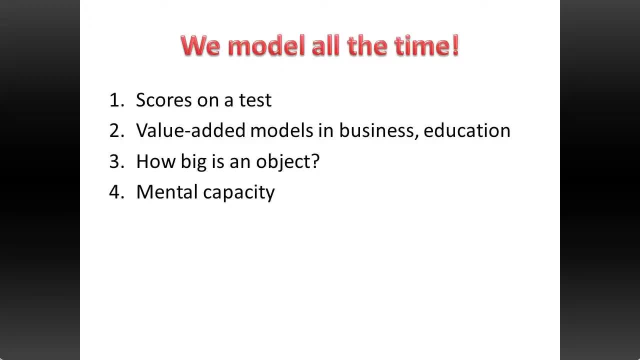 a person's mental capacity by a single number- IQ. Could anything be so foolish? But it's the simplicity of a single number, the attractiveness of a single number, that has us use single numbers to determine all sorts of things, from the batting champion of the major leagues. 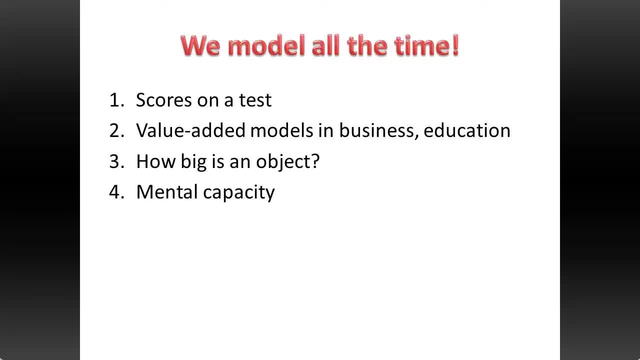 to comparing the educational systems of different countries. One number, How silly. I needn't tell you that scale models of buildings and manufactured objects are geometric models. Most photographs are two-dimensional models of three-dimensional situations. We work with these models to determine information. 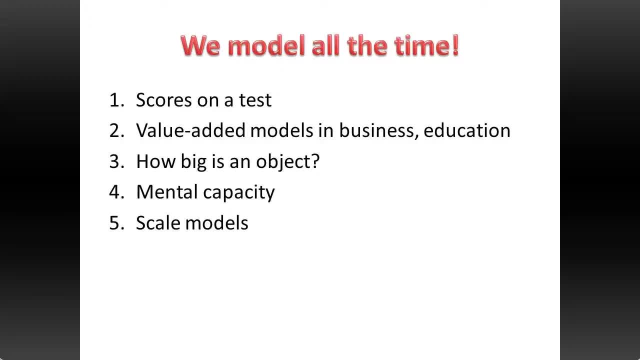 about the actual situation and translate what we have found back to the situation. For this, ratio and proportions are exceedingly important and we use geometric models. in algebra We teach that the path of a ball thrown by a person or hit by a bat or a golf club. 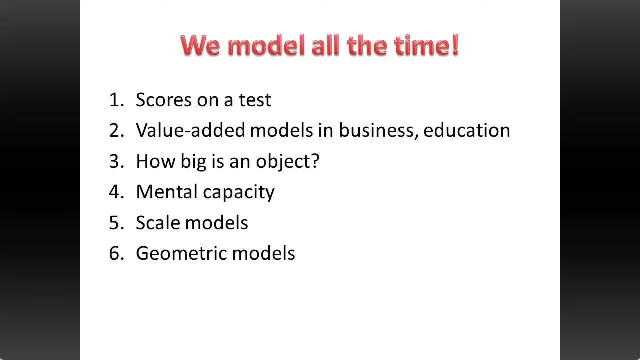 or the path of a bullet from a rifle or a gun, and, more generally, that the path of any projectile, an object that is thrown or shot is a parabola, And we know that a parabola can be described by a quadratic equation. The parabola may be thought of. 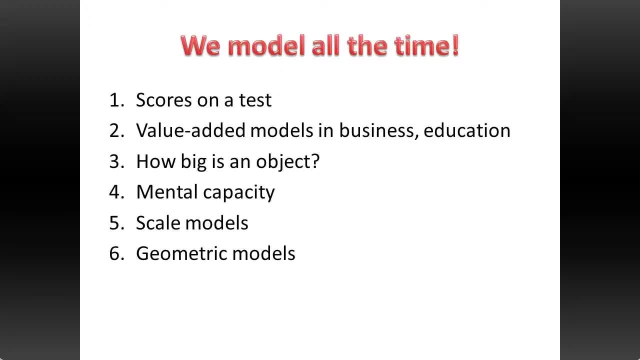 as a mathematical model, a geometric model of the actual situation. But what is a parabola? In order to exactly be a parabola, the force of gravity would have to be constant. There would have to be no wind or other force acting on the projectile. 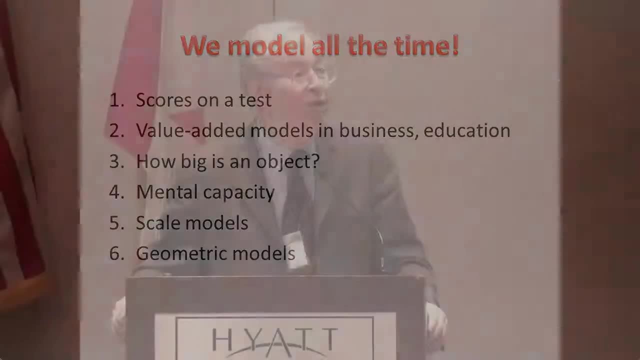 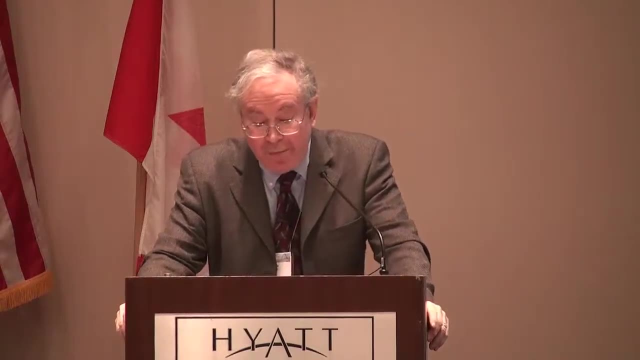 and there would have to be no spin. You know, in baseball it's not just curve balls that curve. all the balls curve somewhat, they all move. Paths of batted balls can be affected quite a bit by the wind, If you've seen golf on television lately. 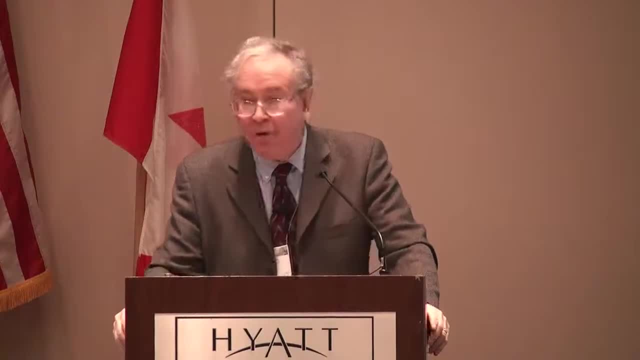 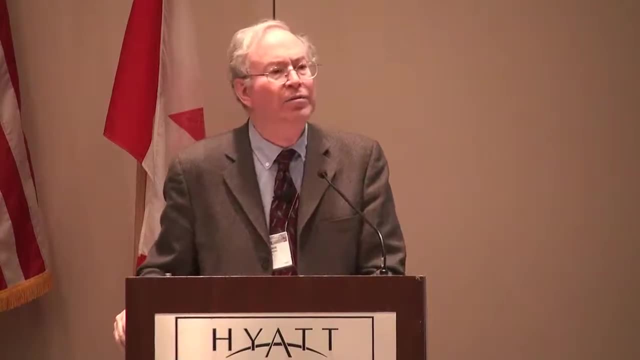 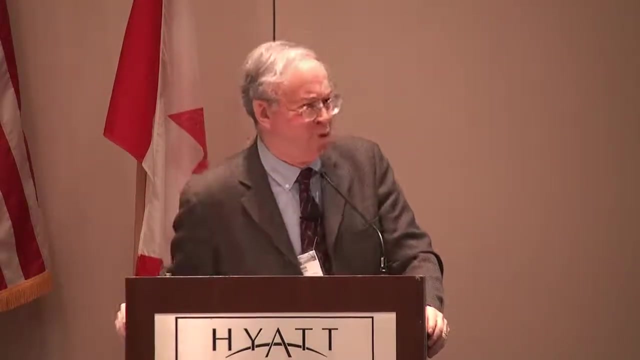 you've seen the latest technology that tracks the path of a golf shot from the tee to where it lands. Rarely are these paths straight. All these paths, in fact, are rarely coplanar. So we assume that there's no spin, no wind, constant gravity. 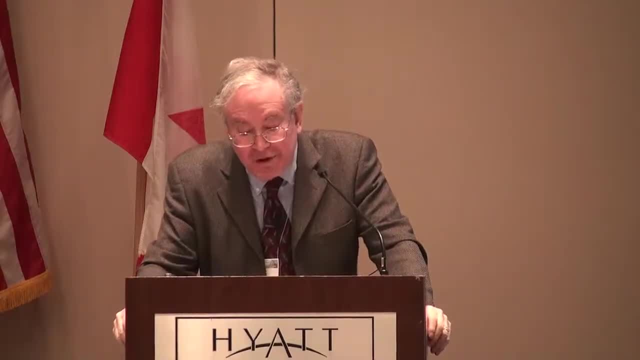 and then we get a parabola. That's our model. We make assumptions in physical situations for the same reason that Mitchell made the assumptionist golf problem of 40 golfers, not 41. To treat the actual path of a projectile is very difficult. 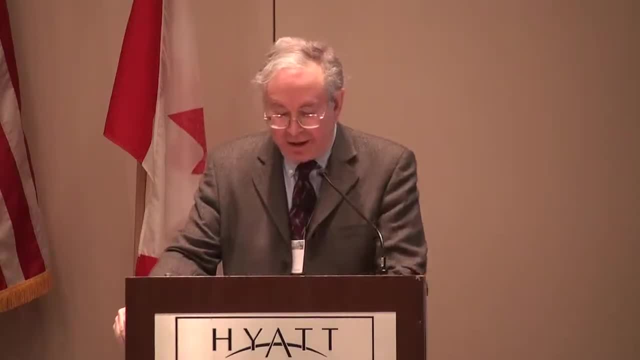 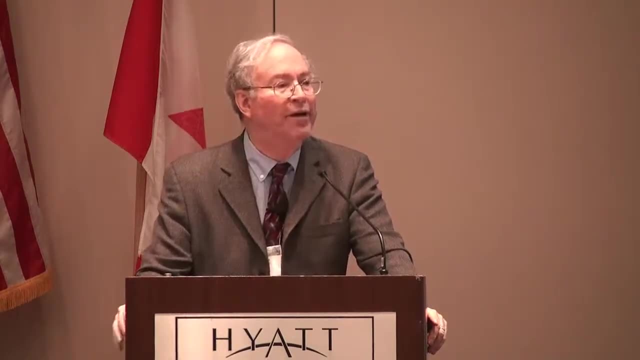 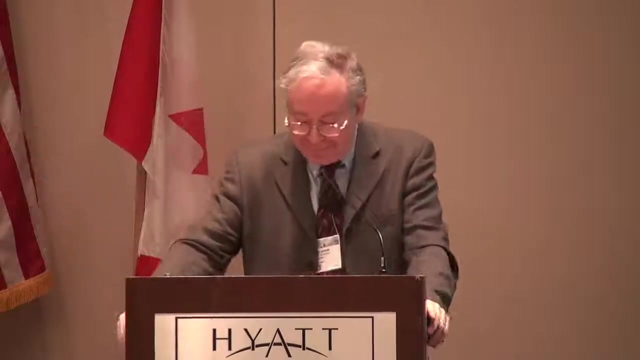 A simplified path is good enough for many purposes. It tells us that under ideal circumstances, the peak height of a fly ball in baseball is halfway between the batter and the fielder And the fielder who catches it. that is Not just any fielder. 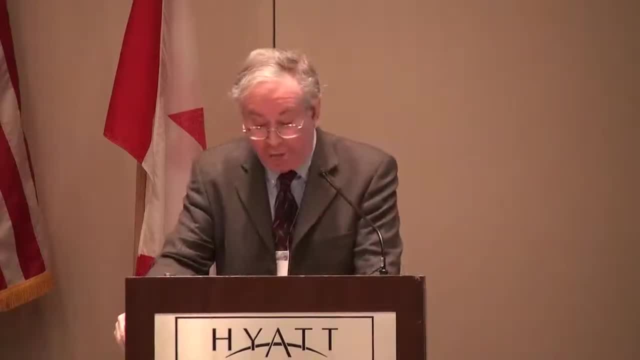 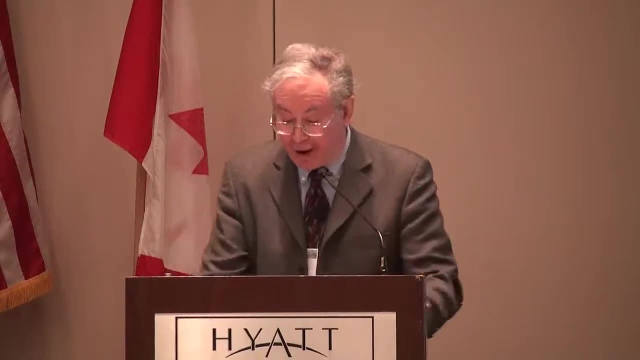 Something that would surprise many people, for it's a common belief that a ball comes down in a path that is more vertical than it goes up, And, by assuming the path is a parabola, we can estimate reasonably closely how far a home run would have traveled had it not been. 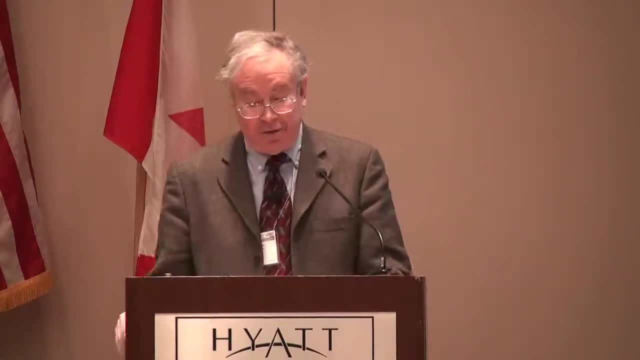 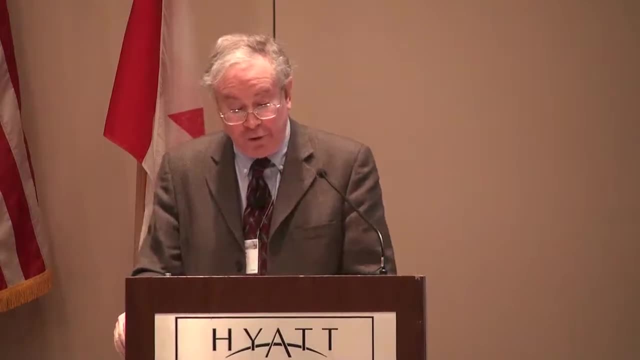 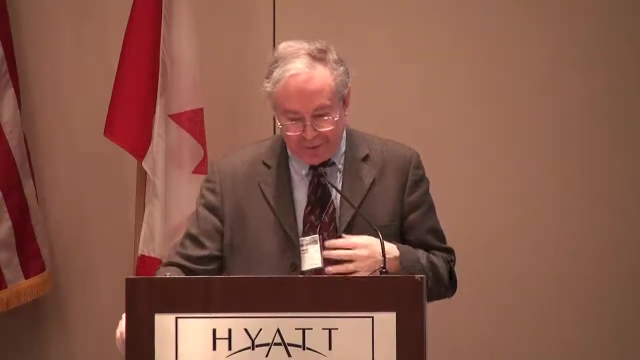 stopped by seats or bleachers. And I needn't tell you that before the days of heat seeking and other projectiles that can change course in flight, calculating the path of a parabola from a few bits of information was important in warfare. I like to distinguish three types. 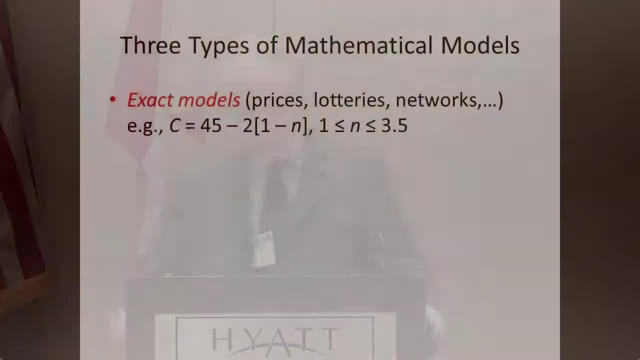 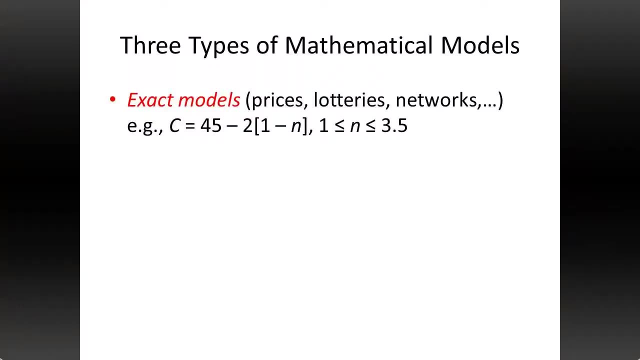 of mathematical models. Some models are exact models, Either because they're based on counting or iteration, or because the application arose from the mathematics. The mathematics came first. For example, compound interest is defined from a mathematical formula. It arises from the mathematics. 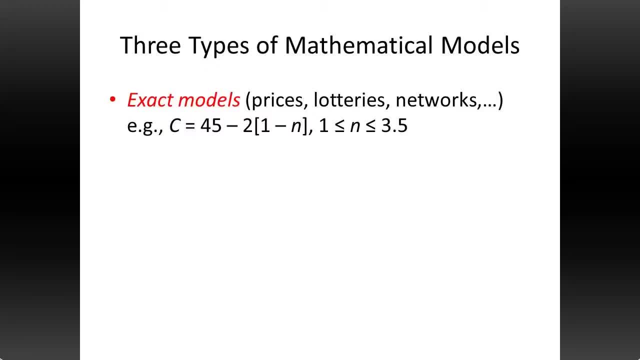 Similarly, lotteries are merely mathematical games played with people. Now I've given a formula here for the cost C of mailing a letter first class in the US weighing n ounces, for 1 is less than or equal to n less than 3.5. 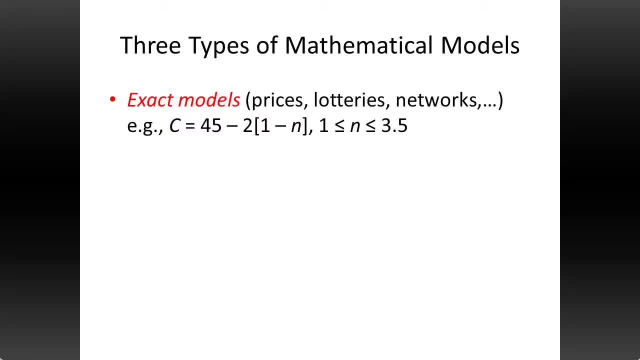 from 1 to 3.5.. And it's given by this formula, where the brackets stand for the greatest integer function. greatest integer less than or equal to 1 minus n. Exact models are isomorphic to real situations. This one works. A network of airplane routes. 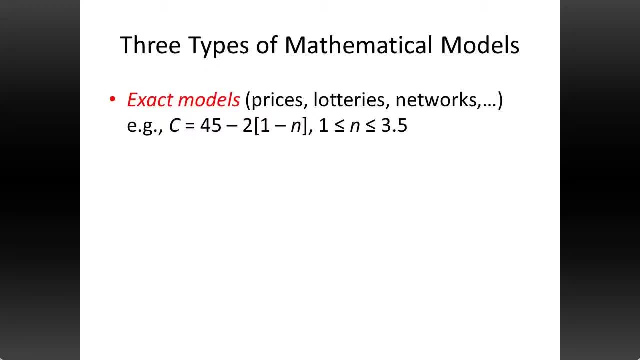 provides a geometric example, While this kind of mathematics is not always considered to be modeling, because there's no testing, there's no estimation, there's no feasibility, it's just there. You don't think of it as modeling, but these are mathematical models And it provides a groundwork. 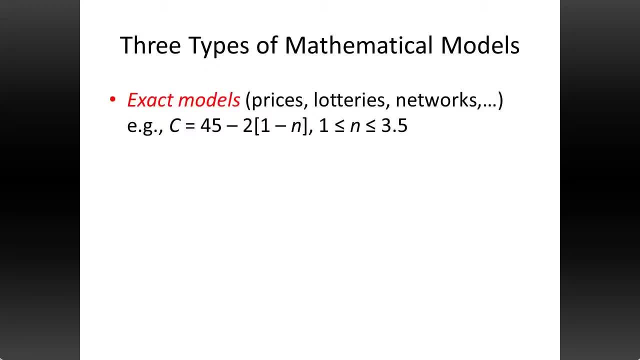 for other messier situations, particularly in teaching. It's nice to start with this. A second kind of model is the almost exact theory based model found in applications of the physical world. A football is kicked. it travels to a height of 40 feet and lands 50 yards from where it is kicked. 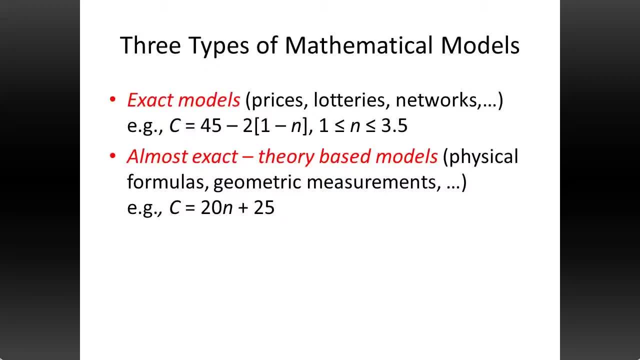 Describe its path. In the postage example just mentioned, avoid the greatest integer function and use c equal 20n plus 25, and then you get one that works for the whole. it works for the whole numbers, but it doesn't work in between. It requires rounding. 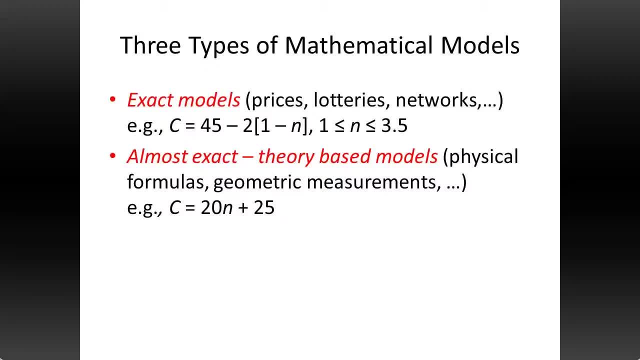 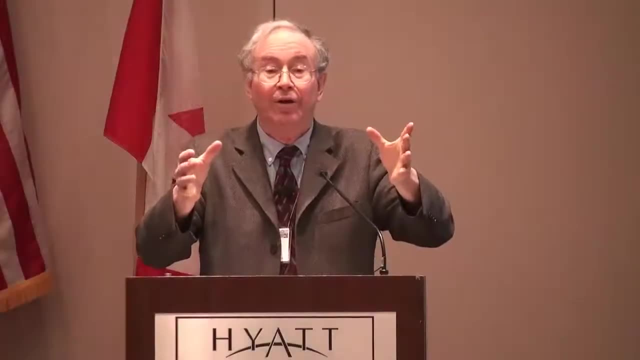 So you say, oh yeah, what you do is you round up first and then you use this model: Find the volume of a can, any can. given its dimensions, It seems like it might be exact, except for the errors in measurement. but in fact few cans are really cylinders. 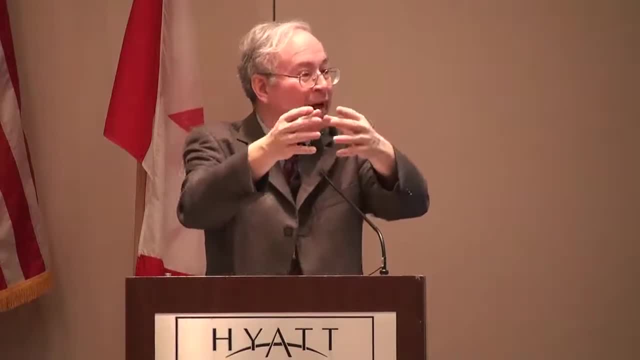 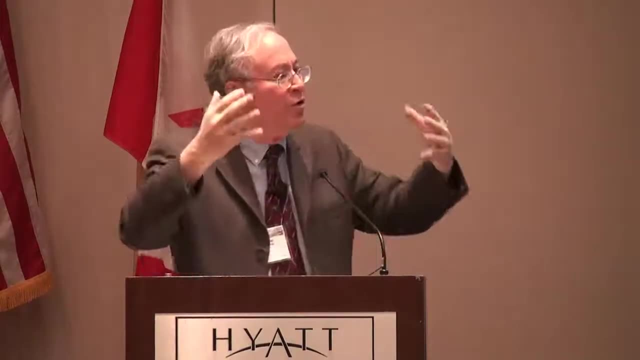 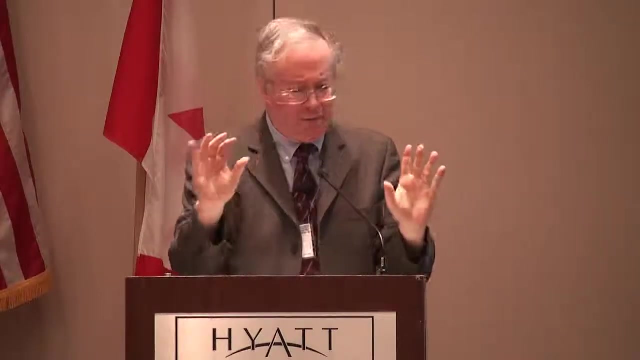 If you really look at a Coke can or a tin can for tuna, you see that there's ridges all over the place. So what we use as a model volume is: whatever the area of the base times the height of a cylinder. we use that, but that's an approximation. 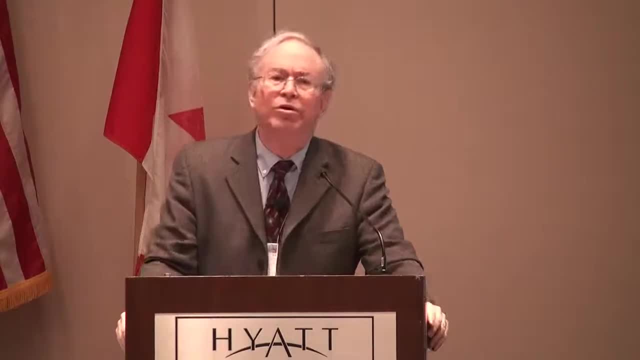 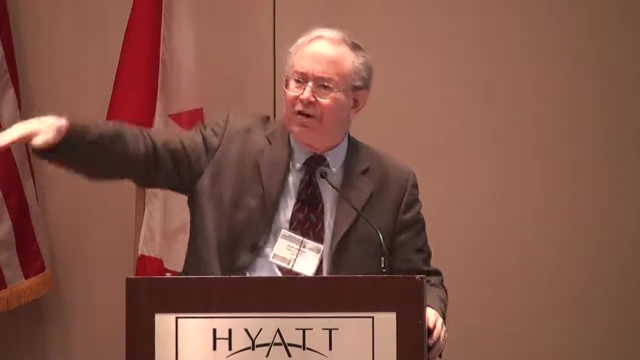 An oven is heated from room temperature to 350 degrees. How does it go up? Well, it might start out exponential up to 350, but it doesn't just keep going. It kind of hovers up and down, turning off and on, to maintain at 350. 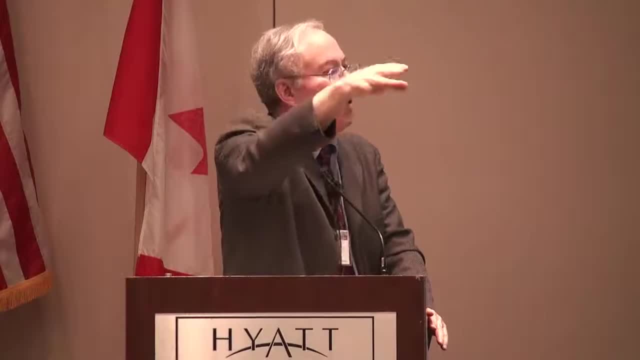 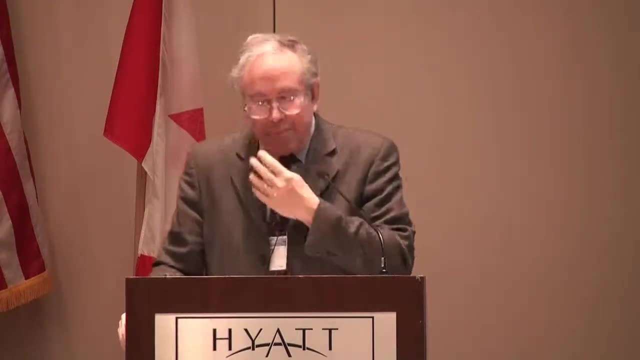 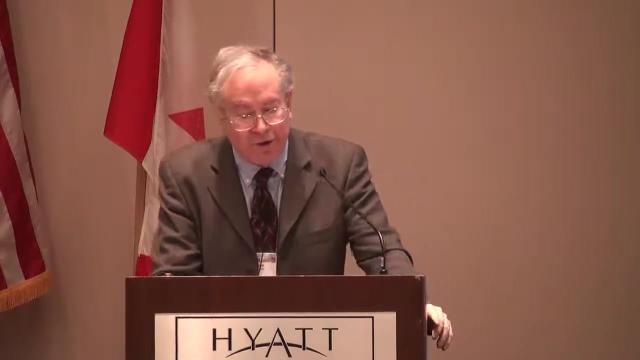 so it becomes almost like a sine wave after it gets there. So these assumptions that we make presume an exactness that's not possible in this situation. Measurement error, the necessity of rounding statistical variability, other factors, force our models to be only an approximation of reality. 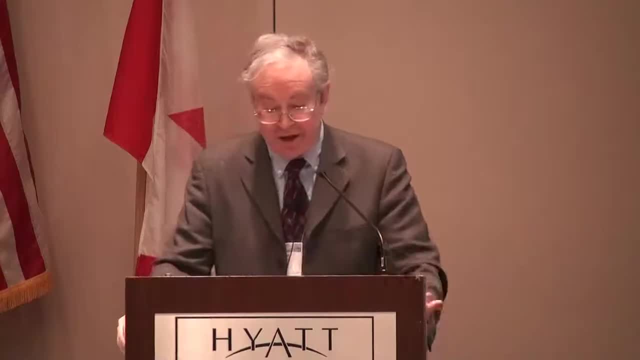 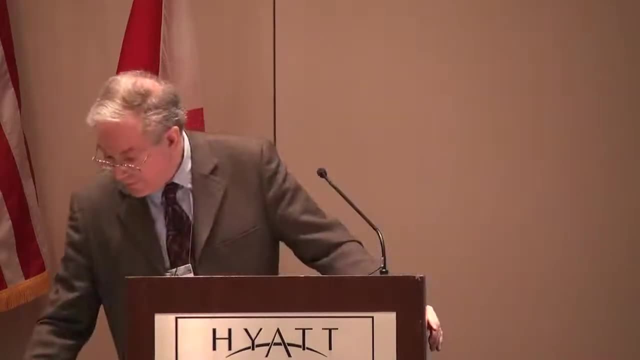 Though some error is known to exist, one person can still trust to some extent the results obtained by using the model. These are the kinds of models that are usually found in textbooks. The third kind is the impressionistic model, A model that seems to fit a real situation. 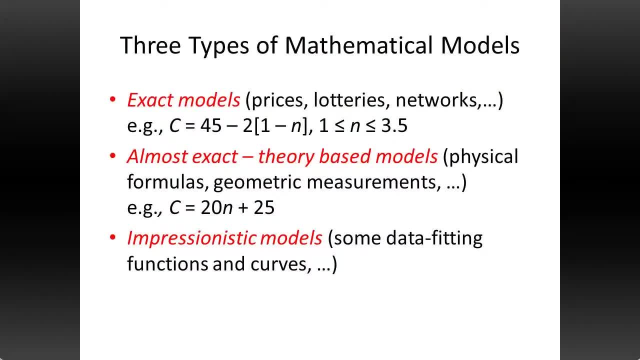 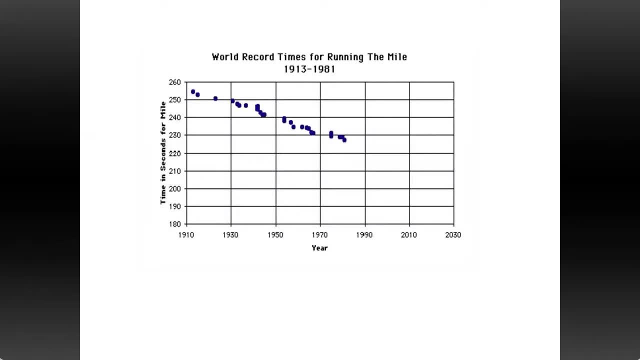 but which is derived from no hard theory. For instance, here's a graph of the world record for running a mile from 1913 to 1981.. Looks pretty linear. Must go on forever, Right? I mean, you know when will the record be zero? 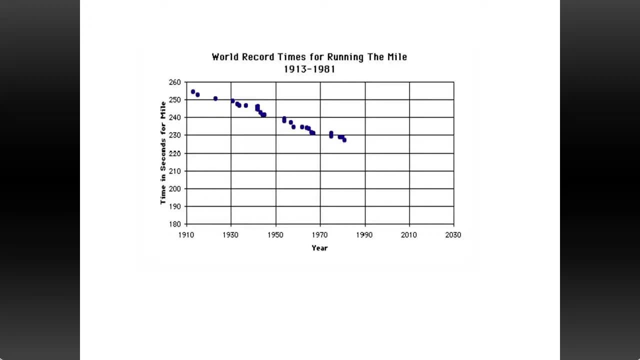 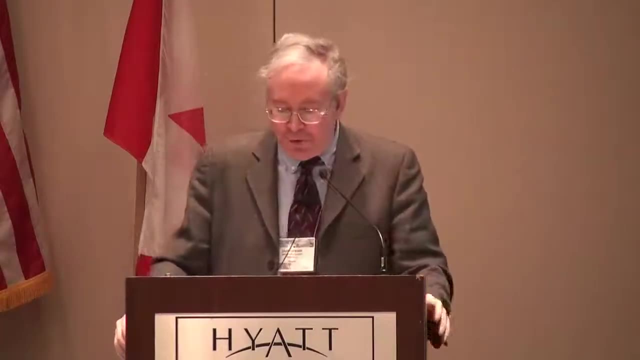 When will you get there? Five minutes before you started, So we can ask all sorts of questions. These tell us, of course, that this is not. This is a model for that time frame. Here the record is linear or almost linear, for two reasons. 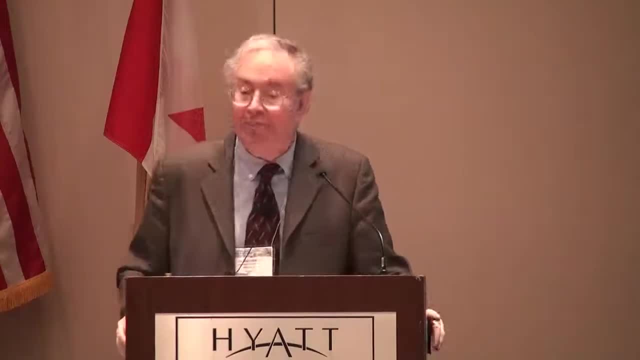 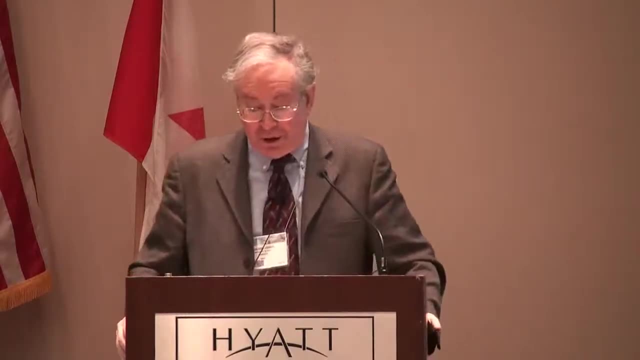 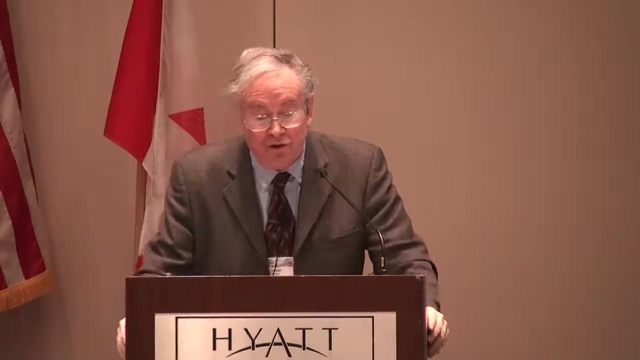 First, because it's a record, the function relating year and time must be a decreasing function. Second, any smooth curve that would fit such a function would be linear when viewed only over a short period of time. It happens that even the 68 years shown of this record is a short period of time. 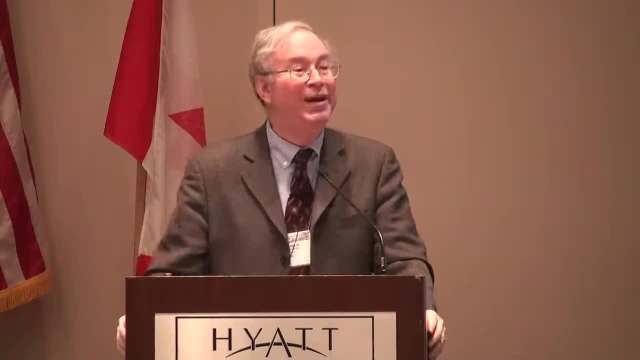 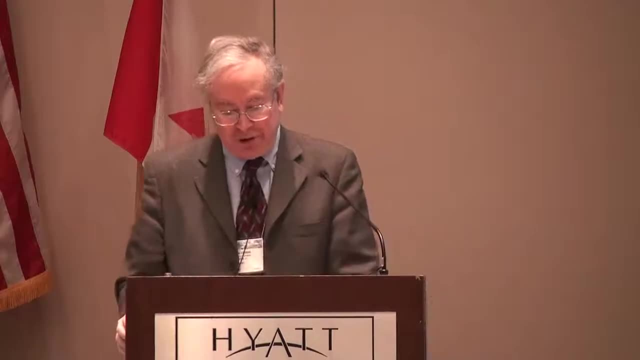 You might use this graph to extrapolate for a few years, but not to go well into this century. It does work for about the next 15 years. I hesitate to say that much research and education and other social sciences fits these models to data. 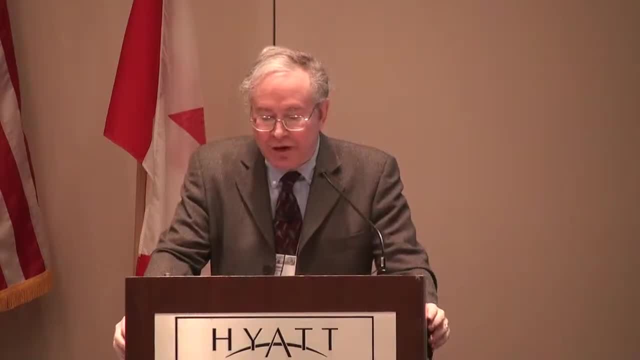 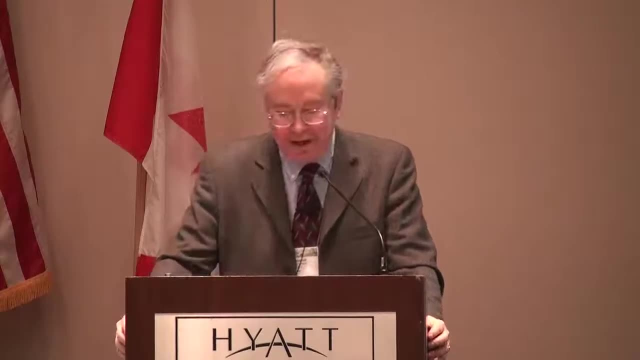 You know this if you've studied linear regression, And in most situations there's no causal rationale for a linear model. The model may work for the given data but may not be generalizable to any other data. The perils of extrapolation are amply seen in this upload. 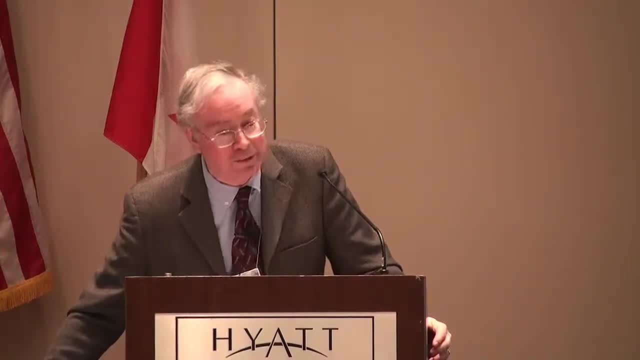 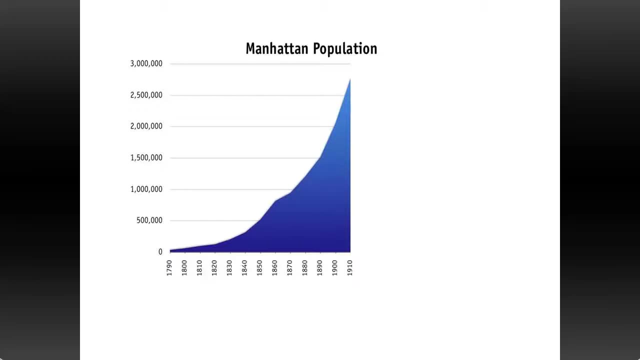 from Wikipedia, the distinguished research journal of the population of Manhattan of over a 110 year period. Here the graph looks like an exponential function from 1790 all the way to 1910.. That looks really exponential And, as you know, we often view population growth. 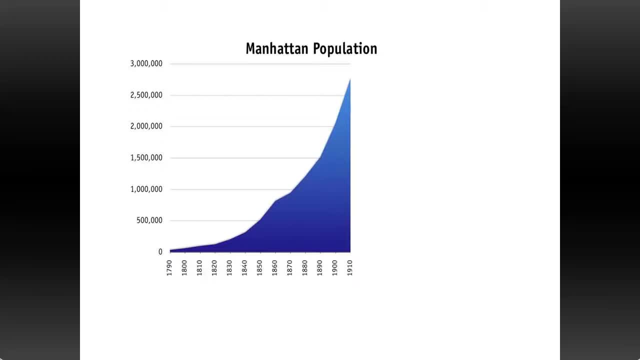 as exponential. But any prediction made in 1910 based on that model would have gone the wrong way. So would a prediction made in 1930 or 1950 or 1980.. When we fit a function to data, as in the mile record, 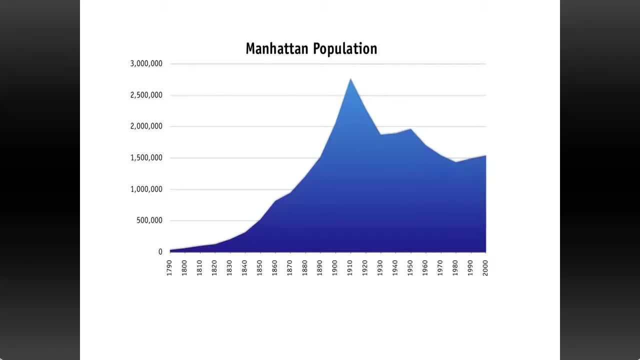 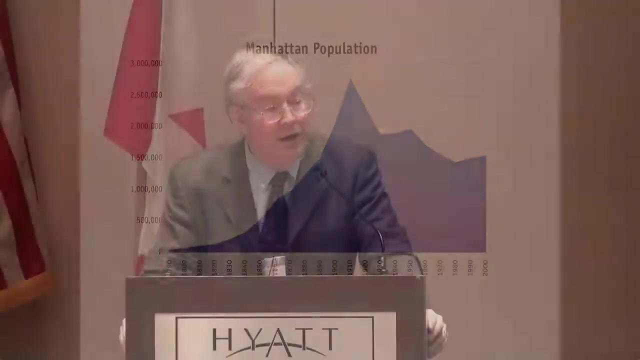 or Manhattan population situations. it's very important to point out that we're working from assumptions about the situation that may be inaccurate or just rough approximations. Some models fit between the almost exact theory based model and the impressionistic model. Among these are models relating 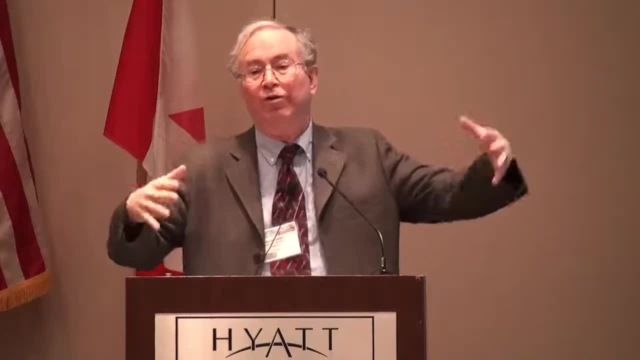 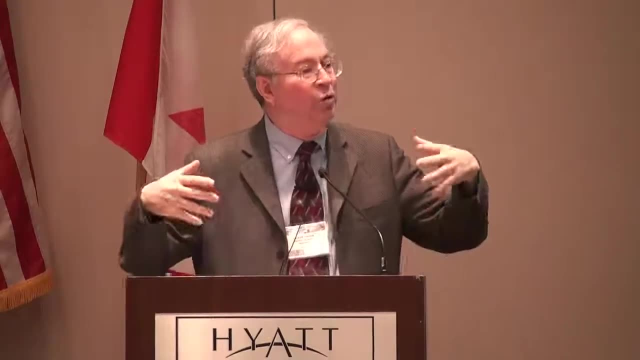 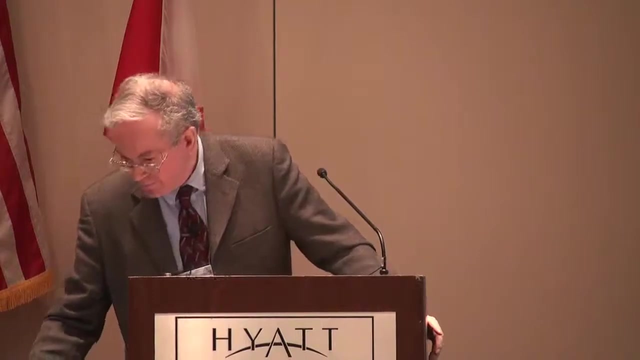 current test scores to future performance. There's a positive correlation between what you know and what you will know, but there's not necessarily a true causal link And there can be major exceptions to any trend that might be established. We move to teaching mathematical modeling. 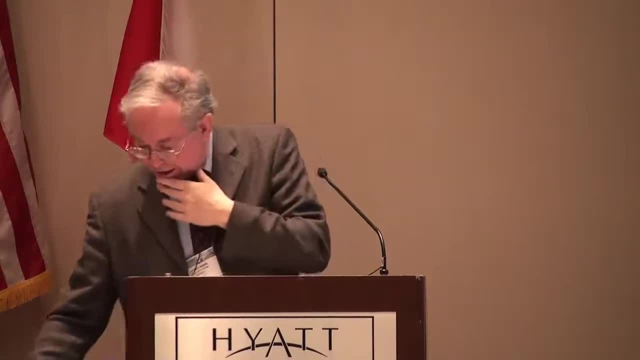 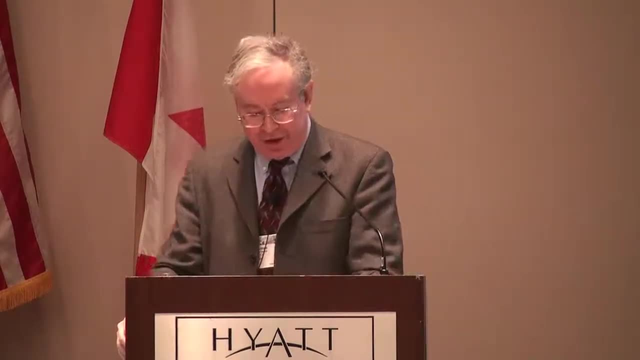 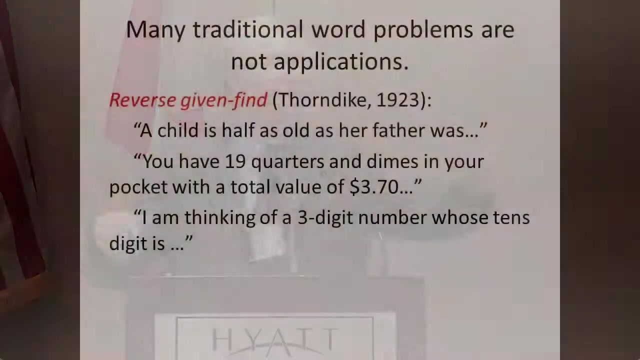 In the 1970s I received an NSF grant to develop a first year algebra course through applications. At the time, what constituted applications in algebra classes began like the ones on this slide. A child is half as old as her father was. You know what I'm talking about. 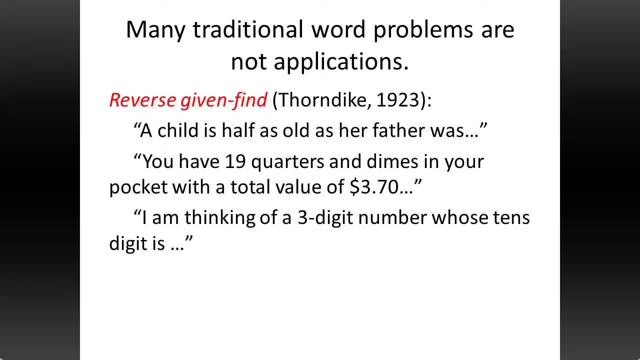 Half as old as her father was when her mother left her. That's the more modern one is: a child is half as old as the man she thinks is her father. You have 19 quarters and dimes in your pocket. You already know the problem. 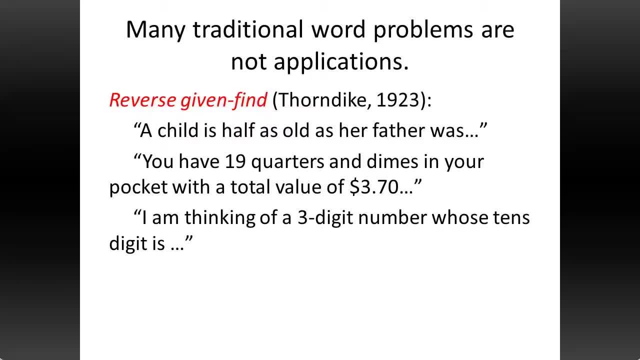 Value of 370.. I haven't even asked you the question. You know what the question is. I'm thinking of the three digit number whose tens digit is. You understand what I'm talking about As a person with a background in pure mathematics. 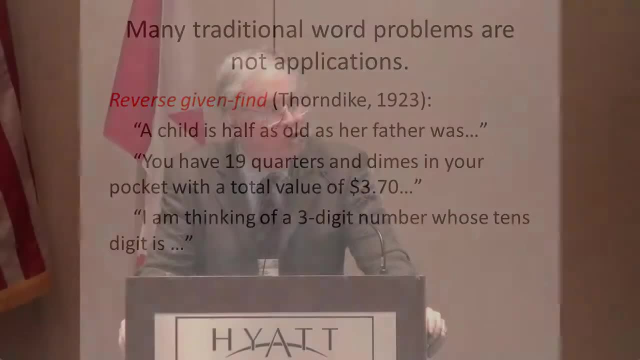 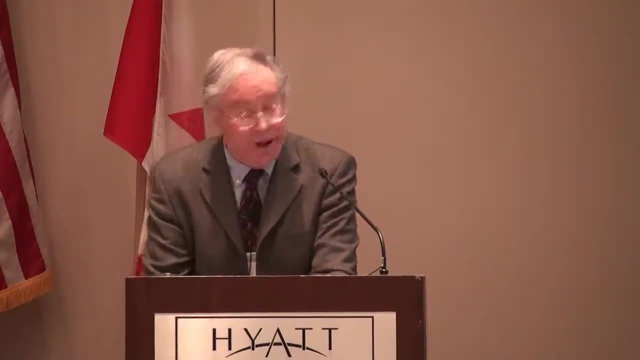 I had little idea of what I was going to do in this NSF backed course. I was supposed to write about applications of algebra, But I did come in with a basic idea that many of these traditional word problems were not applications, nor did they teach students anything. 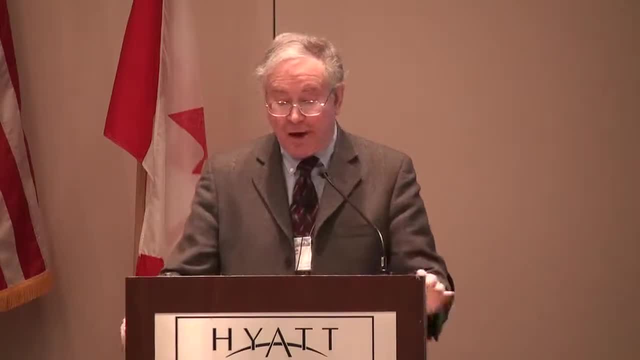 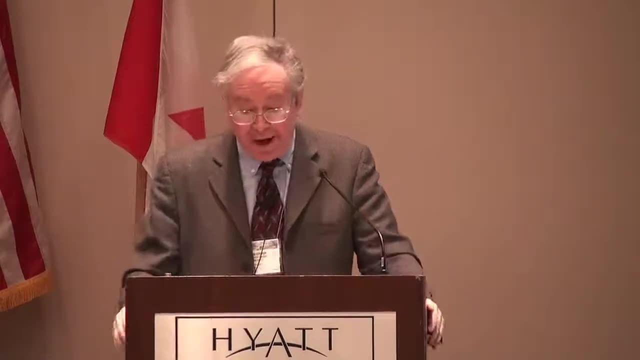 about applied mathematics. They were not applications because so many were what the psychologist E Thorndike called reverse give and find problems. That is, in order to make up the problem, you had to know the answer. How would you know that you had 19 quarters? 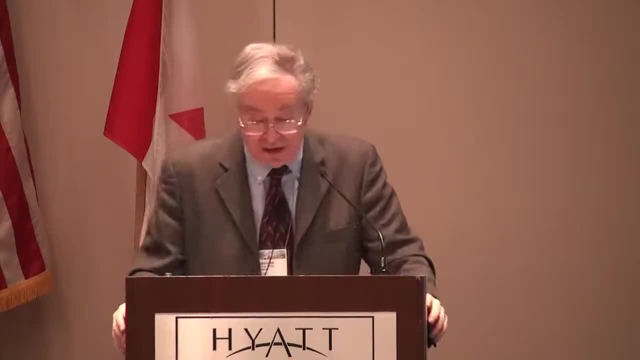 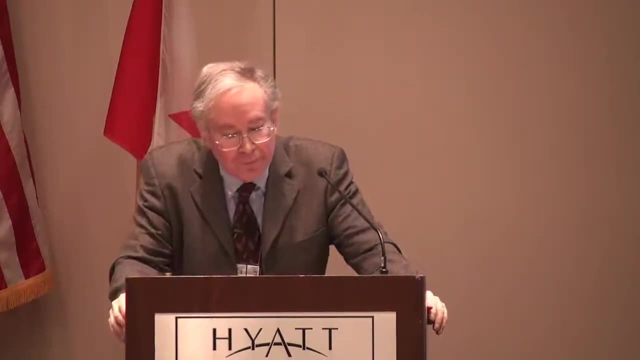 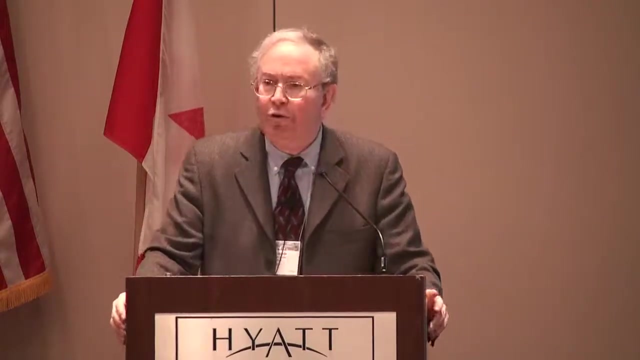 and dimes in your pocket, with a total value of $3.70, if you had not the opportunity to count the quarters and count the dimes. The idea of reverse give and find is found throughout mathematics and it leads to great questions, Given the roots of a polynomial equation. 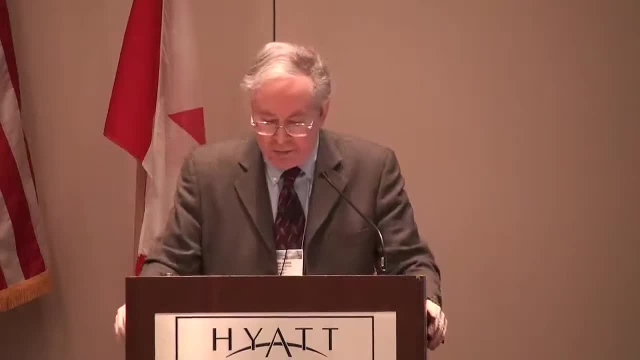 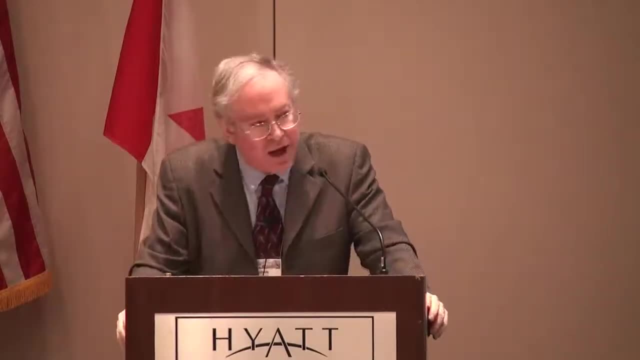 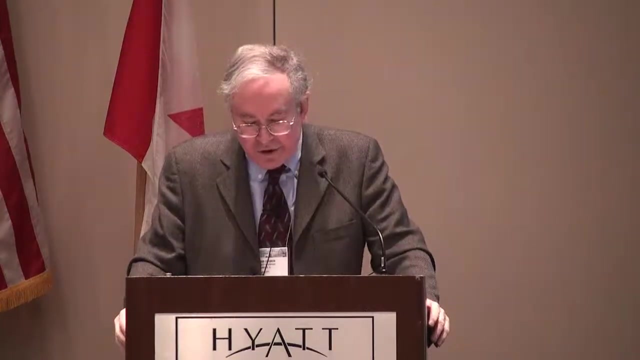 find the equation instead of the other way around. Given the area of a rectangle, find its possible dimensions instead of the other way around. But in real world situations these kinds of questions are typically rather phony. The idea of modeling is that some students see 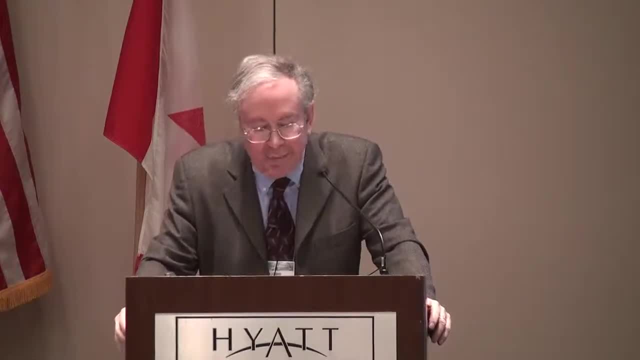 nothing else but these kinds of phony or quasi-phony problems. They leave algebra and many of their mathematics classes without a clue as to why they are studying this content. Why is it required for graduation? Why is this on high stakes tests? Do I really need to know this mathematics? 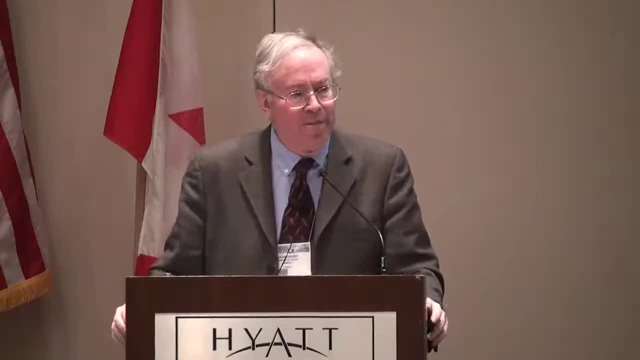 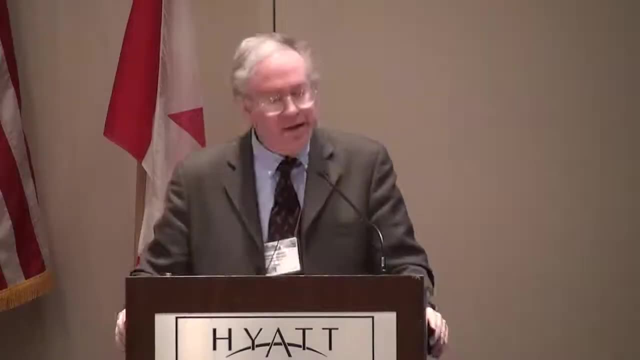 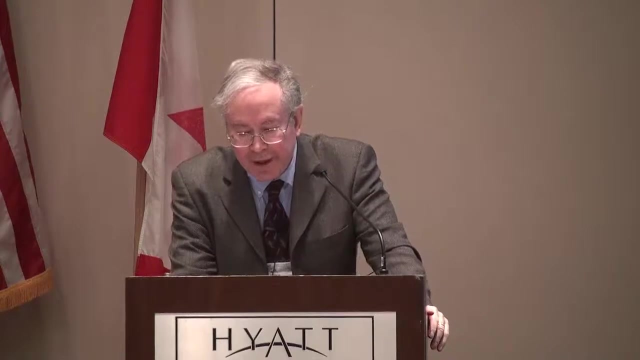 So the point is, many traditional word problems are not applications and not really modeling. Why can't? This leads us to the first of two basic reasons why students cannot apply mathematics well, and I say for algebra here, because that's where it really starts. Students realize they need to know. 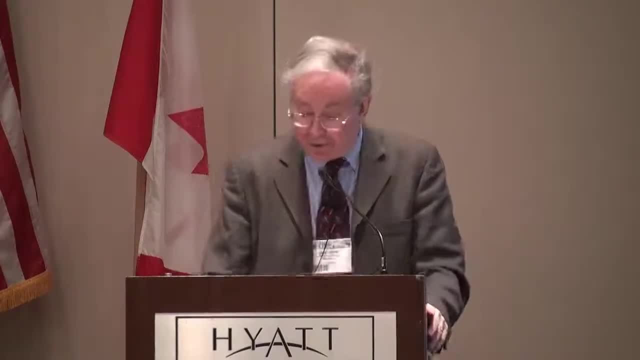 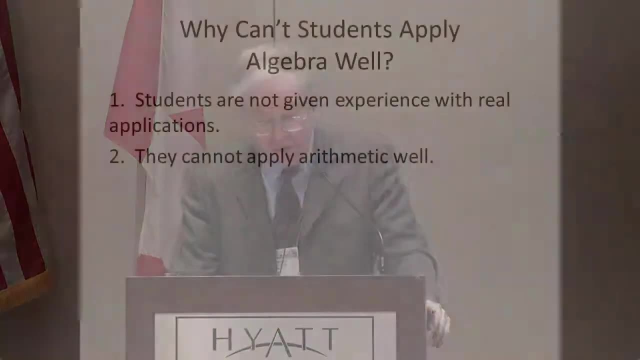 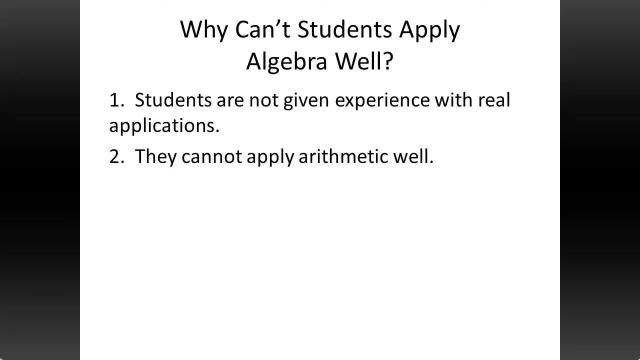 the applications of arithmetic, but when they get to algebra they haven't been taught the applications. It does start with arithmetic, where there is so much emphasis on the early grades on counting and not enough on measuring. No mention of scales of any kind in the calculus measurement formula. 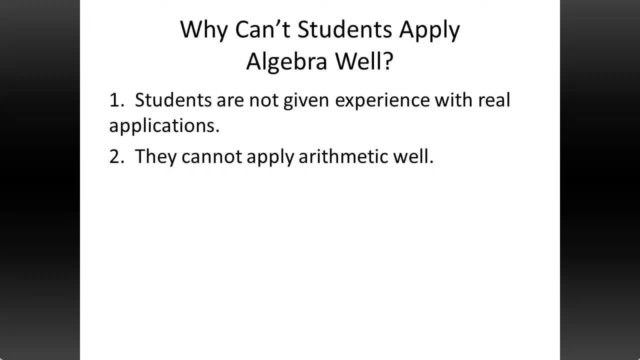 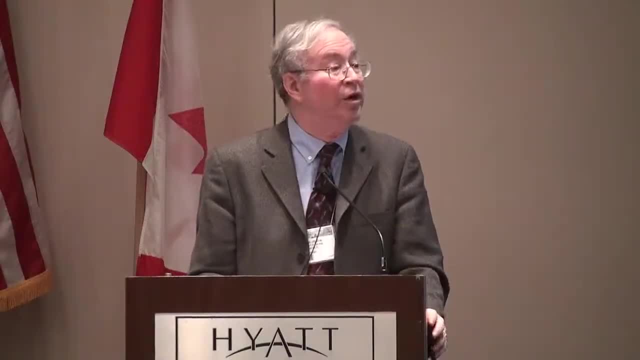 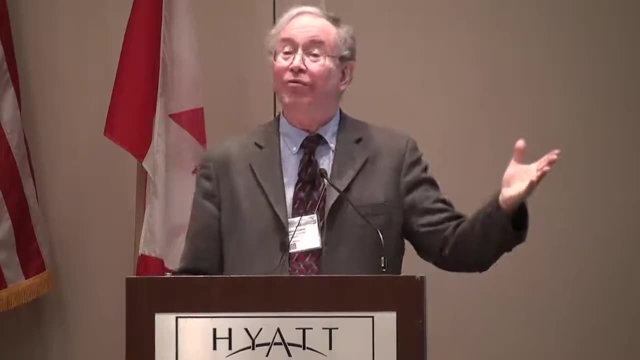 The second reason students can't apply algebra is that they can't apply arithmetic well beyond applications of small numbers and addition and subtraction, they are clueless. Consider the properties of multiplication that we teach. Multiplication is commutative, Multiplication is associative. 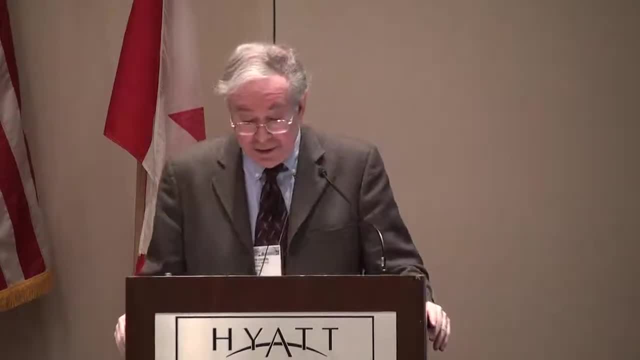 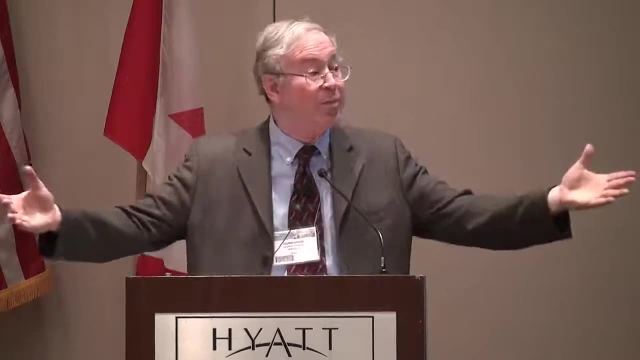 Multiplication distributes over addition. One is the multiplicative identity. The reciprocal of A is 1 over A and, more generally, the reciprocal of X over Y is Y over X. These are the properties we teach in multiplication. And if you ask people what multiplication means, 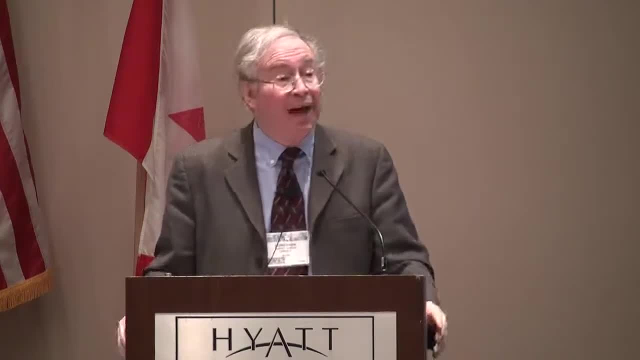 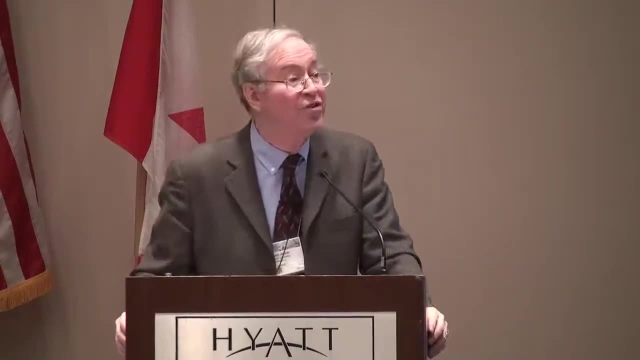 they say: oh, it's repeated addition. As I think everyone in this room knows, repeated addition doesn't work if one is trying to explain 2 thirds times, 4 fifths or 35% of $150.. You can multiply if you're in a grocery store. 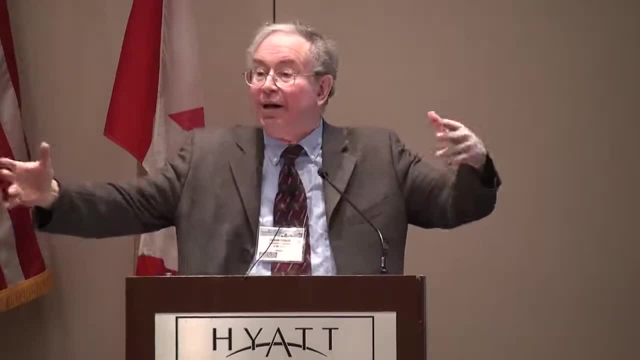 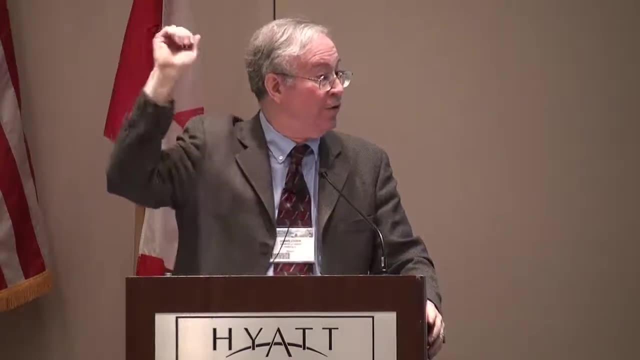 You buy 6 cans of beans, they cost $1.19 a can, instead of adding $1.19,, $1.19,, $1.19. that's what they do. The cashier does that, But we know, because we know we could just multiply by 6.. 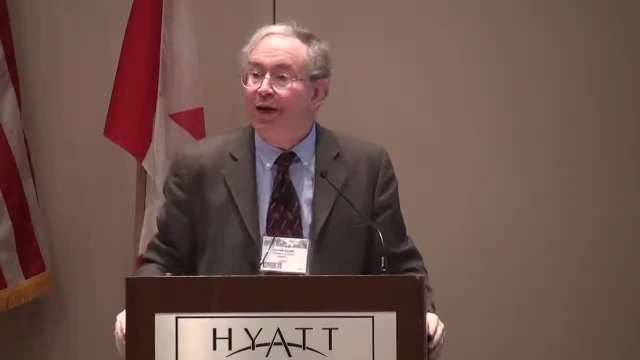 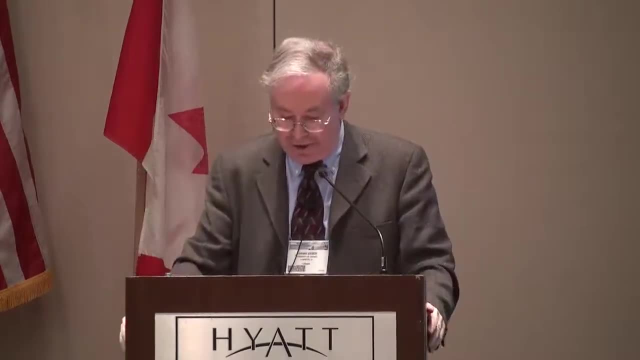 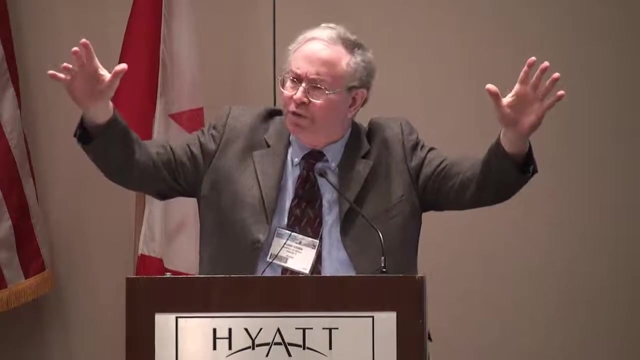 We get 6 times that. But that's not a multiplication situation, That's an addition situation. It is not applying multiplication for what multiplication does. As a consequence, many students leave. students have keywords for addition and subtraction. put together Total Takeaway. 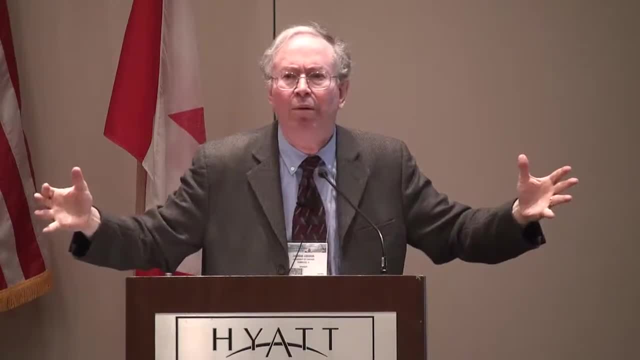 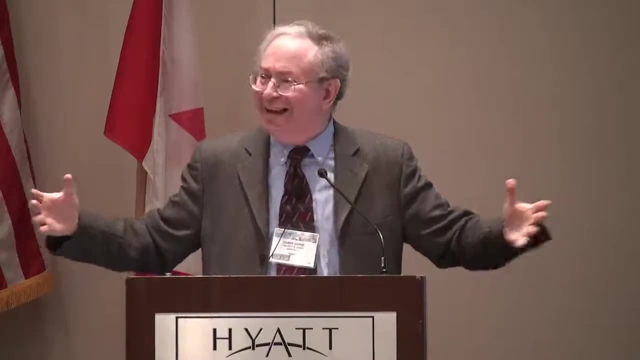 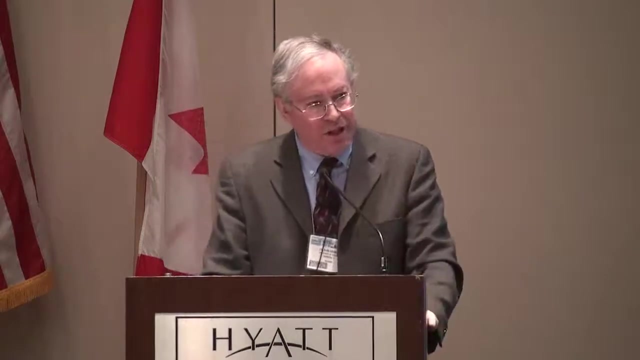 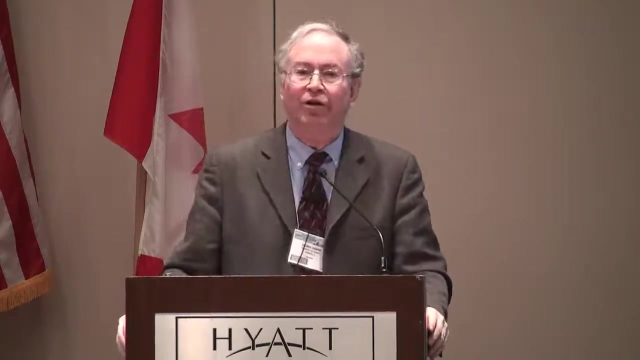 They have these words. What for multiplication? Times, Times, That doesn't do anything. That's what the symbol is. As a result, students have to memorize formulas such as D equals RT or A equals LW, without realizing that these formulas result from essential uses of multiplication. 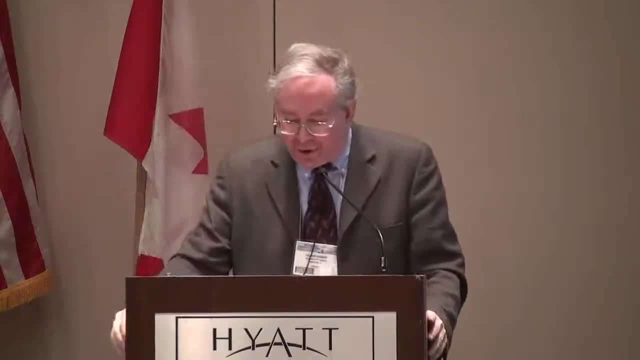 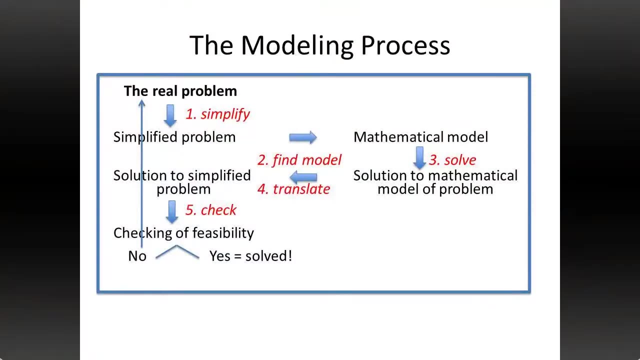 and rate factor. If we refer to the modeling diagram, the same diagram I showed before, we see that this analysis exposes a gap in the curriculum of many students. There is little or no instruction in the finding of the mathematical model in number 2. Students have no place to turn. 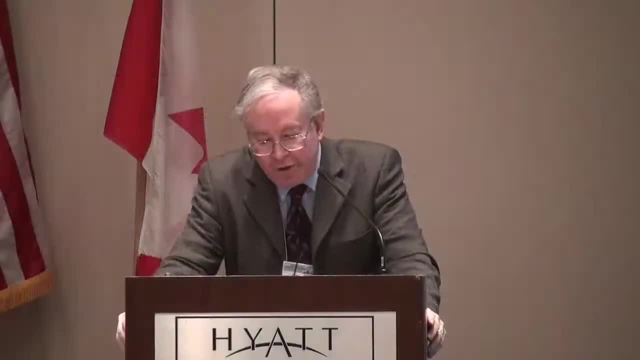 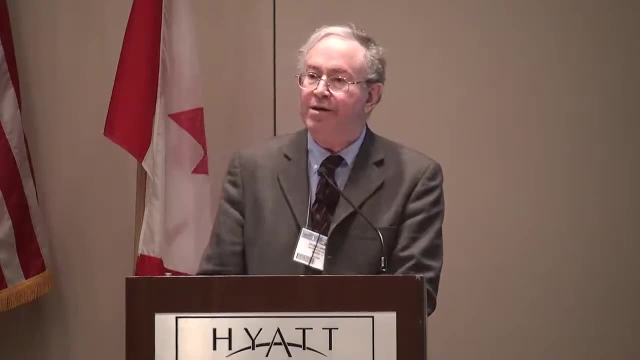 except to memorize without understanding. In the 70's we thus began a practice that, I'm happy to say, has been picked up in a variety of ways by curricula. in many places in the Common Core Standards That practice is to emphasize in a quasi-formal way. 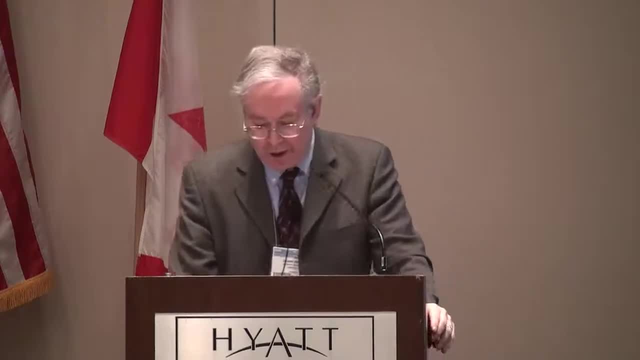 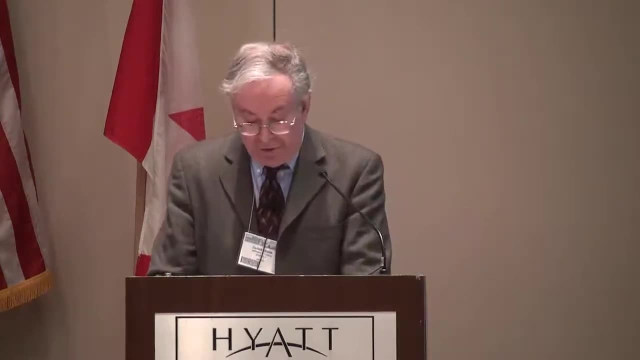 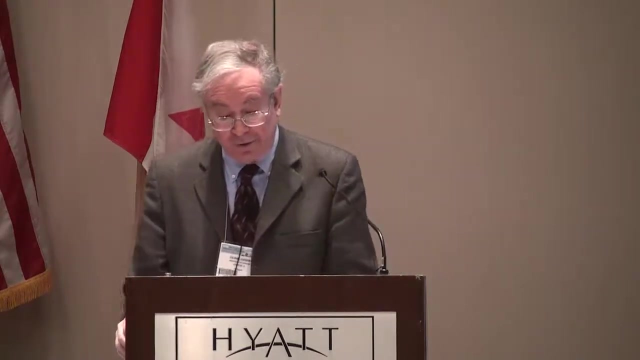 the connections between the real world and mathematical operations. While this has been done forever for some applications of addition and subtraction, with putting together and takeaway, even those ideas don't cover all the important uses of those operations and overall the connections are not discussed in a systematic enough way. 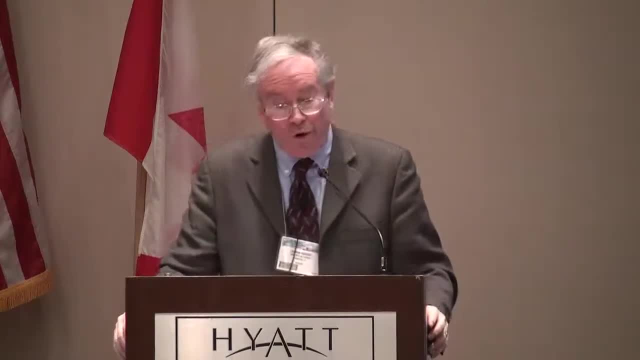 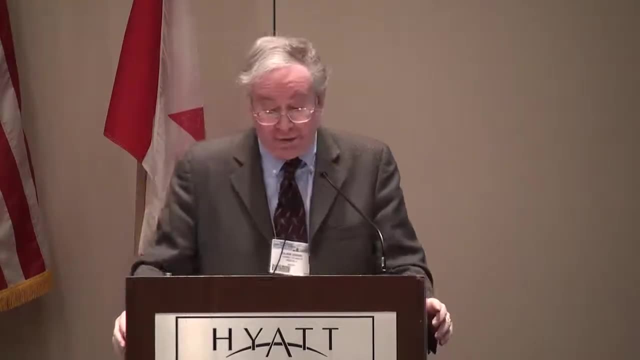 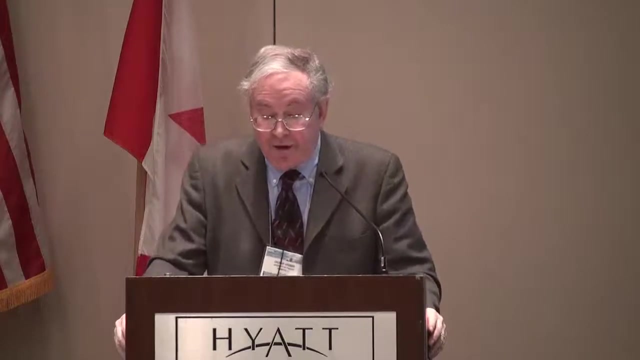 In this regard, the Common Core Standards can be viewed both as forward looking and backward looking. Applications are found throughout, from kindergarten on, though ironically they are found less in the standards for STEM students at the high school level as they are for all other levels. Thus those high school students 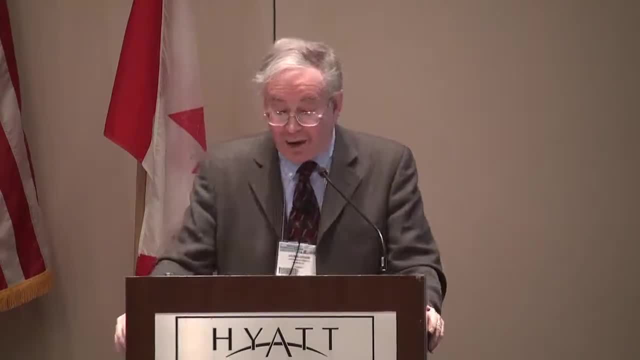 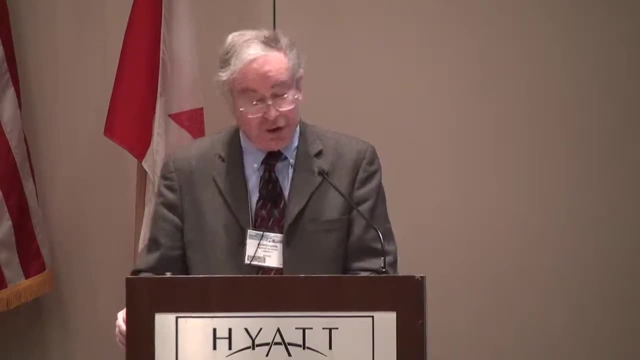 who might be most comfortable seeing how the mathematics they are studying can be employed in a wide variety of disciplines, and who we would want to encourage to go into STEM disciplines in a Common Core curriculum. these students spend less of their time on modeling and applications than their classmates. 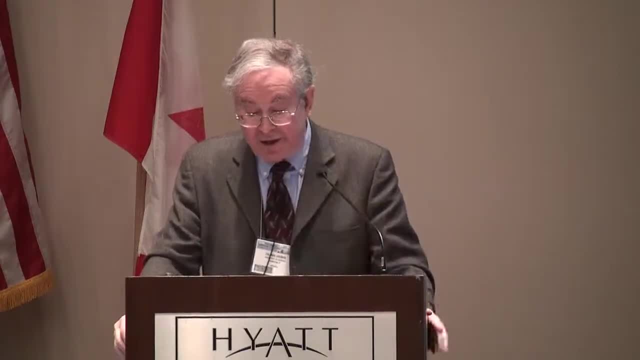 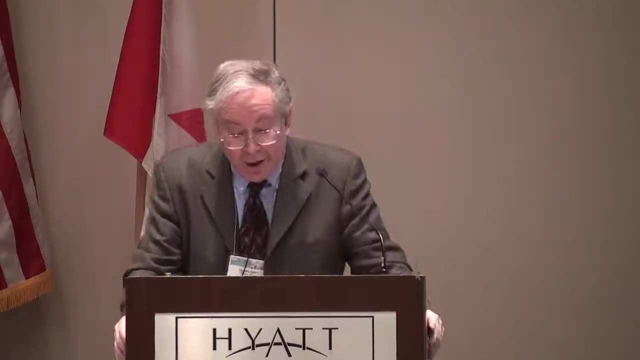 The Common Core reflects a weakness in many traditional curricula and can be seen again by looking at the modeling process diagram. I'm here restating an insight of Conrad Wolfram. Of the five steps in the modeling process, the one that can be done with technology automatically. 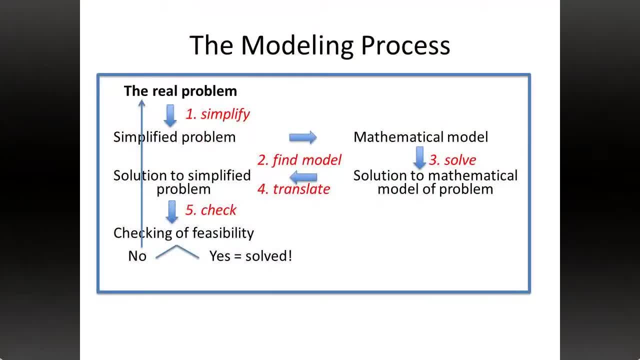 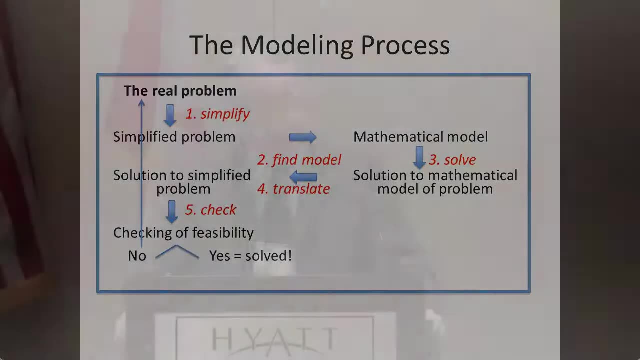 is step three, that is, working within a mathematical model to solve a problem. The other four steps: the simplification of a situation, the finding of the model, the translation of the solution, the checking of feasibility and deciding whether the problem is indeed solved. all those other four steps. 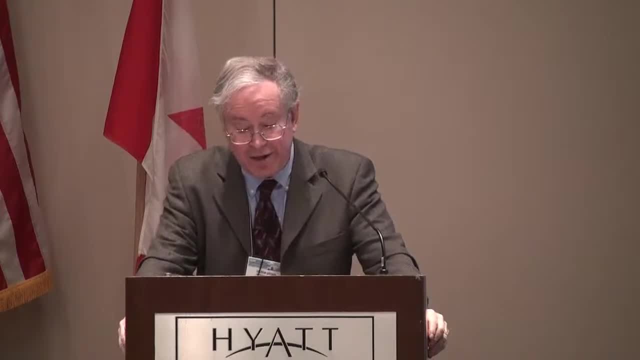 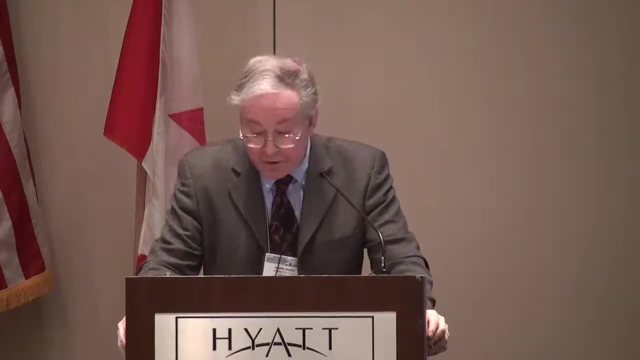 require human judgment. So many mathematics classes are spending almost all of their time working on step three, the stuff that computers can do better than humans. No wonder students ask why they have to study this mathematics If you're going to teach them to apply mathematics. 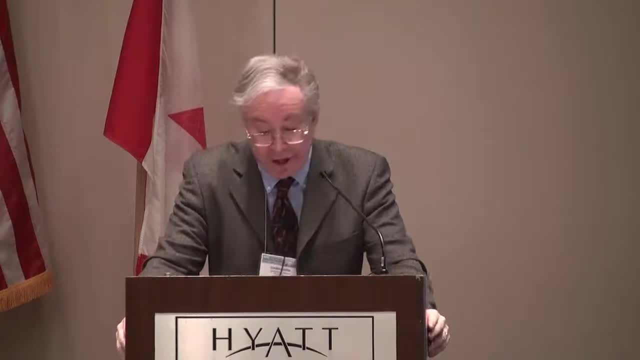 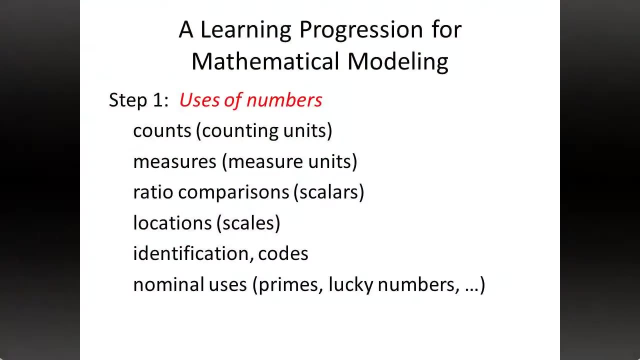 it's the other four steps where you should be spending a lot of your time These days in common core standards. there's much rhetoric about learning progressions, that's the move from one grade to the next, and so on. So here's a learning progression. 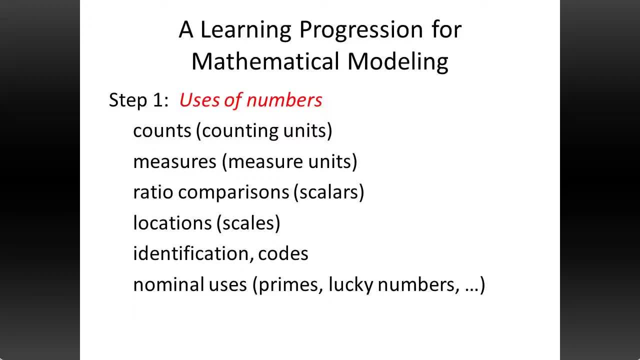 with respect to mathematical modeling, We begin with uses of numbers. in primary school, we expect that students have seen numbers used as counts and measures and these uses. we don't just deal with numbers, we deal with quantities. quantities are numbers and their units- Counts have counting units. 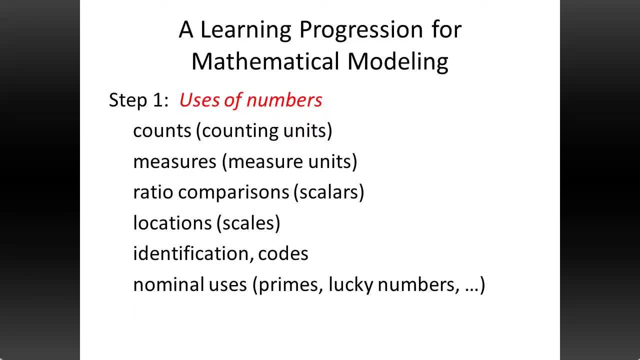 measures have measure units When the negative numbers arise. this occurs very early. we know it can be done with first and second graders, although it doesn't occur in the common core until grade 47 or something like that. I think it's grade 6. it's just silly. 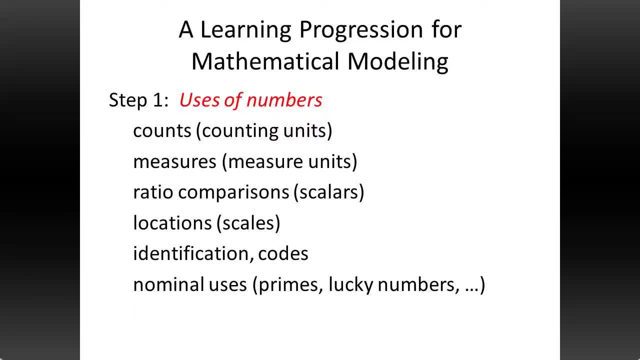 Fractions and percent show that numbers are also the result of ratio comparisons, and such numbers don't have units, they're scalars. Pi is a wonderful example of an irrational number that is, by definition, a ratio comparison. a scalar Numbers also represent locations, street addresses, rank orders. 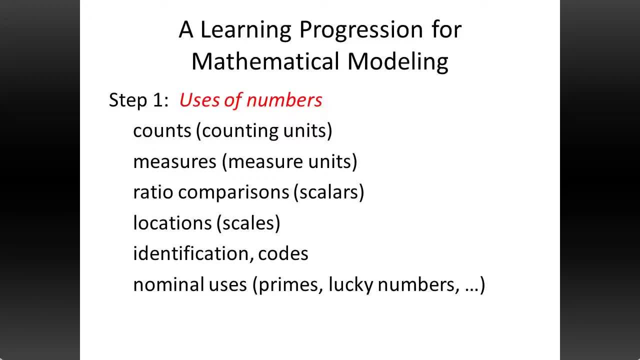 and scales such as the Celsius scale or the decibel scale for sound intensity. they represent the fourth use of numbers scales. Numbers may also be used for identification in codes, as in charge card numbers, or as ISBNs, and of course they're numbers simply used as numbers. 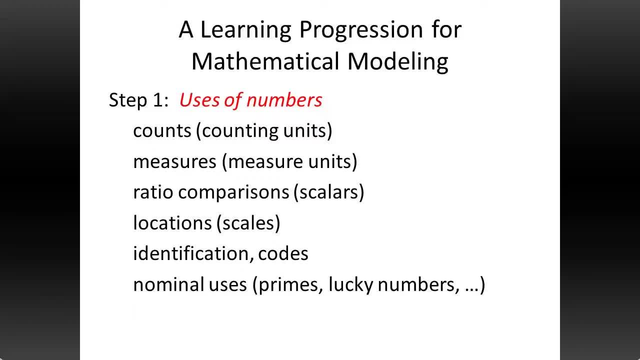 nominal uses, such as when we examine prime numbers or lucky numbers. The uses of the operations of arithmetic are some, but not all of the uses of numbers. The sum x plus y has meaning if x and y are counts or measures, but not necessarily when x and y. 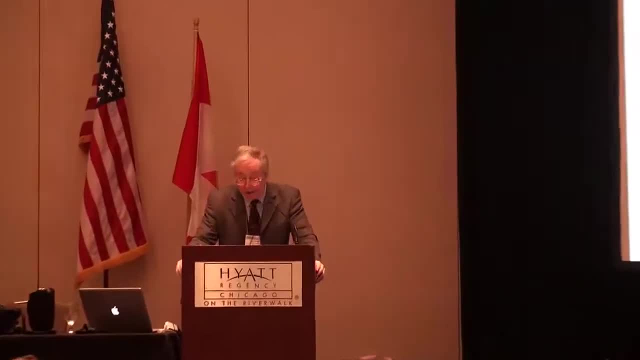 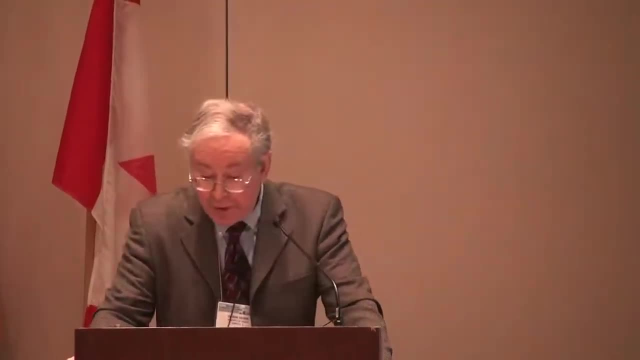 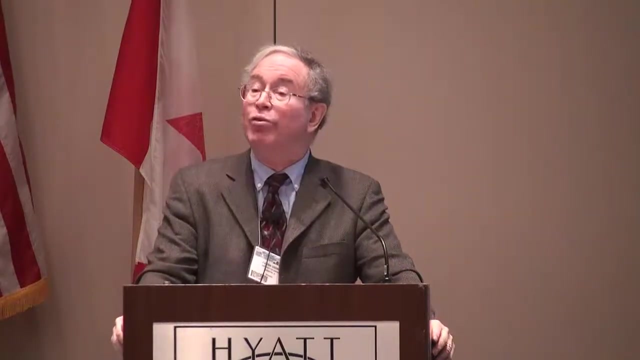 are ratio comparisons, and almost never if x and y are codes. You don't add the scales of two maps, nor do you add telephone numbers. Also, when x and y are locations, the sum x plus y doesn't have much meaning. For example, the sum of two addresses. 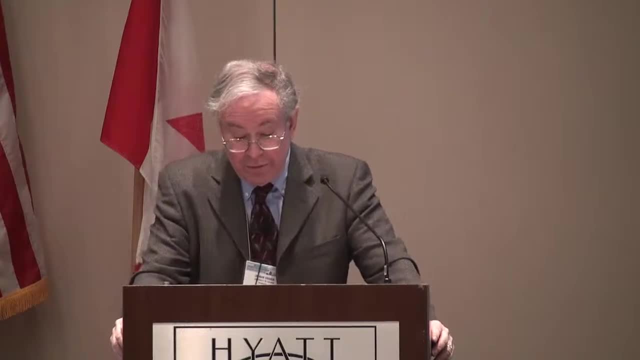 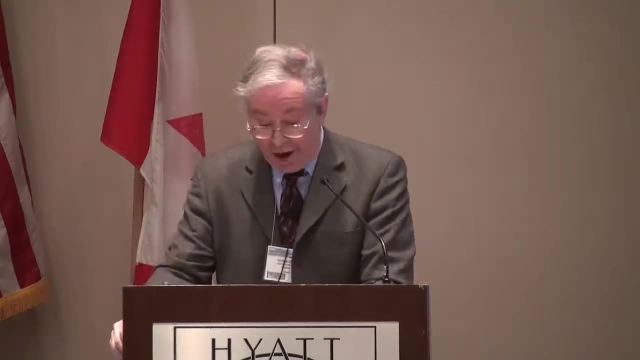 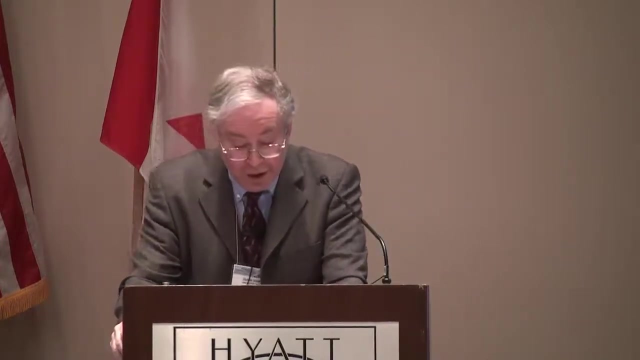 doesn't have too much meaning. Yet in these very same contexts, other operations may have meaning. The difference x minus y of two temperatures almost always has a meaning. In Chicago, the difference of the addresses of two houses on the same street can be used to approximate how far those houses are from each other. 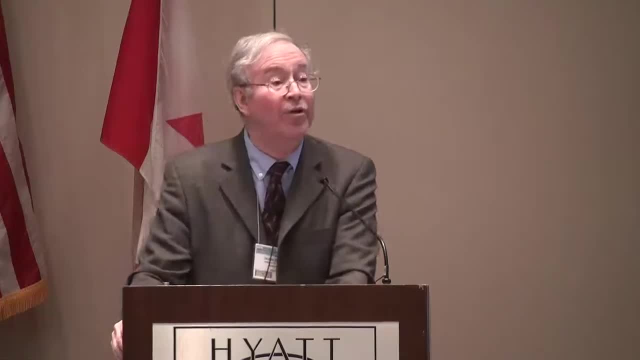 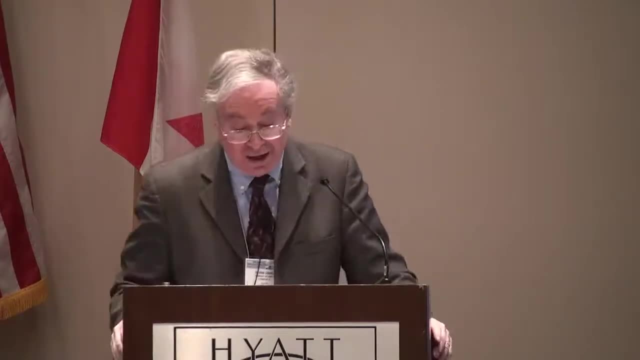 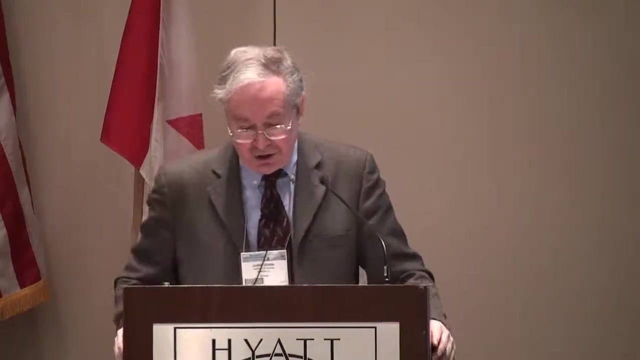 even if they're miles away, because we know 800 numbers is a mile in most parts of the city. Two scales may be multiplied to get the result of applying one scale after the other. Each of the operations has fundamental meanings. This is the second step. Addition is putting together a slide. 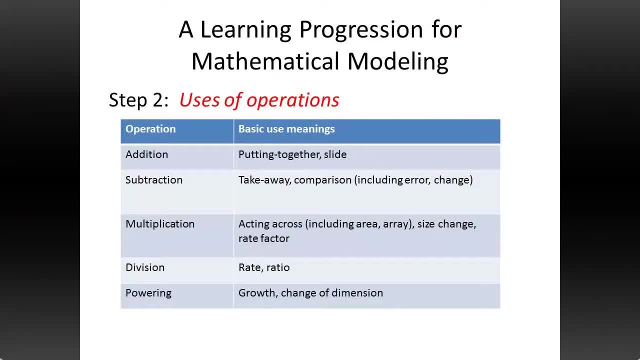 Subtraction is take away or comparison, and special cases of comparison are error and change. Multiplication is acting across, including area and its discrete counterpart being array. How many are there in an array? What's the area of a rectangle? Size change or rate factor? Division is rate or ratio. 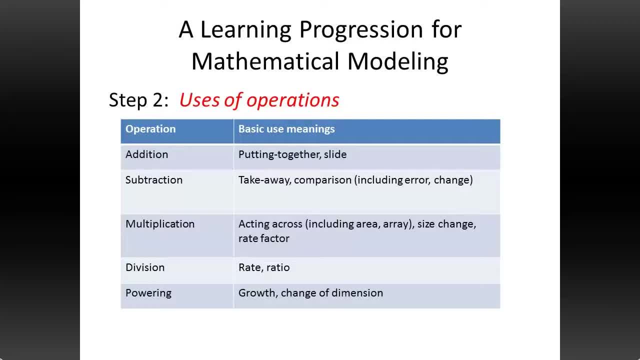 Powering is growth or change of dimension. The applied meanings are related to each other just as the abstract meanings are. For example, take away undoes putting together, Just like subtraction undoes addition, Size change undoes ratio, Just the way, or they're related in the same way. 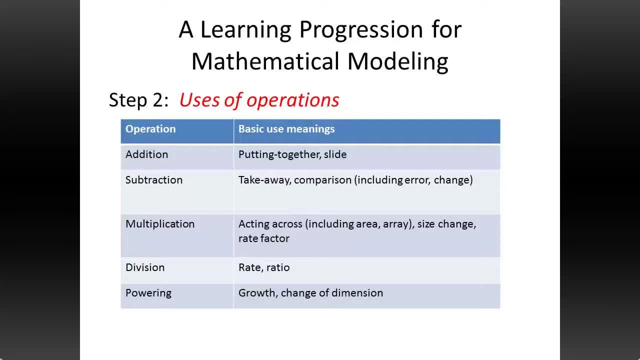 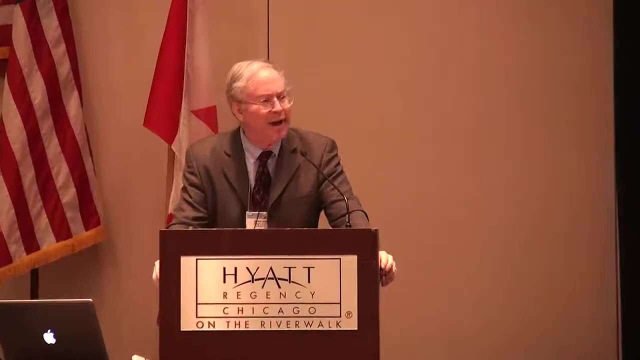 as multiplication and division. Allow me a true story about what happens when people do not understand the relationships between uses of numbers and uses of operations. I was reading a magazine called Light Metal Age. This was not a magazine about some rock groups who were not into heavy metal. 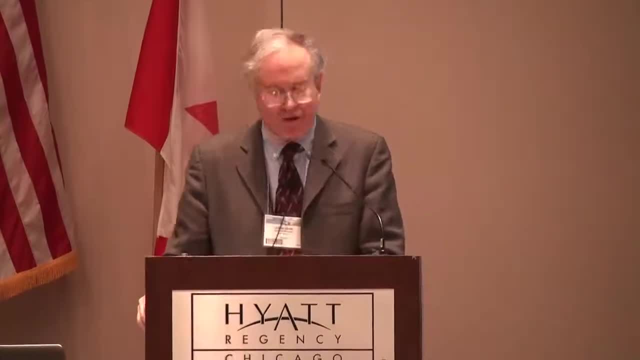 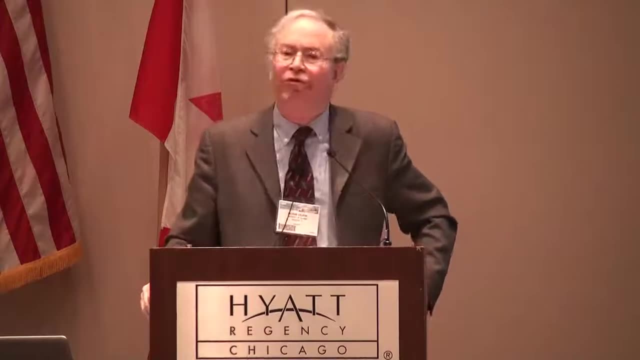 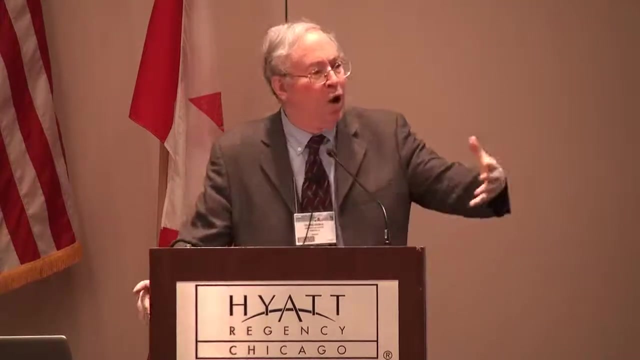 It is a magazine devoted to the production and fabrication of materials such as aluminum and titanium. The gentleman and I struck up a conversation and I found out that he worked for Alu Suisse, the aluminum company of Switzerland, The Switzerland equivalent of Alcoa. He had written an article. 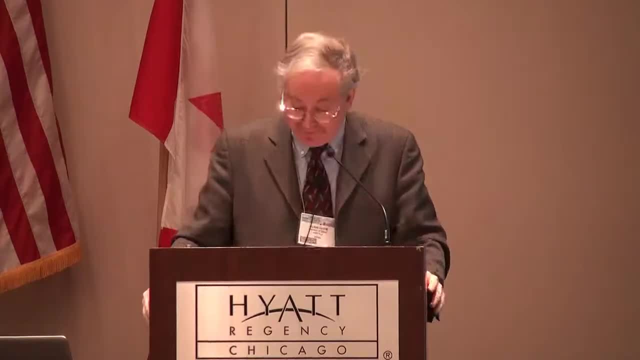 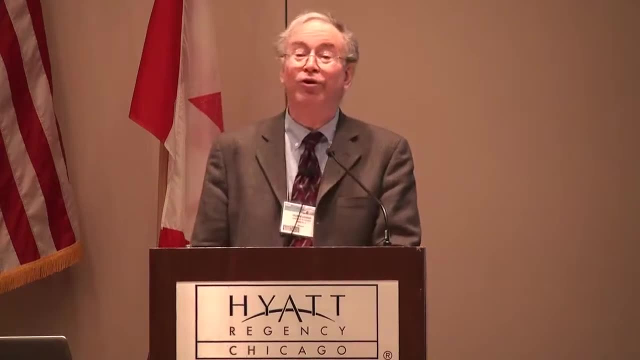 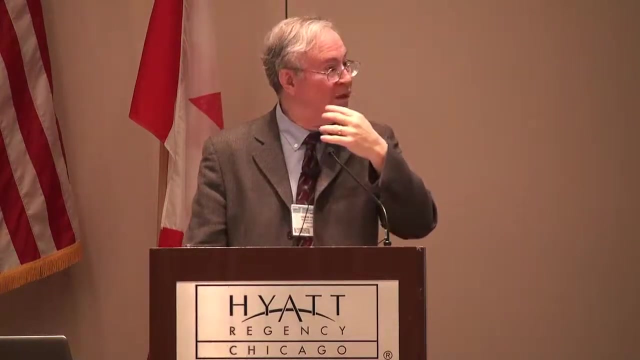 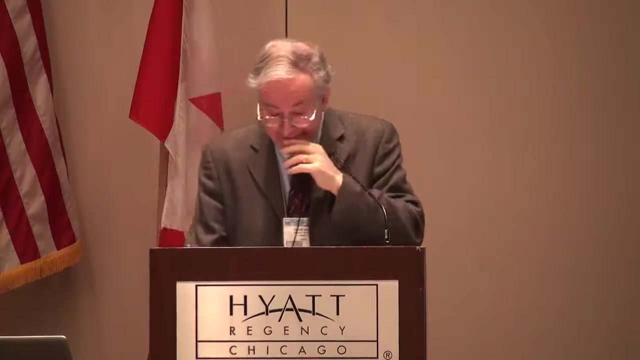 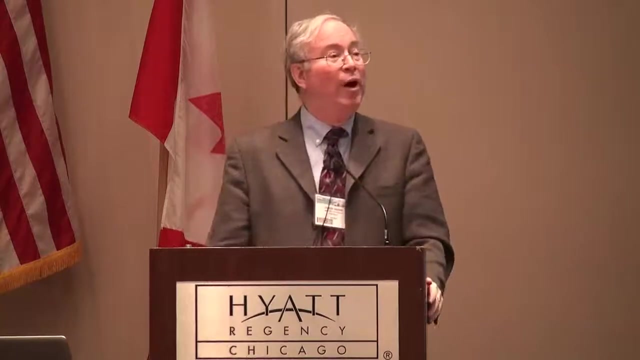 for the European counterpart of Light Metal Age and he was now reading the English translation. This translation included, as you might expect, the conversion of metric units into our customary units. Did I Just the mention of metric? In one place? he noted an error in the translation. A particular process with aluminum. needed to be done at a particular temperature with a 5 degree Celsius leeway. So the question became: what's the Fahrenheit equivalent of 5 degrees Celsius, Instead of realizing that temperatures are scale values and a difference of 5 degrees. a difference of 5 degrees. 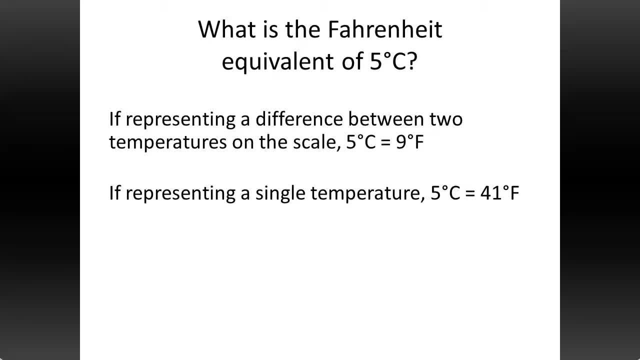 Celsius is equivalent to a difference of 9 degrees Fahrenheit. You know there's 9 fifths or 5 ninths in the formula. The difference of 5 degrees Celsius was interpreted as 41 degrees Fahrenheit. Imagine a company thinking. Imagine a company thinking that it had so much leeway. 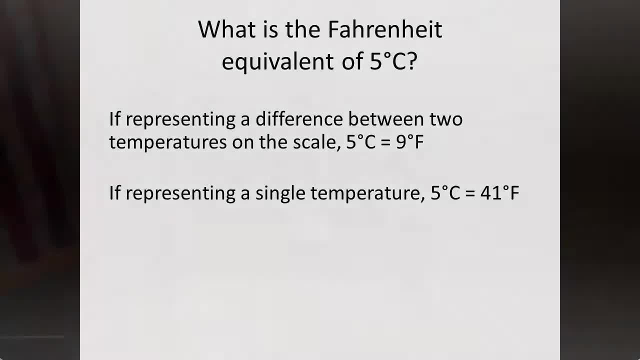 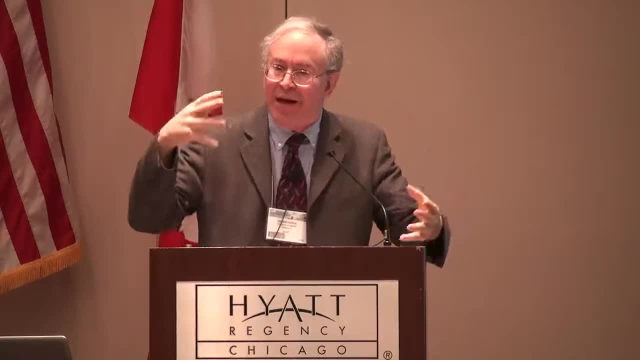 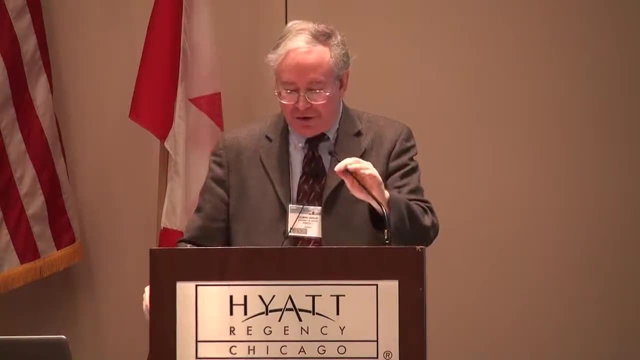 in its production temperature, only to find out that the translator had no values, as if they were measures. So this notion of scaling and scales is very important to teach students, Whereas the units of measures are usually ignored in the formulas students see in mathematics classrooms. they help to distinguish. 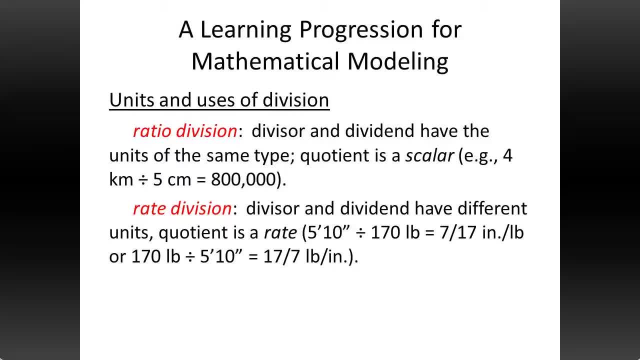 the various meanings of operations. Ratio division is when the divisor and dividend have the same units and we say the units cancel and the divisor and dividend have different units. For instance, divide my height- 5 feet 10 or 70 inches- by my weight, 170 pounds. 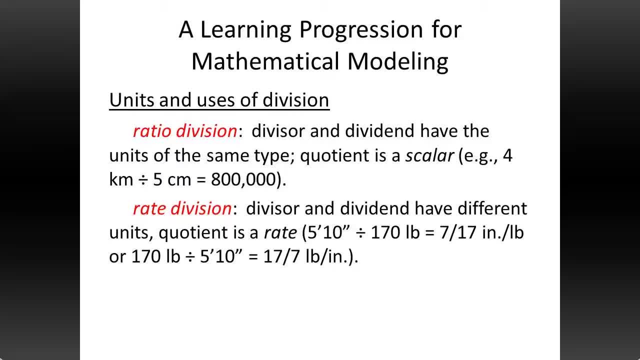 and you get a rate either 7- 17ths of a pound per inch. take an inch- 7 17ths of a pound and divide the other way and you get an equivalent rate- 17- 17ths of a pound per inch, or I should not have used 7 and 17. 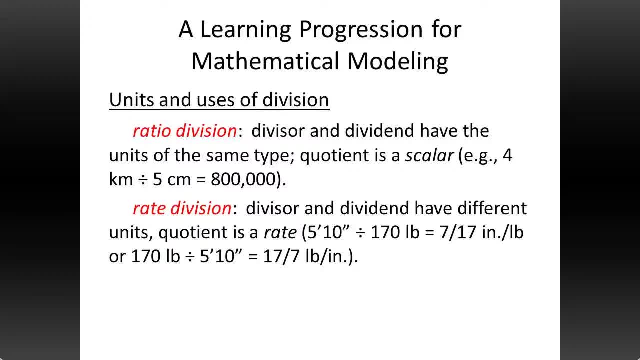 but what could I do? The numbers are messy. I'm not exactly 5'10 and my weight is not exactly, But you get the idea. The quotient is a rate and it's important. you can do it either way, Or consider multiplication With area or acting across multiplication. 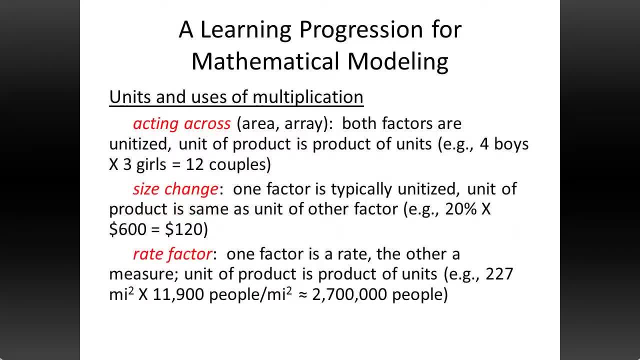 the units multiply to create a product unit. 4 boys times 3 girls is 12 couples. That's a different unit. Inches times inches is square inches. kilowatts times hours is kilowatt hours. With size change. the magnitude of the size change is a ratio comparison. 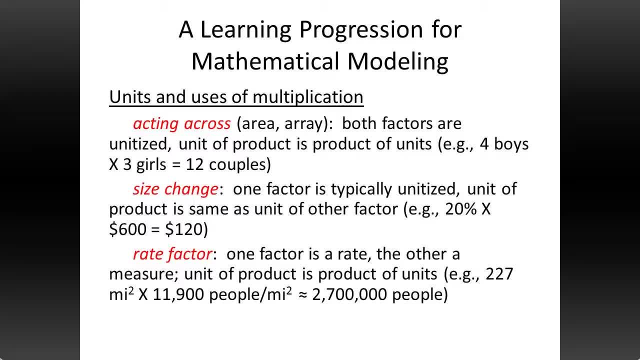 It's a scalar. This magnitude is multiplied by a measure and the result is a measure with the same unit as in 20% times $600 is $120. Some people wrongly think the percent is a unit. It's not a unit, It's a number name. 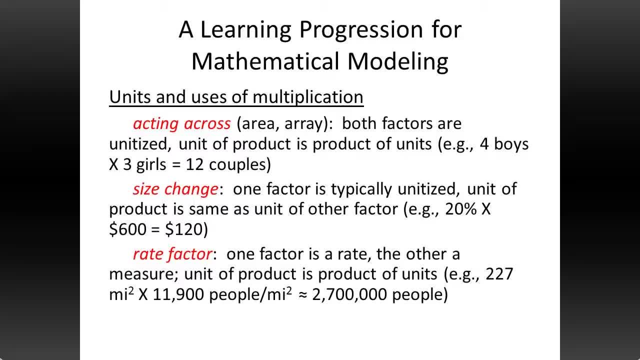 like million or billion. In rate. factor multiplication is a rate and the units multiply. For instance, Chicago has about 11,900 people per square mile. This is a rate people per square mile multiplied by Chicago's land area about 227 square miles, and you get a good estimate. 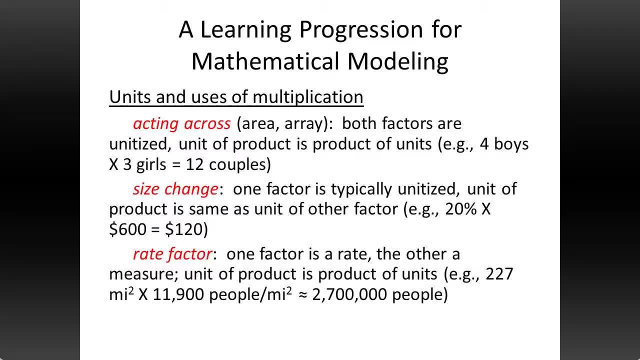 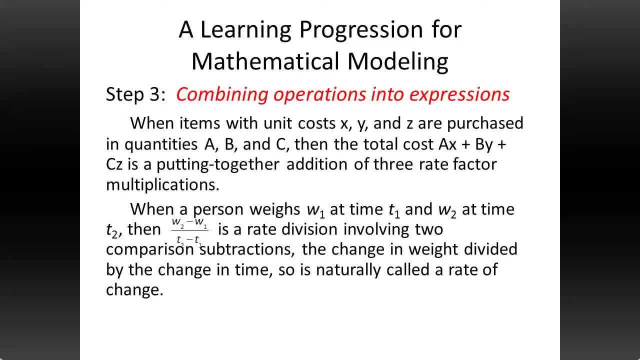 of Chicago's population, namely about 2,700,000. As a learning progression, it's fundamentally important that in the primary school these uses of numbers and operations go beyond counts to include non-integers, to give meaning to algebraic expressions, For instance when items with unit costs. 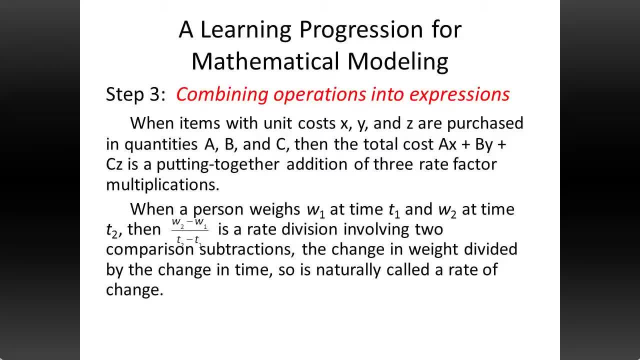 X, Y and Z are purchased in quantities A, B and C. the sum AX plus BY plus CZ is in addition putting together rate factor multiplications to arrive at a total price. You have three rate factor multiplications. you put them together in the addition. 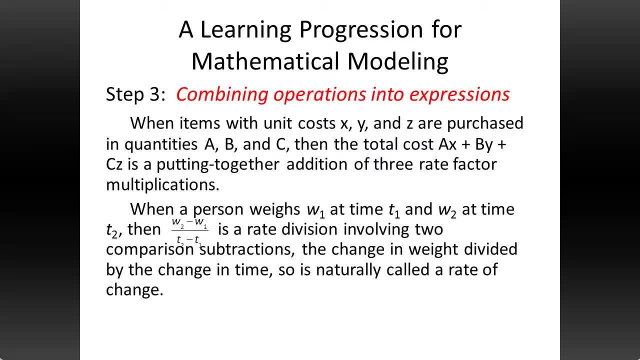 The calculation of rate of change of a quantity two different times. Here I took weight, the change in weight and the change in time, this calculation. so you have a comparison subtraction, two comparison subtractions, and you want the rate, the rate of change. you divide and so rate of change. 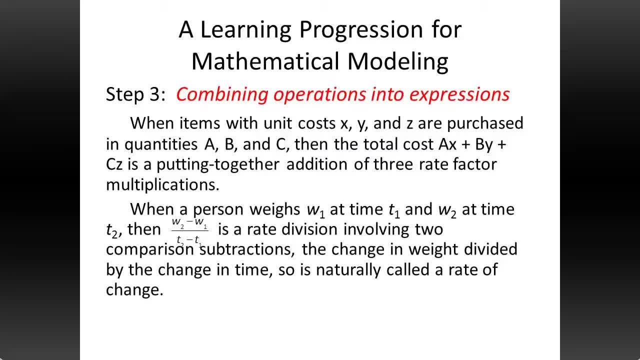 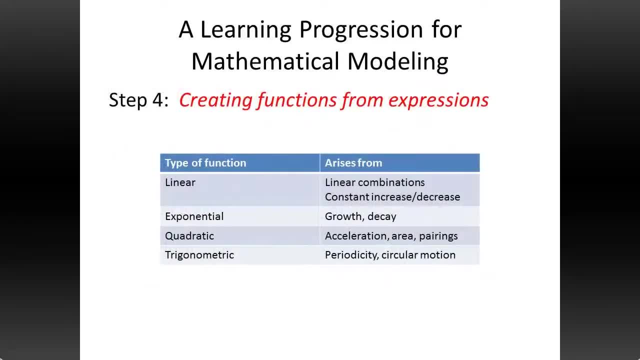 should precede slope because it's so natural. out of the operations- and you see what the slope formula means, From the meanings of algebraic expressions- come the situations that functions- model Linear functions- arise from linear combinations: Constant increase or constant decrease. Exponential functions, as we know in all books, have this. 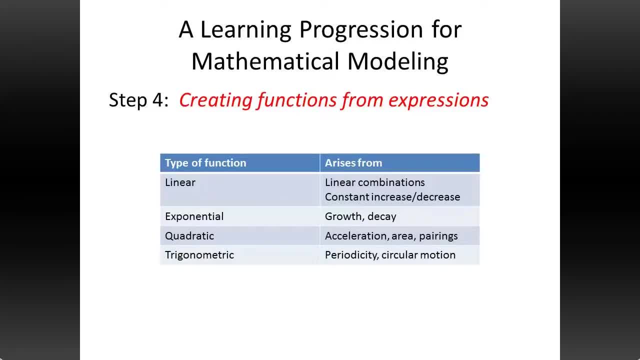 they model situations of growth or decay. Quadratic functions: model situations of acceleration or deceleration. Acceleration is a rate, of a rate that's how you get the square or area again, giving you squares. Trigonometric functions model circular motion, often quite appropriate in situations. 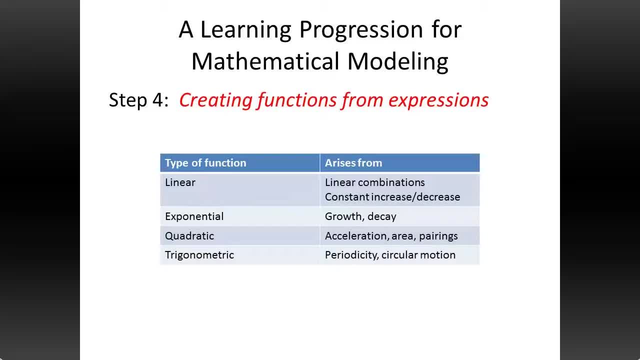 where phenomena occur periodically, The broad kinds of situations, various kinds of functions, model should be as much a part of the curriculum as the mathematical properties, the situation, the translation. how do you get the model? that's really fundamental, For it's almost certain we would not be studying. 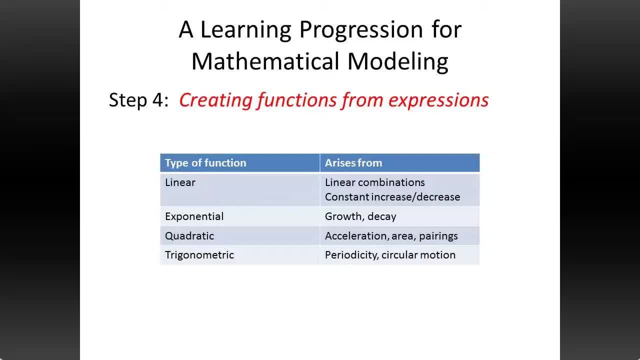 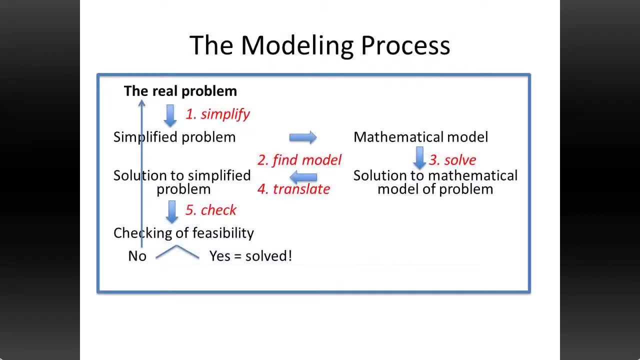 these functions were it not for their applications. Let me go back to the these learning programs, back to the modeling diagram. Obviously, the pivotal step in mathematical modeling is to find the model, to find the mathematics that fits the particular situation In classical mathematics. this task has been dealt with. 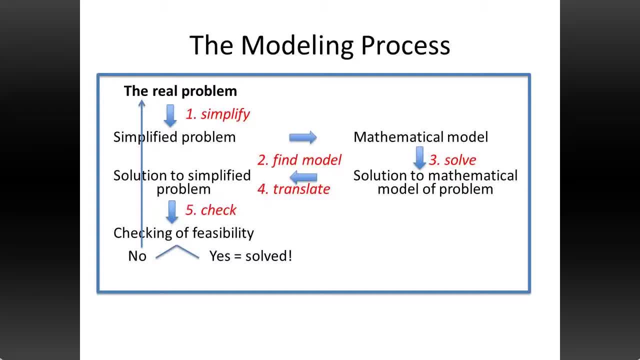 by translating words describing the real situation into mathematics. This is why applications are so often characterized as word problems. We have enough experience to know that this way of teaching modeling has very limited value. Word problems are highly stylized. Applications are typically not restricted to a particular style. 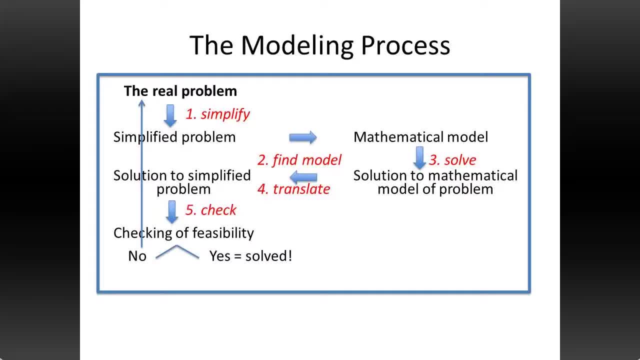 They may not have any words in it, They may just have pictures, and so on. Consequently, the finding of a mathematical model allows the student to recognize that a facet of the application situation is modeled by a corresponding facet of the mathematical idea or operation. To do this, the student needs a repertoire. 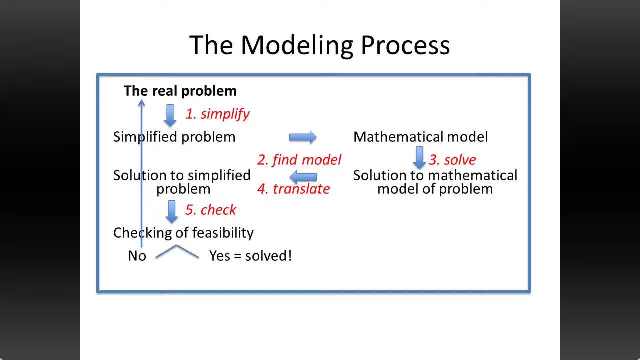 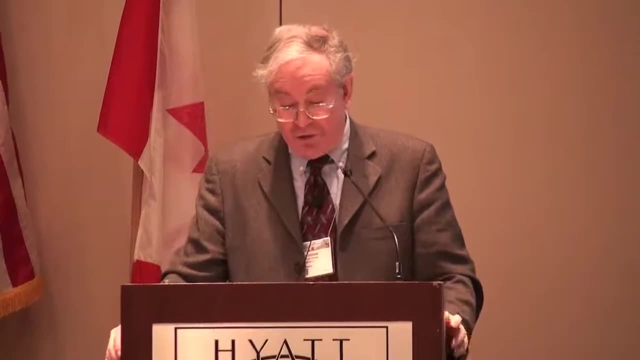 of the basic use ideas of the mathematical concepts. In turn, obtaining that repertoire requires that when a mathematical concept is being taught, the student be introduced to its major uses. In fact, many curricula that teach mathematical modeling often introduce a mathematical concept or mathematical idea by starting from a use. 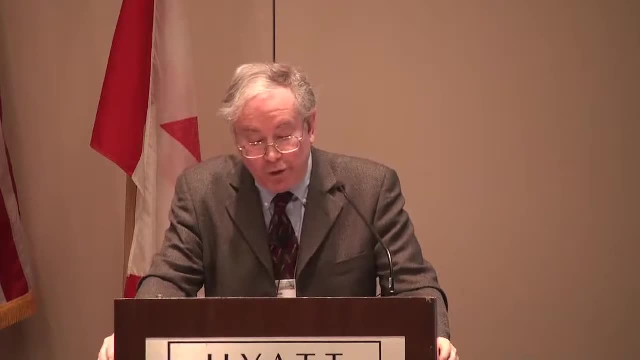 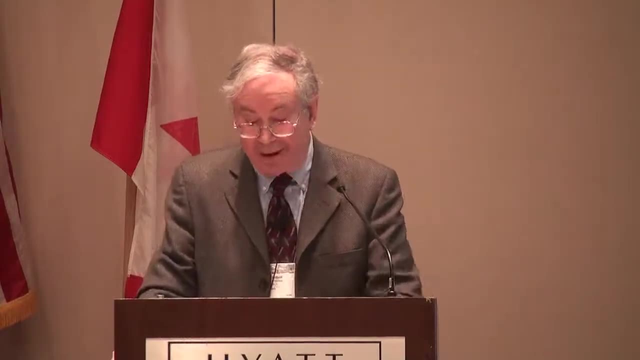 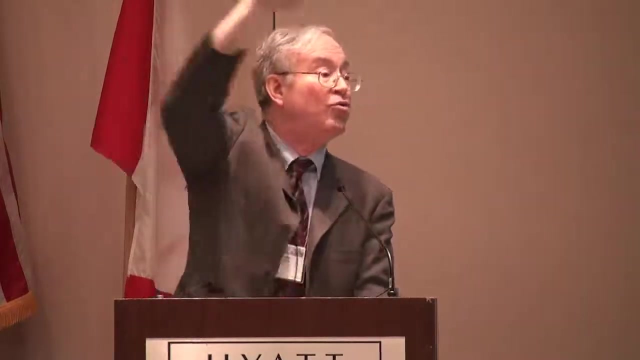 So, even though in this diagram the mathematical modeling process goes from the real world situation, starts with the real world, then goes to its mathematical counterpart, In order to teach mathematical modeling we must go in the reverse direction and study the basic uses of each mathematical idea, so that a student knows. 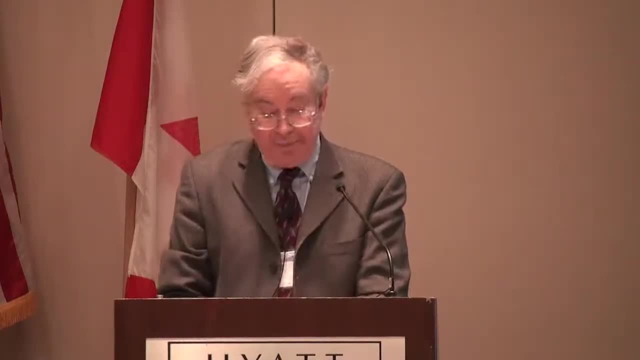 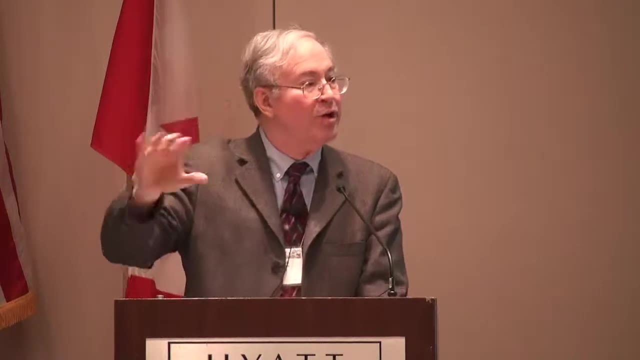 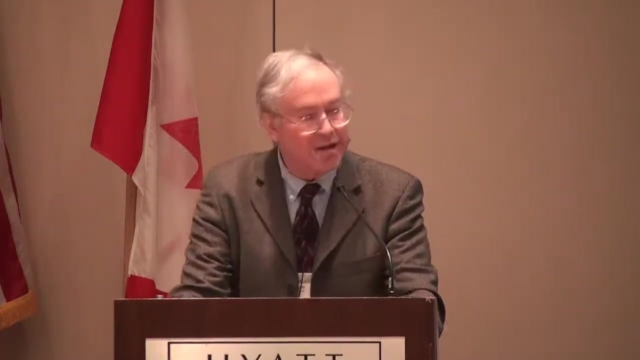 what they might connect the real world to. So you have to go the other way. The most important mathematical ideas have more than one basic use, So you want to teach multiple uses of the ideas. After finding a model, the next step in the modeling process is solving the problem. 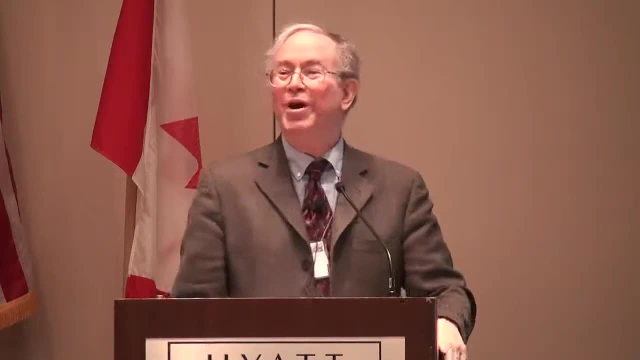 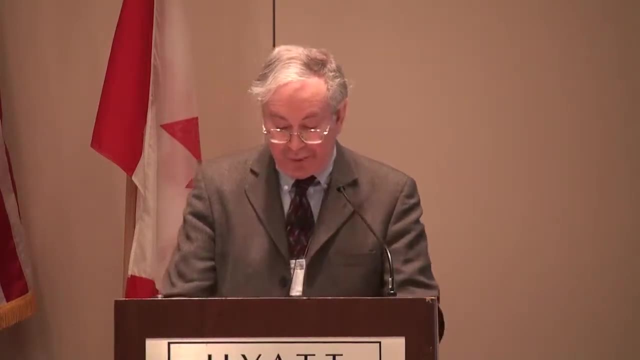 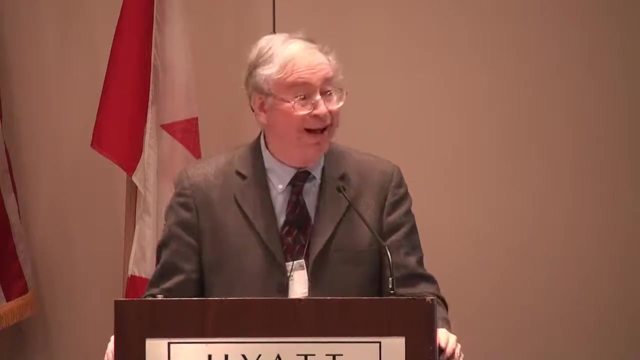 as it has been restated in its mathematical model. Some people call this doing the math. This is a difficult step for many students because in most classrooms in the country, students are solving the problem in the mathematical model to practice some mathematical idea. If they really wanted to know the answer. 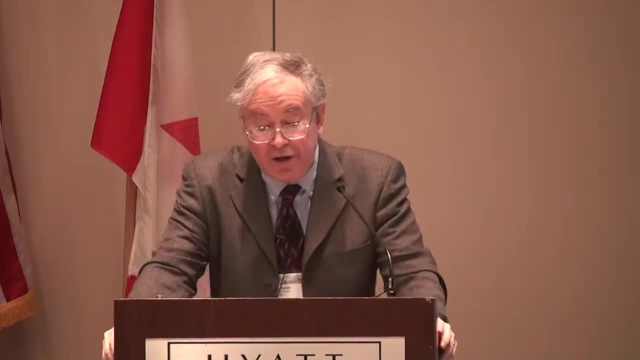 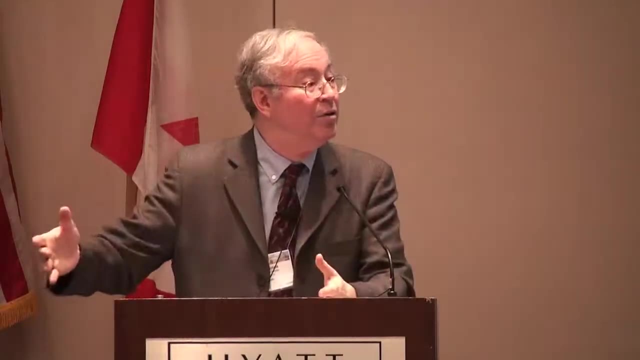 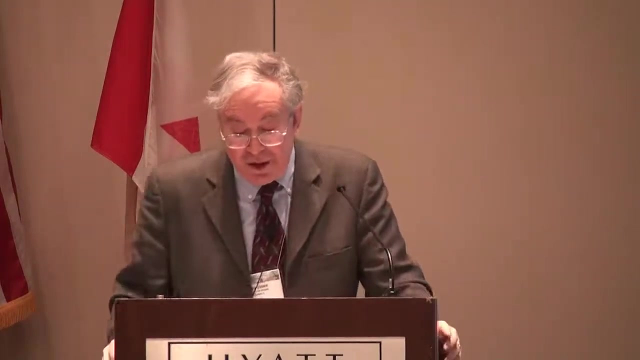 they might really be motivated. The application has not been there because it's important, even when it is important. it's been there so they can practice computation, practice solving an equation. We know that the purpose is to practice some mathematical technique, because in the real world people use any technology they can. 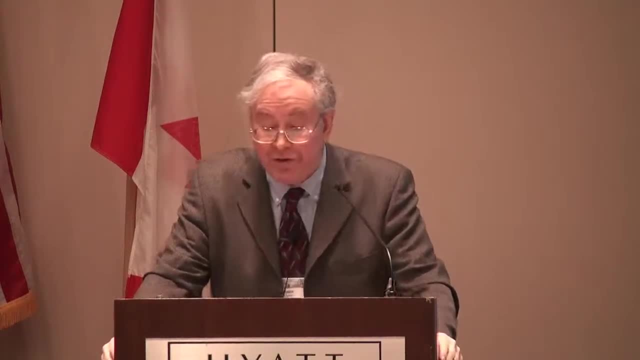 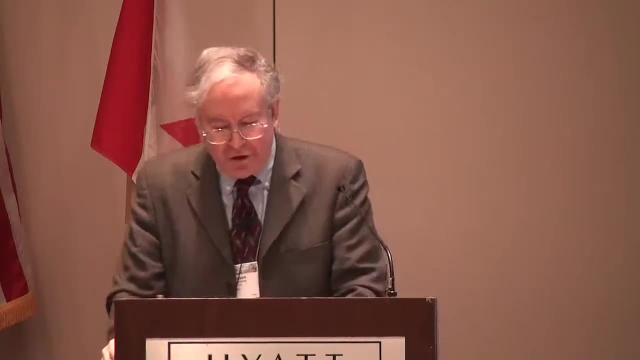 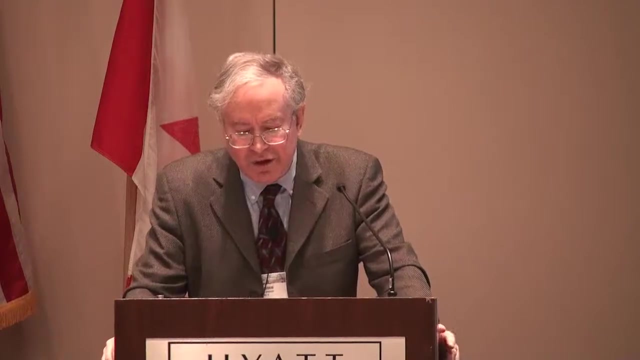 to solve a problem. But in the classroom in the United States technology is cheating. It isn't cheating at all, It's wisdom. All of this talk in the Common Core Standards about fluency, that is, speed and accuracy, is totally misguided. If you want fluency, today you use a calculator and computer. 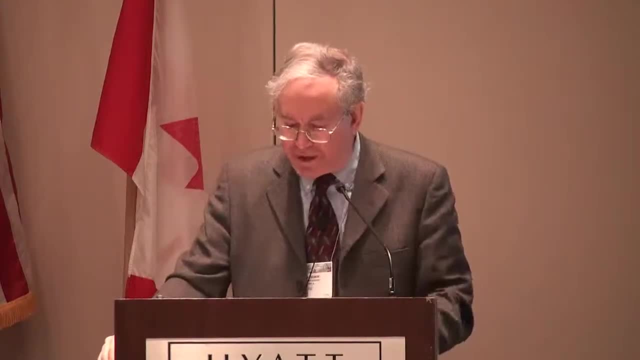 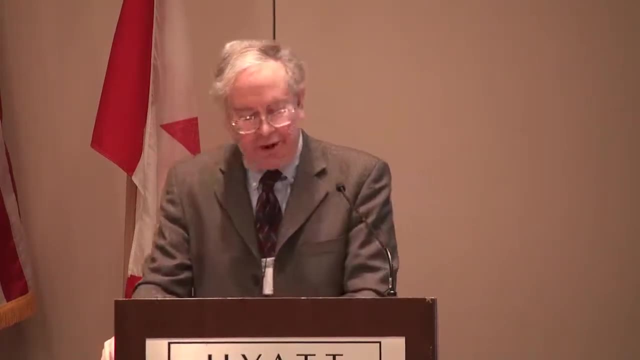 When do you see cashiers in a store use paper and pencil to add up how much it will cost you? When does the person who does your tax returns use paper and pencil when working on your return? Would you gain or would you lose confidence in the results they got? 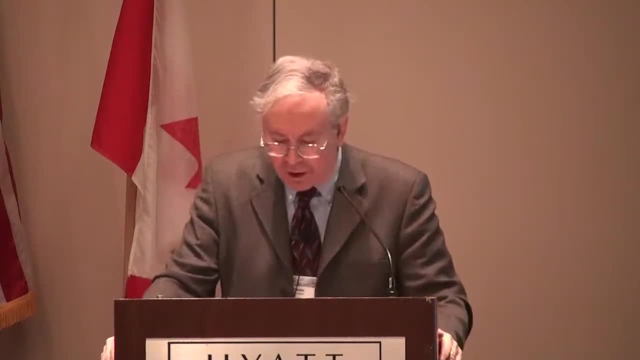 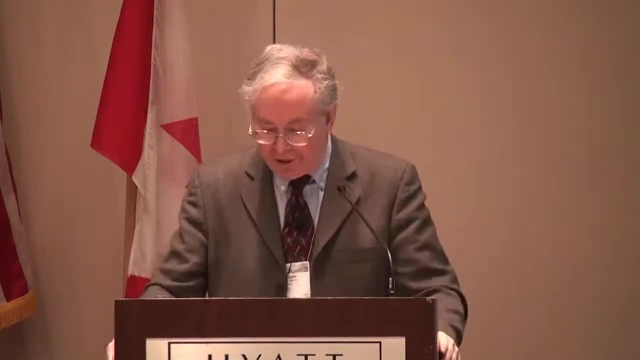 There is not one mention of calculators in grades K-8 in the Common Core, and the use in high schools is limited to complicated expressions or explorations, not to the actual doing of everyday mathematics. This view is the opposite of the view towards technology in the real world. 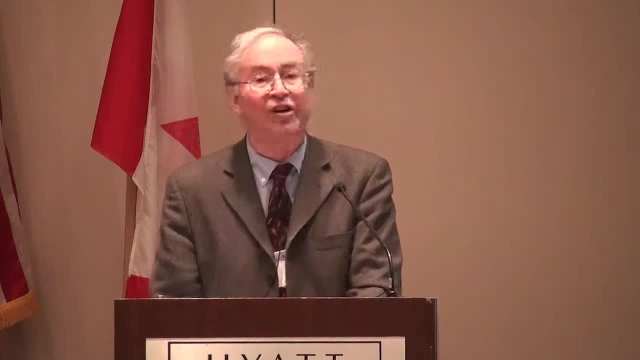 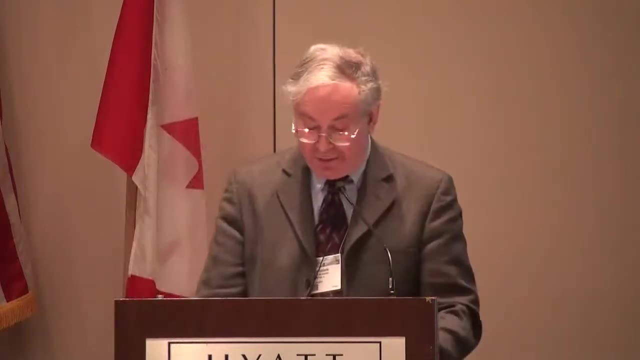 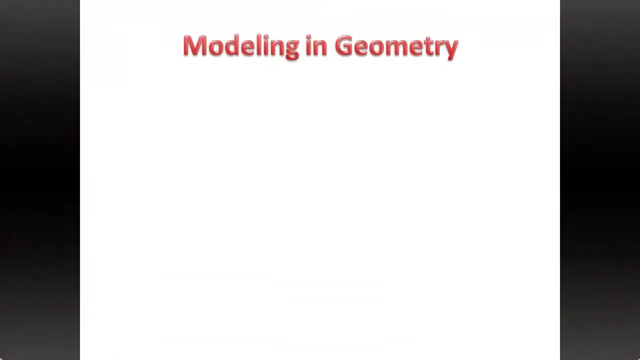 and it's just the opposite of what we need in this country to prepare students for today's workplace, let alone tomorrow's. So far, my examples have mainly been from arithmetic and algebra. Let me turn now to geometry. How does geometry fit into all this? Very nicely, it happens. 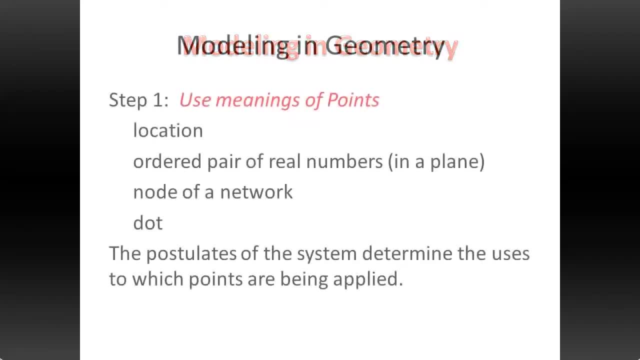 In geometry, the basic notion is the point. Point is, in most deductive systems, an undefined term. This is not a weakness of mathematics but a strength, because undefined allows point to take on a variety of meanings. In particular, a point may be a location, an ordered pair, ordered triple. 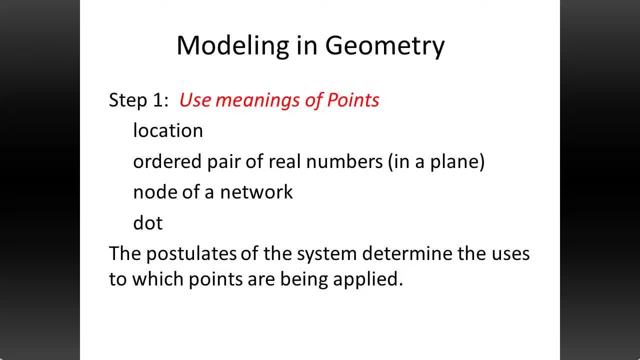 or even an ordered n-tuple of numbers, a network or a dot. These notions of point are as basic as the uses of number. and just as uses of number lead us to uses of operations and uses of expressions, so uses of points lead us to uses of lines. 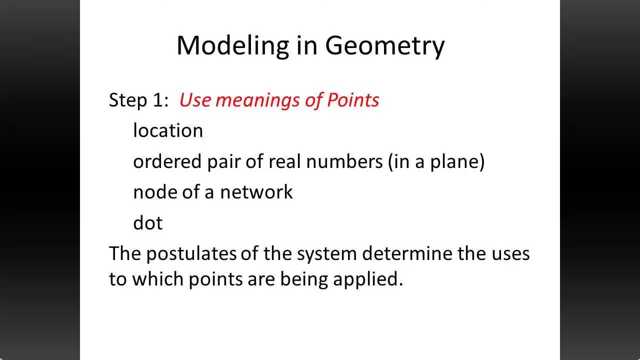 and other geometric figures. We might view discussions of these notions as the first step in a learning progression of modeling and geometry, but by this I do not mean that it should occur in that order. Undefined term is an advanced concept compared to the uses of geometry. It might go in the same order. 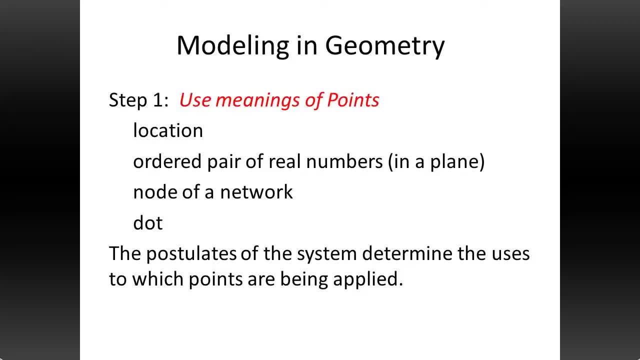 you might go to in arithmetic. The mathematics of these various kinds of points is different. That is the basic reason why we have postulates. The postulates tell us what kinds of points and lines we are dealing with. For instance, there is the postulate that two distinct points determine a line. 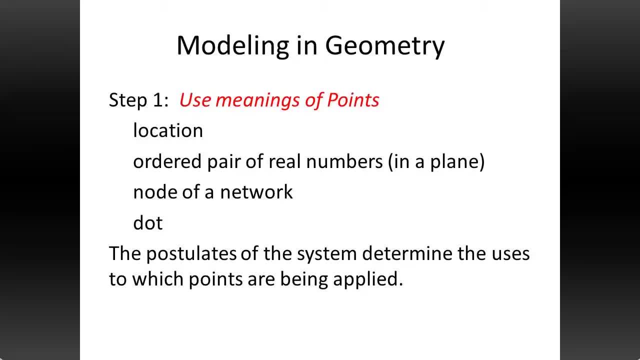 That is, there is exactly one line through two points. This postulate holds for thinking of points as locations or as ordered pairs, but it doesn't hold for nodes and networks, where you might have many paths connecting two nodes, and it doesn't hold for dots, because the dots have some width. 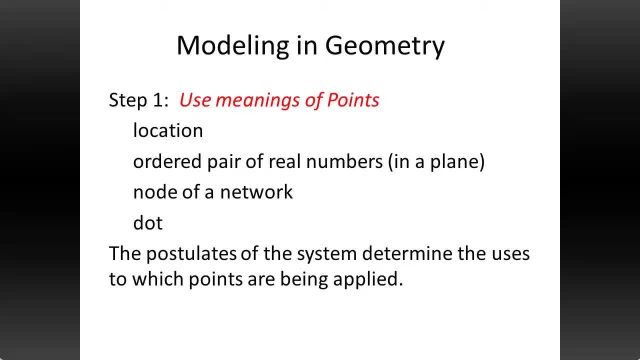 and you might have a number of lines connecting dots. I needn't say much about the application of points as locations, the most common application of geometry to objects in the plane or in space. We can describe these points also by ordered pairs or ordered triples. The postulates of plane Euclidean geometry. 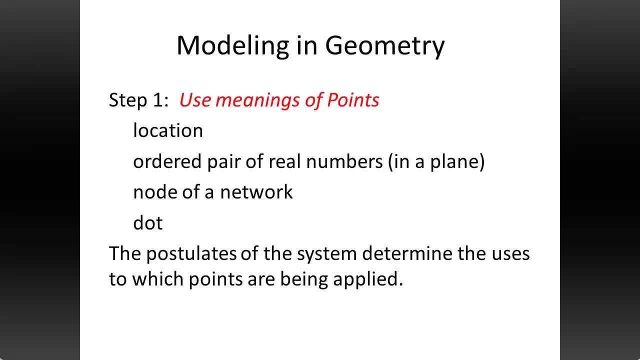 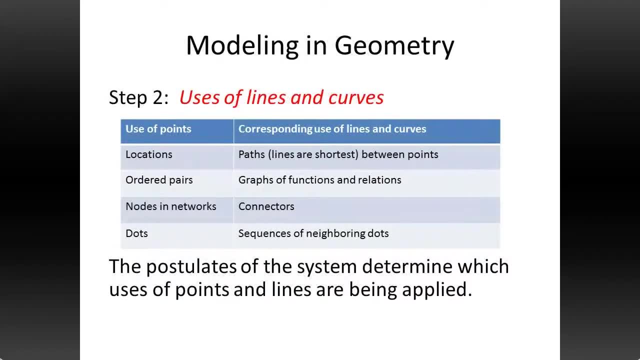 fit our notion of point as location and also as ordered pair in a rectangular coordinate system. In other words, we move from number to operation, so we can move from point to line or curve. Lines contain paths of shortest distances between points and are subject to the postulates. 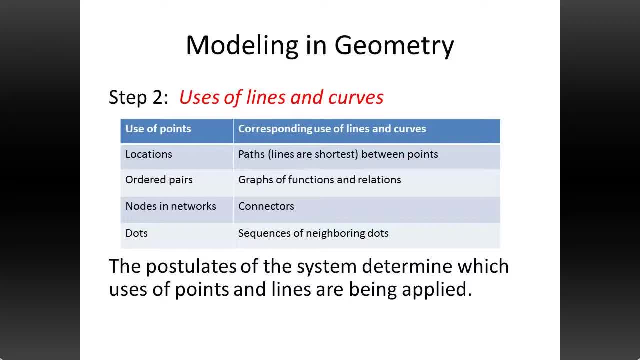 that connect points and lines. Curves contain other paths connecting points. We model objects by looking at their physical features and emulating those features in the models. we study Points as ordered pairs or ordered triples or ordered n-tuples. also have applications different from locations, In particular data points. 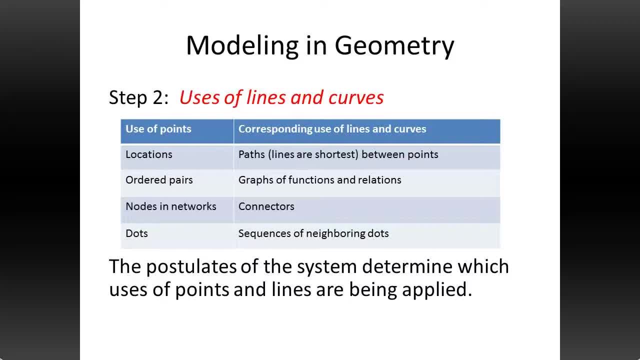 We often want to consider lines that fit these data points. As locations, we're limited to two or three dimensions, but data points we're not limited at all and n-dimensional points have some meaning. Most of our geometry in school is done in the plane. There's a subtlety to considering an ordered pair. 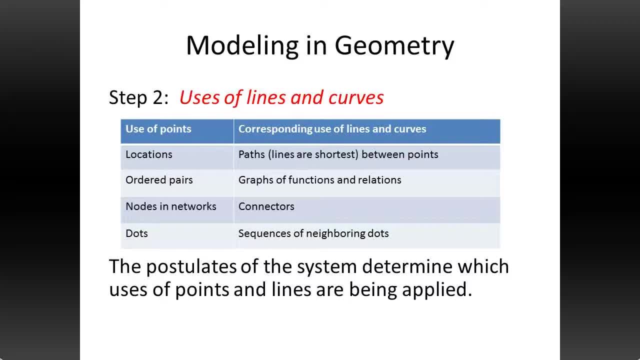 of real numbers as a conception of point, The graph of a function from the reals to the reals- The typical graphs we most study in school- or the graph of a function. The graph of sets of ordered pairs now is a geometric object, not just a representation of a function. 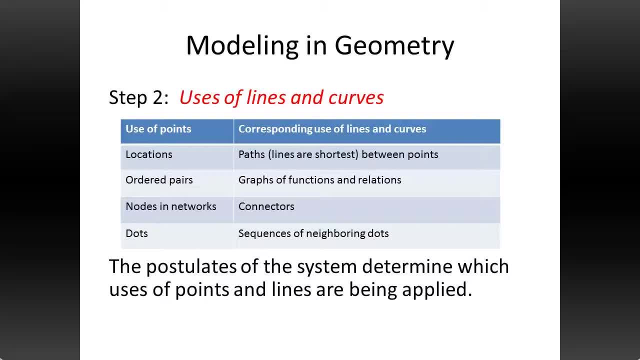 So it has all the mathematical properties that we associate with lines and curves. So, for example, we can think of the graph y equal x squared. We can think of that. that is a parabola. It's not just a representation of the function, It is a geometric object. 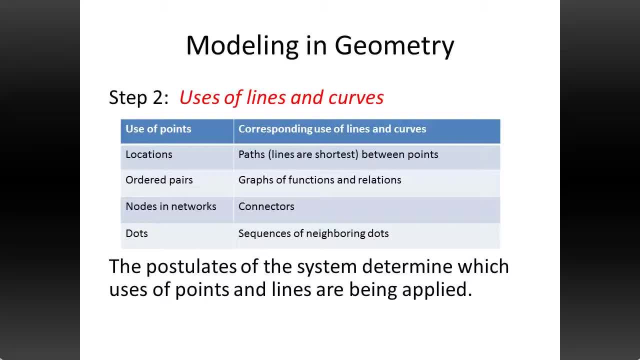 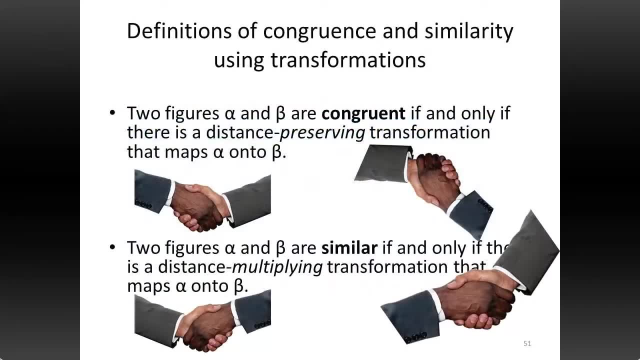 Here the common core standards are a great help. By prescribing the definitions of congruence and similarity in terms of transformations, They've opened the door for any figures to be considered in geometry, Not just triangles, other polygons and circles. So, for example, these hands shaking are all similar. 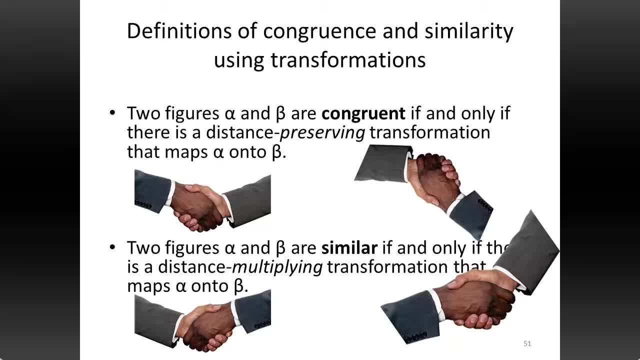 And three of them are congruent. I think it's pretty obvious which three should be the congruent ones, But it might not be obvious to you that the one on the bottom is congruent and the one on the bottom left is congruent to the one above it. 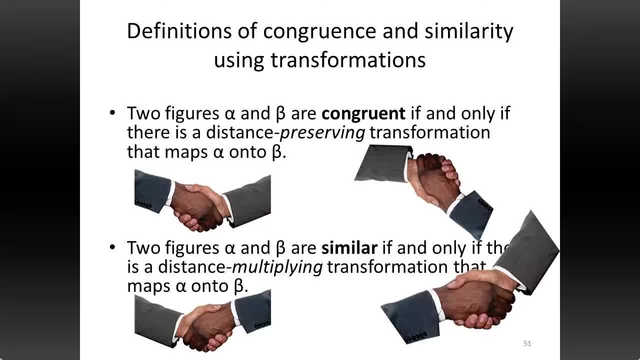 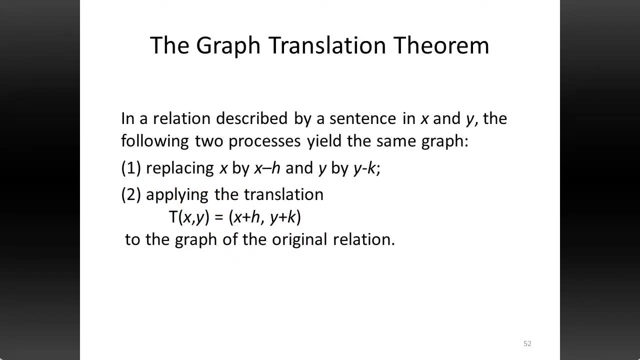 It is. It's a reflection image. It's a glide reflection image. These are the definitions of congruence and similarity. These are definitions in terms of transformations, which is what the common core would like students to learn, With the general conception of congruence and the ability to consider sets of ordered pairs. 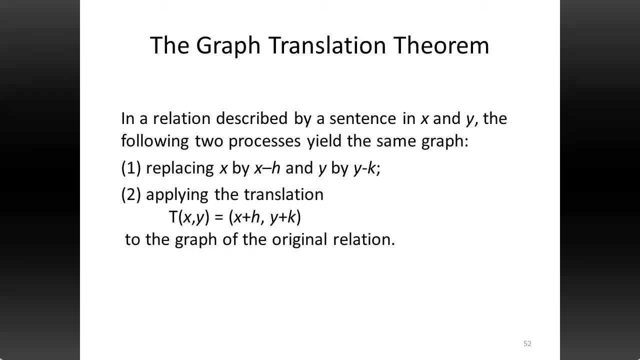 as geometric figures. we can have theorems about graphs. One of these that is exemplified in many of today's books is called the graph translation theorem, although it's seldom except, I think, in the UCSMP books- called the graph translation theorem. It's just there. 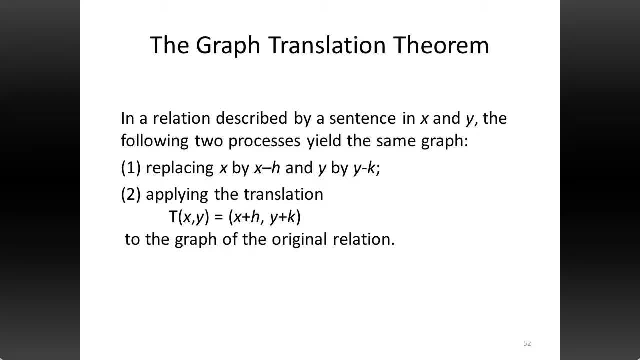 Because they don't want to call it a theorem, because theorems are supposedly only in geometry. What nonsense. But here it is, In a relation described by a sentence. in x and y, these processes, you can substitute x minus h for x or y minus k for y. 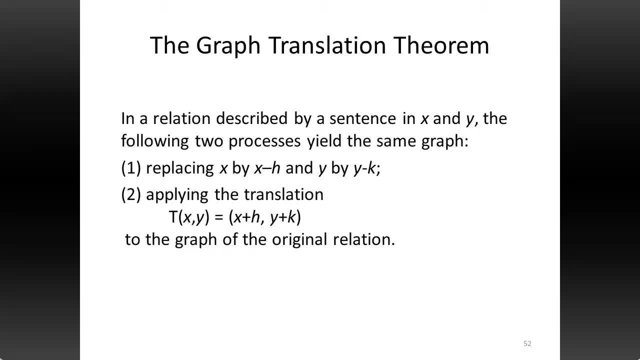 and the result in the graph is: if h is up or if h is negative, it's to the left and if ku is negative, it's down. From this theorem- it doesn't look like it's modeling, but I'll get there- From this theorem we can easily deduce: 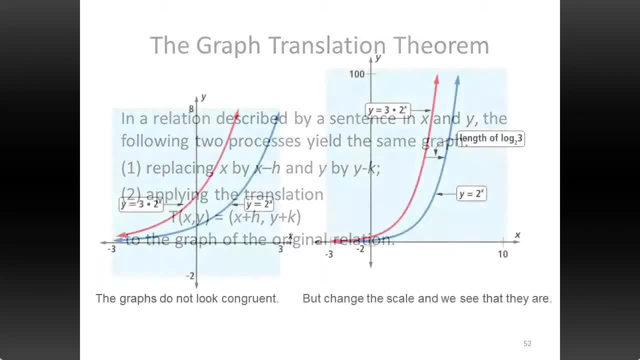 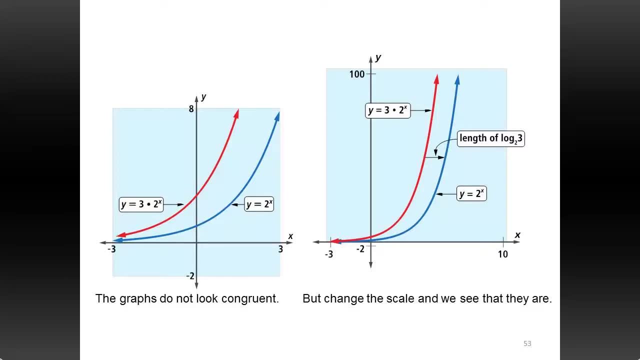 that the graphs of any two exponential functions with the same basis are congruent. Consider, for example, the graphs of y equal 2 to the x and y equal 3 times 2 to the x. It looks different on the left when we do our usual thing. 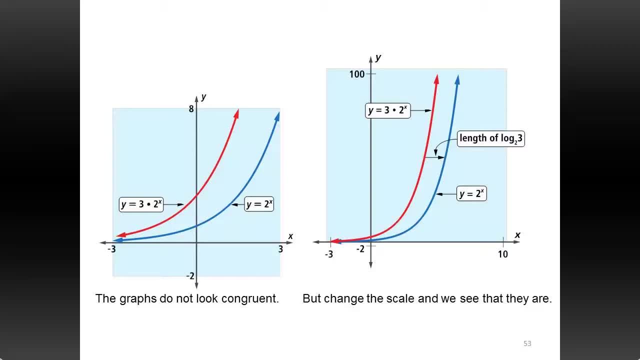 where we just go from negative 3 to 3 right around the origin, we see that, in fact, the blue graph is a translation image of the other graph. These, in fact, are simply the same kind of growth, starting at a different point in time, Instead of starting with one dollar. 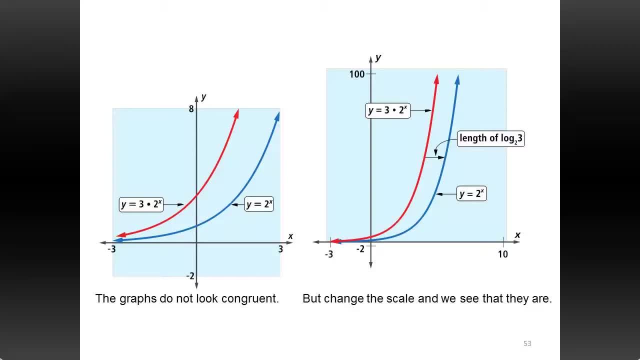 you start with three dollars. and the reason? we can prove this using logarithms: because 3 is a power of 2, 3 is 2 to the log of 3 to the base 2, and therefore y equal 3 times 2 to the x. 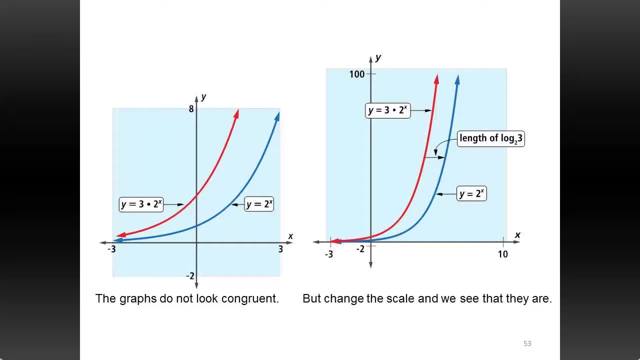 is y equal 2 to the x, plus log of 3 to the base 2, which means it is that much to the left. so it's very nice if you have, and any two exponential functions with the same basis are congruent. so it means that 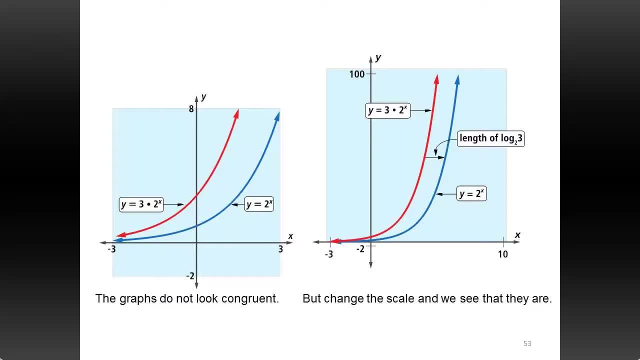 if you have doubling, ultimately all money that doubles. if your money doubles and it's negative where you started, it will ultimately have a certain time frame behind the other. so, for instance, if you won the lottery this week- I'm sure many of you did- you're just ahead of us. 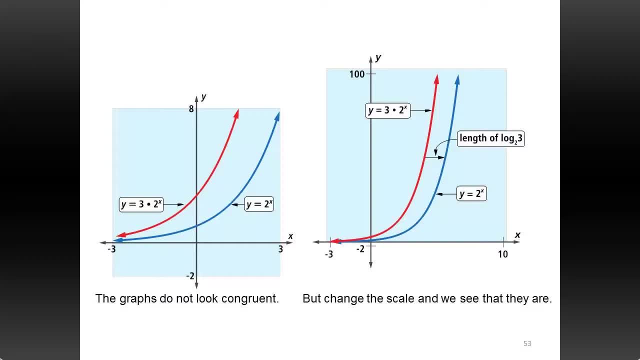 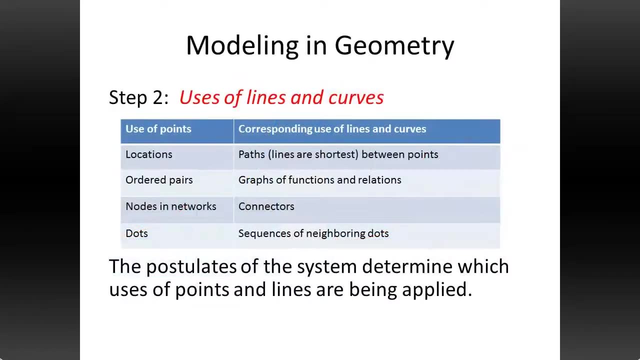 those of us who are struggling with smaller amounts to double, we'll catch up. The point as a node of a network is different from the point as a location or as an ordered pair of numbers. The postulates are not the same for networks. There may be two or more lines through the same two points. 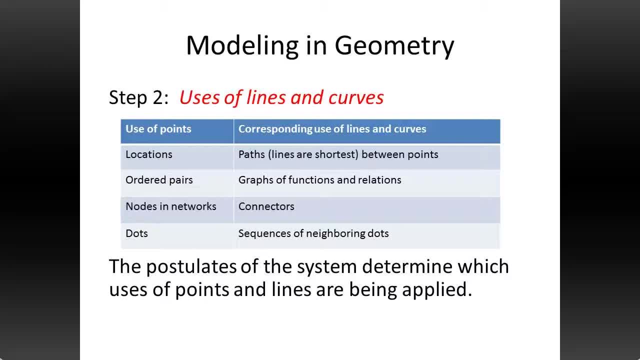 for example. but there's still rich geometry here, started by Euler with the and studied mainly in topology. A fourth conception of point, that of a dot, may rankle some of you. A dot isn't a point. you may say it's a representation of a point. Yes, a dot is a representation of a point. 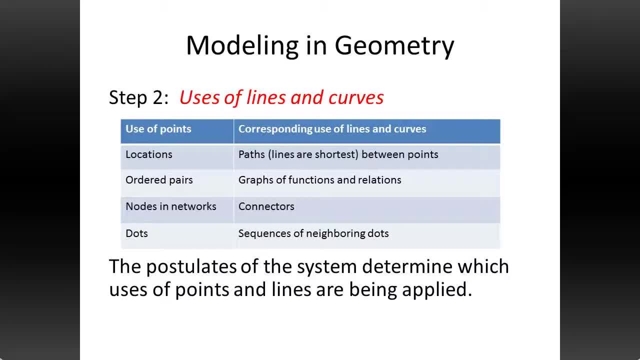 when the point is thought of as a location, but it's a very useful thing to think of a plane as a union of dots In the screens of our televisions, computers and handheld devices. we call these points pixels. Both of here is probably the most famous piece of art applying this conception. 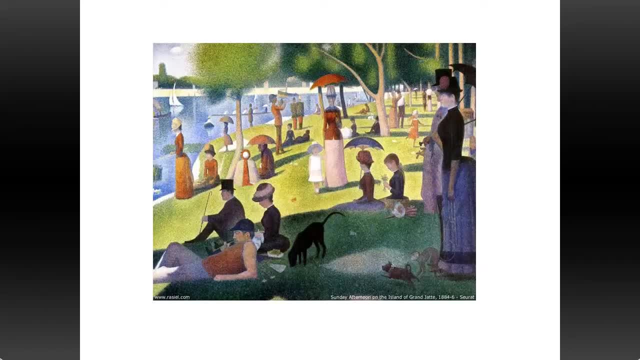 Seurat's large canvas Sunday afternoon on the island of La Conchette. Painted 125 years ago, it's approximately 7 feet high and 10 feet wide- about the size- and was done in the style that artists call pointillism. Again, the geometry is different. 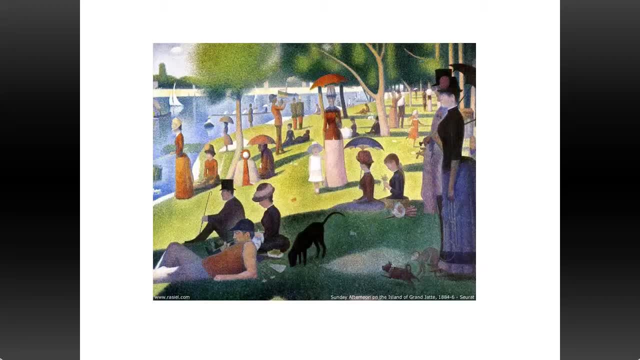 because between two points there may not be a third point. Knowing these alternate conceptions of points shows us that it's not only Euclidean geometry but other geometries as well, and notice how connected geometry and algebra become and how the notion of a mathematical system, with its postulates, definitions and theorems. 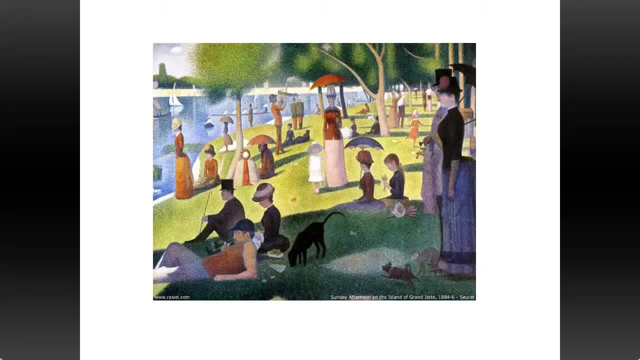 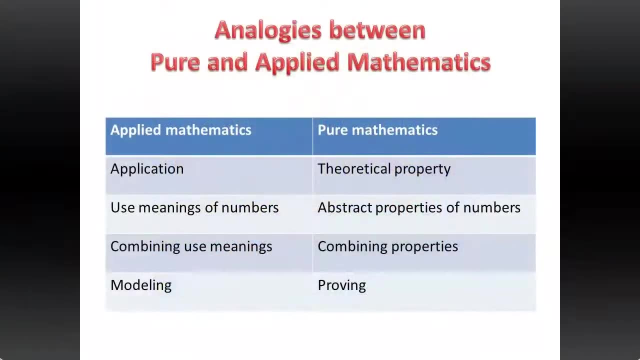 that we so often associate only with pure mathematics becomes critical in the understanding of geometric modeling. In fact, there are analogies between pure and applied mathematics. Applications are to applied mathematics as theoretical properties are to pure mathematics. More specifically, the use, meanings of number and operations are to applied mathematics. 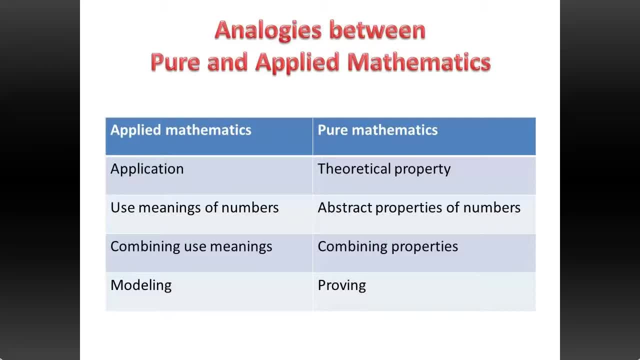 what the field properties of mathematical numbers are to pure mathematics. Combining rate and change to get the concept of rate of change is akin to combining postulates and definitions to obtain a theorem. The basic process by which we work with applications is mathematical modeling, The basic process by which we develop pure mathematics. 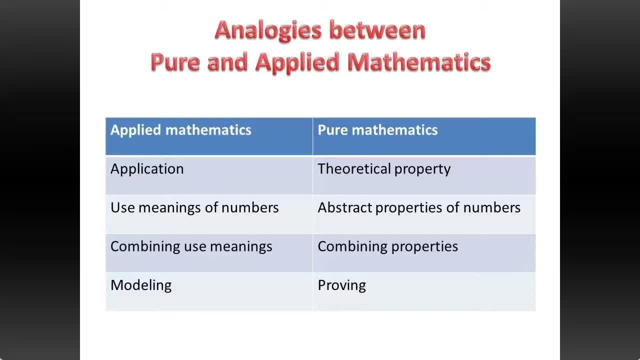 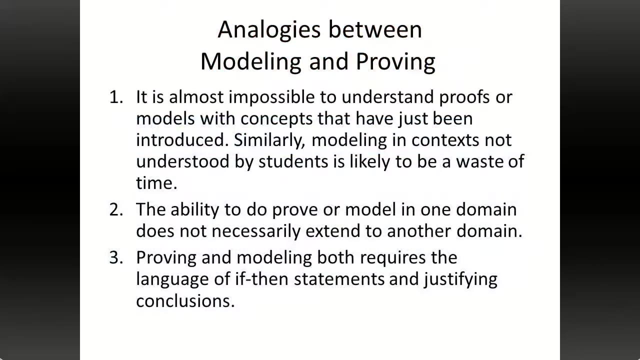 is that of proving, proving and modeling counterparts. We have been trying to teach students prove for quite a bit longer than we've been teaching modeling. what can we learn from that experience? Here's some thoughts. Students understand proofs with concepts that have just been introduced. For instance, the college student. 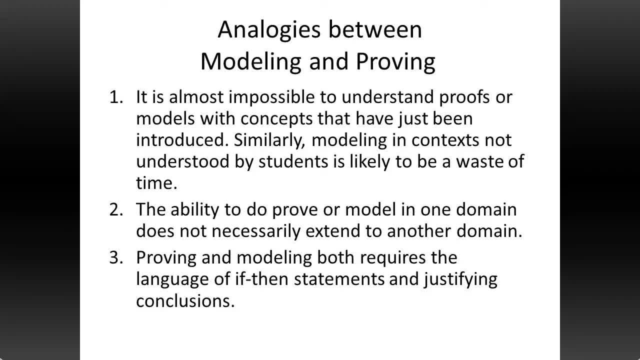 who's just introduced the concept of group in abstract algebra finds it difficult to write proofs about groups. The student in geometry finds it difficult to write proofs about quadrilaterals if they haven't studied quadrilaterals before. Similarly, modeling in contexts not understood by students. 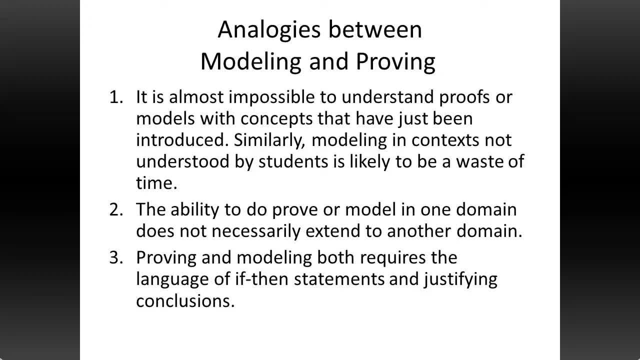 is likely to be a waste of time. Students have to have seen the context before. Second, the ability to do proofs in one domain doesn't necessarily extend proofs in another domain. Same is true for modeling. Third, proof learning requires the language of if-then statements. 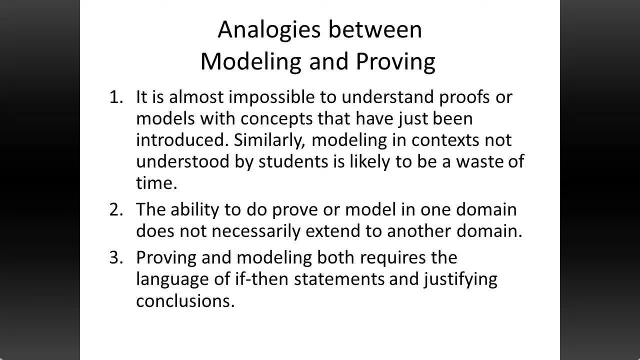 and justifying conclusions. Modeling requires the same logic. If these boundary conditions are assumed, if we have 40 golfers, what happens If we have 41 golfers? In fact, I think if-then statements are more natural in modeling than they are in proving. 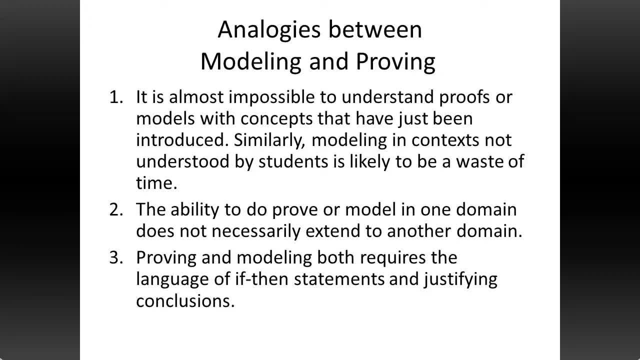 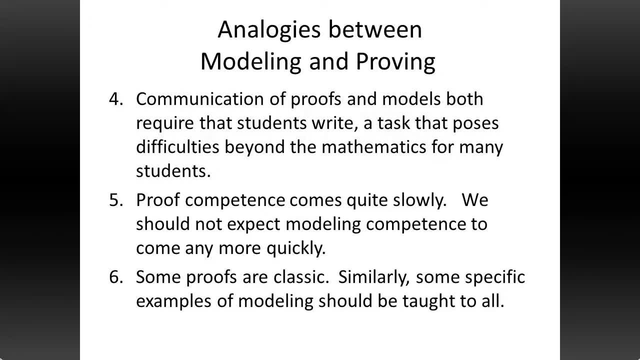 because we really have to make the statements in modeling. So I think we can use modeling to teach students about if-then statements. Communication of proofs and modeling both require that students write. This is a task in itself. Many students who can think really well do not have much writing ability. 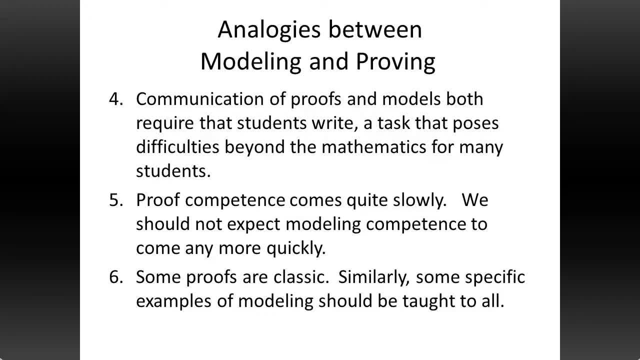 Writing is very important for both. Proof competence comes quite slowly. We shouldn't expect modeling competence to come any more quickly. That's why you need the learning progression. It needs to happen over multiple years, the same as with proof, And finally some proofs like the infinitude of primes. 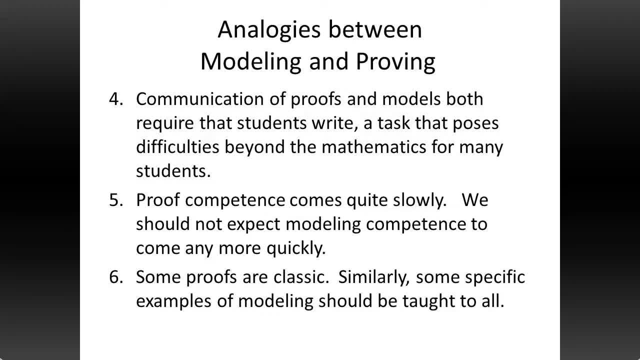 are classic. Similarly, some models should be treated with the same reverence and taught to all. One that would surely qualify is Kepler's modeling of Tycho Brahe's data about the orbits of the planets and coming up with what today are known as Kepler's three laws.